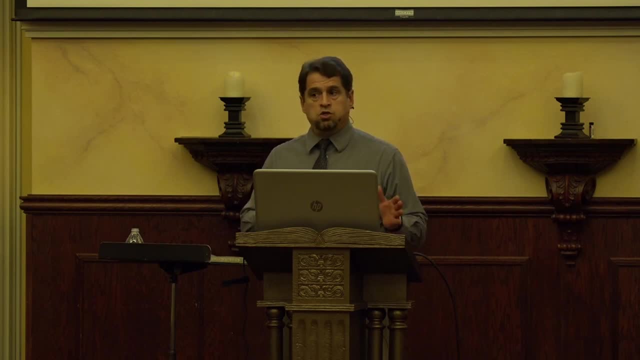 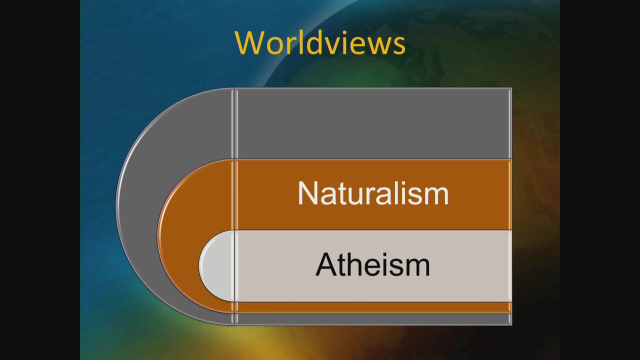 They've rejected the existence of God, rejected the Bible as being a source for truth and believe that all of this came about through purely natural processes. This atheistic worldview creates a philosophical position known as naturalism, And this is the position that is taken by science today. is the position of naturalism? They argue that all physical 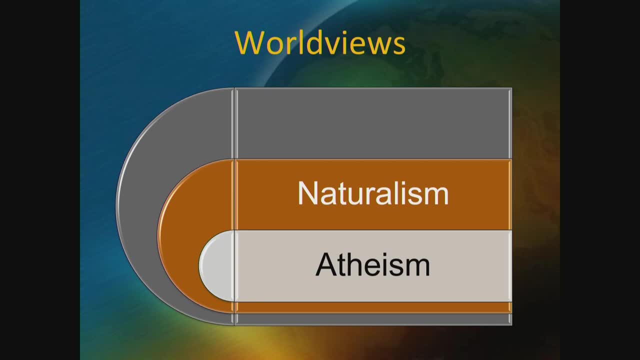 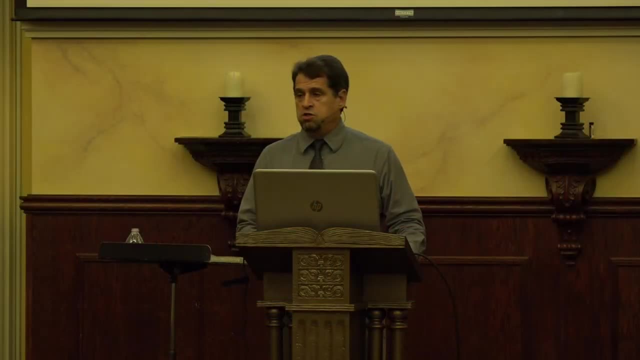 phenomena occurs through purely natural processes and the origin of everything we see has come into existence through purely natural processes. This is the position that the scientific community has taken And this is why our science museums today are called natural history museums. They're the history of the world from natural processes. They call them natural history. museums. That's why we call a synonym going back for more than a century, of a scientist is what they call a naturalist. for the same reason, The reason why we call the world out there nature is because it's believed to have come about through purely natural processes. This is the 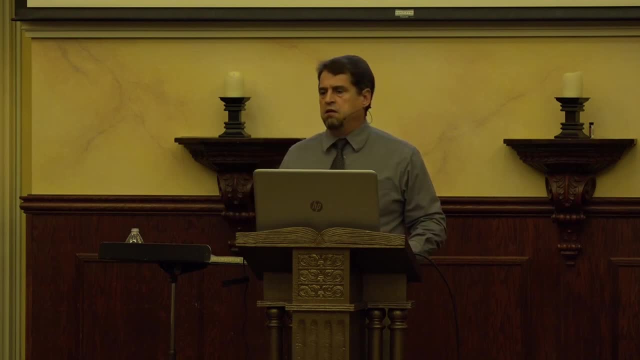 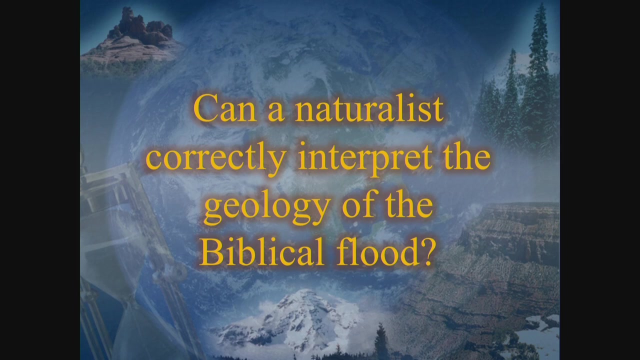 position that the scientific community has taken, But I argue that, for much of we want to ask ourselves. in general, though, is it possible to interpret a world with the supernatural history? through rigid naturalism, Scientists are trying to explain how our world came to be through purely. 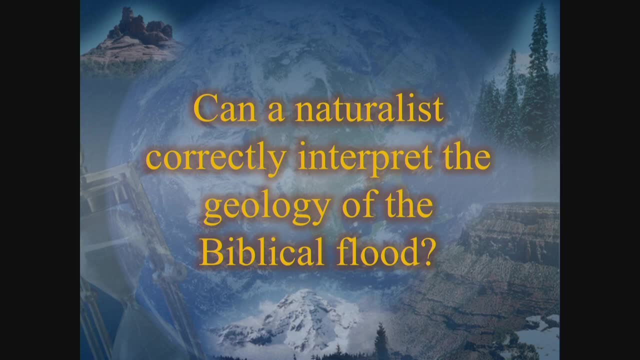 natural processes, but we know from the Bible that God spoke the universe into existence. I mean, how are you going to explain the origin of something that Almighty God spoke into existence? I mean, some aspects of the creation can never be understood within the boundaries of naturalism, and one of those particular events is the global flood. 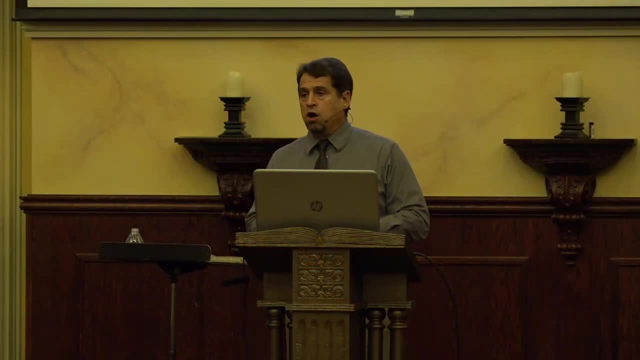 which is kind of the focus of our talk tonight. I argue that it's impossible to correctly interpret the geology of the biblical flood through rigid naturalism. I mean, you would think they could. Geologists know a lot about geologic processes, about how things erode. how about? 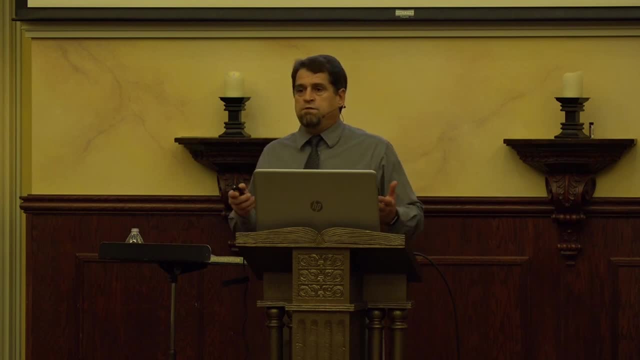 erosion and sediment deposition. We're going to talk a lot about this stuff. You'd figure they could, because they're really smart and they know a lot about geologic processes. but I argue that they can't, that it's impossible for naturalists to correctly interpret the geology of this event. 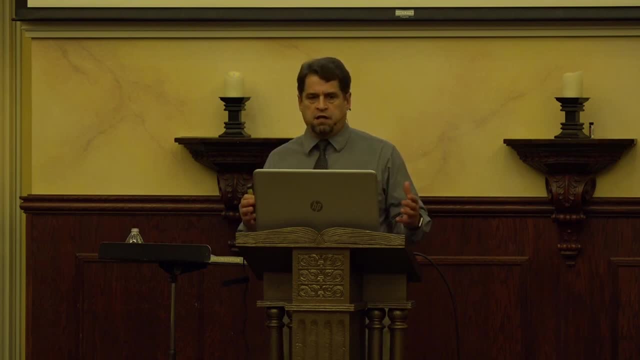 We've got to remember that this was a global-scale event. global-scale event. Genesis 6 through 9 records the details of the flood of Manoah, And the waters prevailed so mightily upon the earth that all the high mountains under the whole. 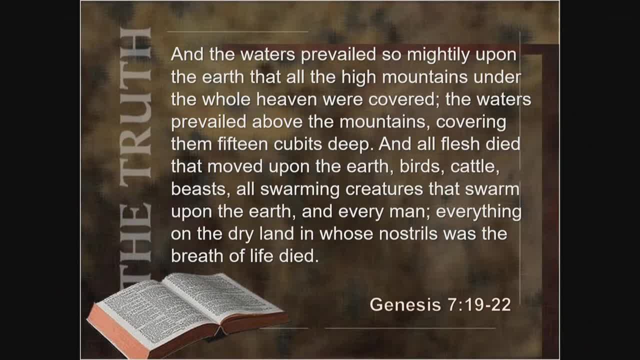 heaven were covered, The waters prevailed above the mountains, covering them fifteen cubits deep, and all flesh died that moved upon the earth: Birds, cattle, beasts, all swarming creatures that swarmed upon the earth, and every man, Everything on dry land and whose nostrils were. 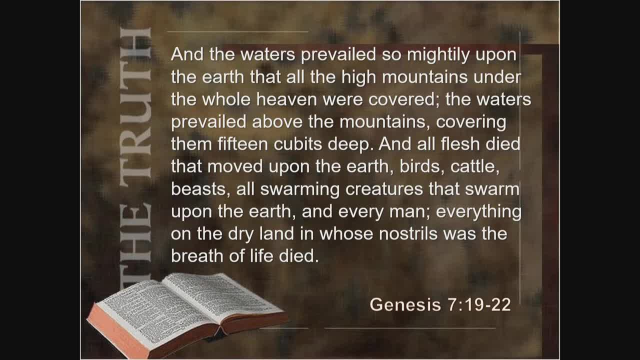 the breath of life died. This was a global-scale, all-encompassing event. All the high mountains were covered, Everything on dry land and whose nostrils were the breath of life died And every man. This was a terrible and global-scale event And I'd argue: you know what would we? 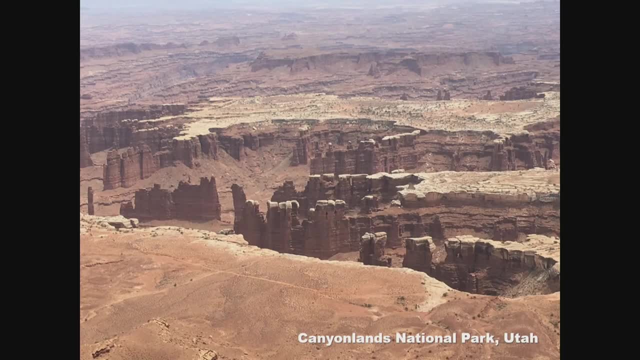 expect to see if an event like this was real and global in scale, other than what we see. We live on a flood wasteland. I mean, some of the best places to see this are in states where there's little vegetation. You go down through Utah and you know some of these areas where vegetation hasn't. 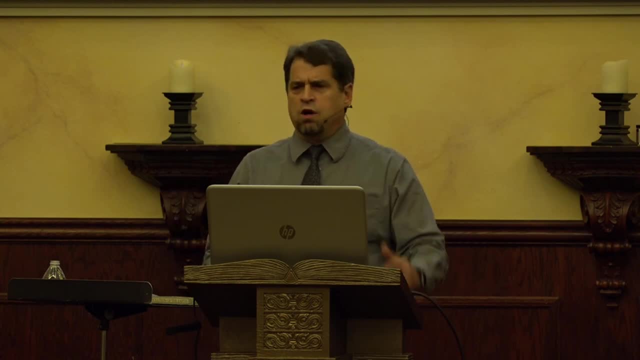 you know, doesn't completely cover the ground And I happened to watch a program the other night on PBS that was doing flybys over Utah and Arizona. some of these flood And that's what you see when you look at these areas from the 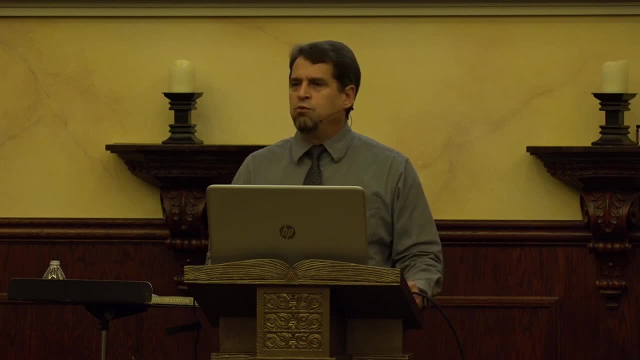 airplane. It's so obvious. It's what we live on. We live on a flood wasteland. That's what this world is And, again, you would think that a geologist could recognize it. If there had been a global flood as the one described in the Bible, you would think that a geologist would be able to. 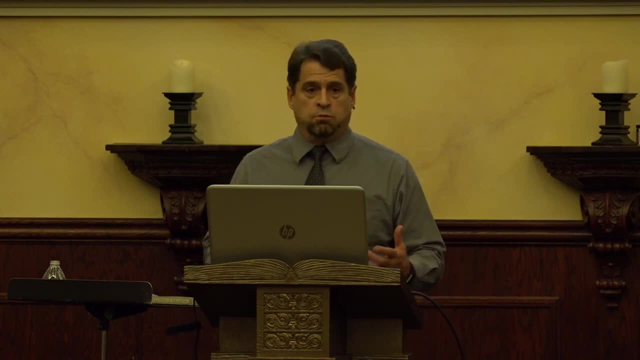 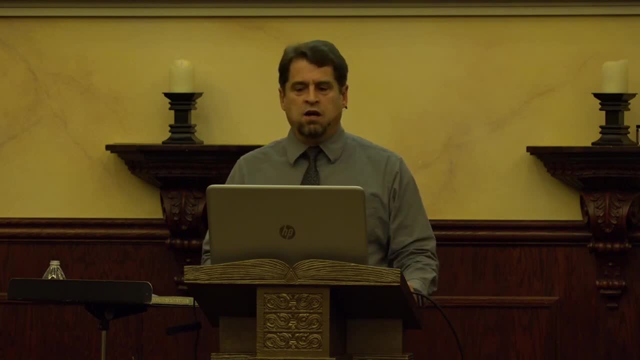 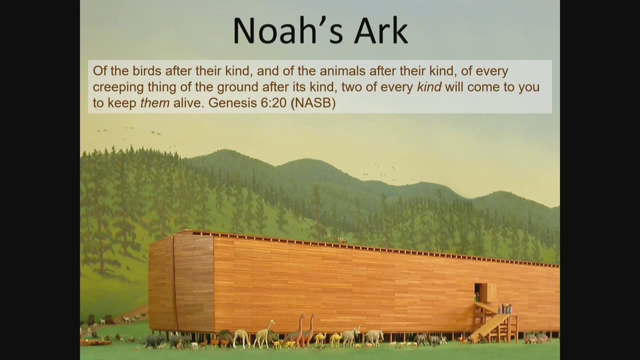 that was involved in this event And it's this piece right here. God told Noah there was going to be a flood, told him how to make an ark that would allow him to survive this event, along with all the animals that came to Noah. It specifically says: the animals will come to you. 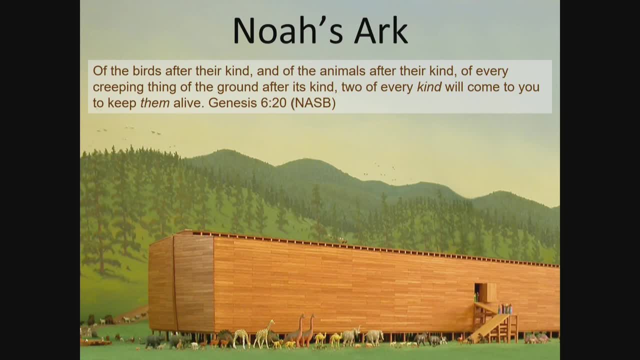 to be kept alive. The only reason life exists today on top of these vast layers of flood deposits that cover the entire world is because they were saved from this event through an act of supernatural intervention. This supernatural connection with this event precludes or prevents a naturalist from correctly interpreting the event. We live in a world that's covered in. 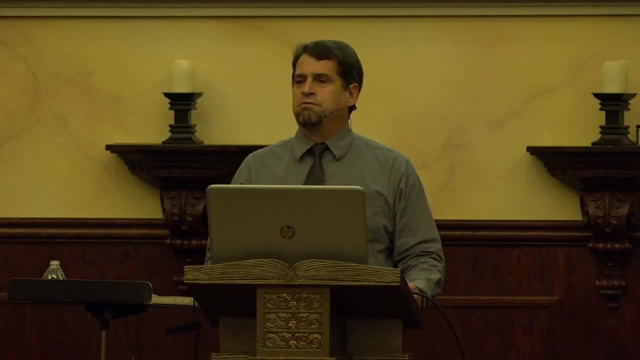 monumental layers of flood deposit, But life exists on top of those vast layers of rocks. How is a geologist rigidly bound in naturalism going to make sense of that? It's impossible. How can they make sense of a world as it now exists? It's impossible. So be skeptical about their interpretations of. 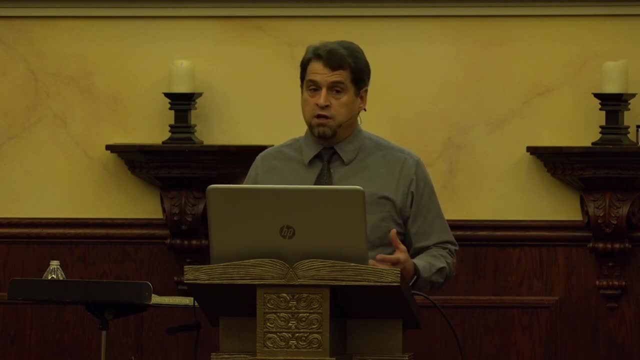 geology, I would argue. if there has been a global flood as the one described in the Bible, then one thing is certain: The geology of that event has been misinterpreted Big time. When this philosophical view of naturalism is applied to geology, as it has been this birthed, 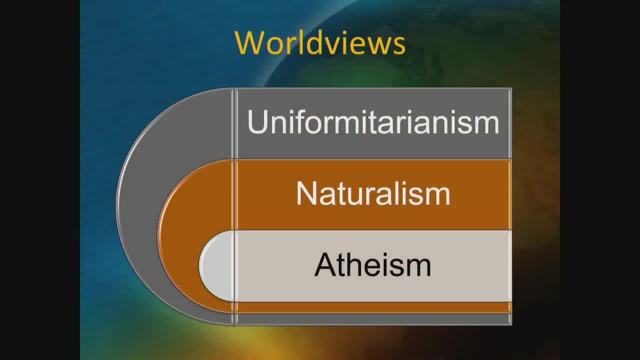 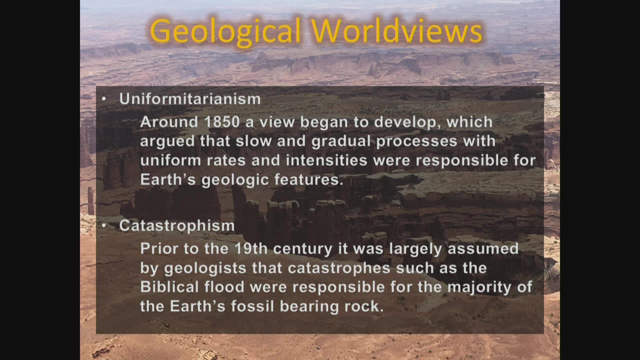 what we call uniformitarianism. Around 1850, this view called uniformitarianism finally really started to take shape, which argued that slow and gradual processes with uniform rates and intensities were responsible for Earth's geologic features like fossiliferous rock and erosion. This view became known as 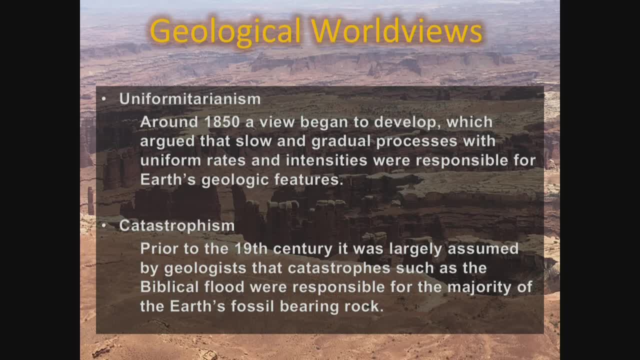 uniformitarianism. However, prior to the 19th century, it was largely assumed by geologists that catastrophes, most importantly the biblical world, were not a problem. The biblical world was responsible for the majority of these features. The concept of uniformitarianism was ushered in by 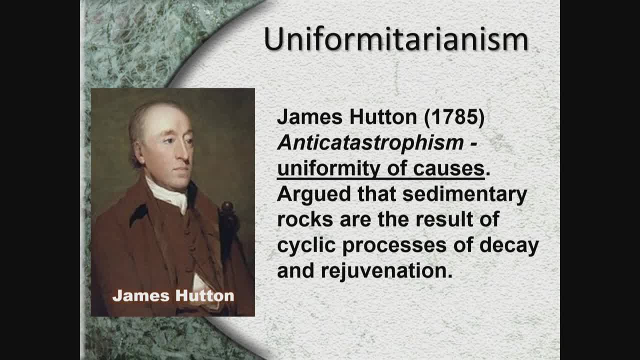 two champions of geology, one of them shown here, James Hutton, and another by the name of Charles Lyell. I will introduce you to in just a second. James Hutton was an anti-catastrophist. Prior to ushering in this view, the vast majority of peoples assumed there had been a global flood. 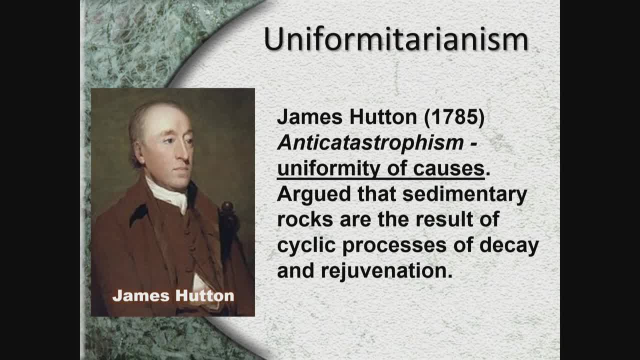 at least peoples that lived in areas with access to the Bible assumed that the layers of rocks that they saw, that the fossils they found, were those that were formed by the global flood. So he was an anti-catastrophist who argued in his 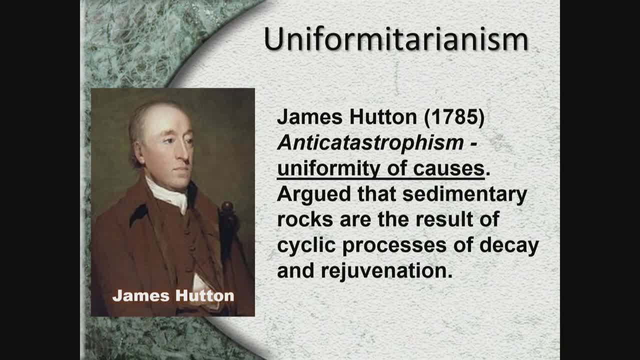 1875 book titled The Theory of the Earth for Uniformity of Causes, to Explain the Earth's Geologic Features, He asserted that sedimentary rocks are the result of cyclic processes of erosion and sediment deposition, processes that, he argued, do not change over time. He summarized this: 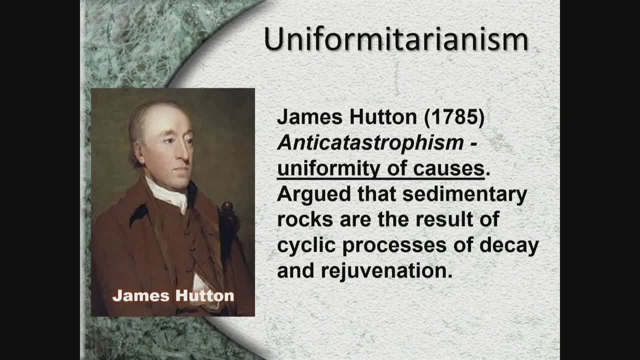 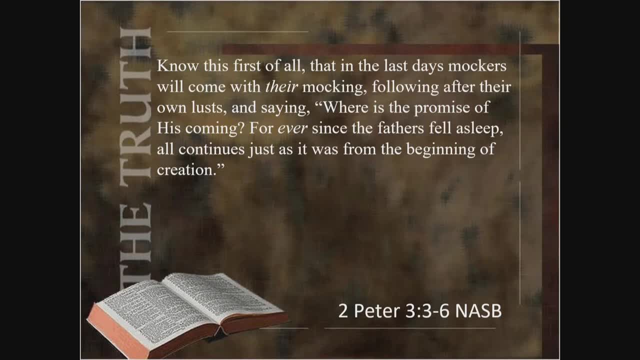 with his famous phrase: no vestige of a beginning, no prospect of an end. With this in mind, listen to this prophecy from 1 Peter 3,, 3-6 in total. Know this first of all, that in the last 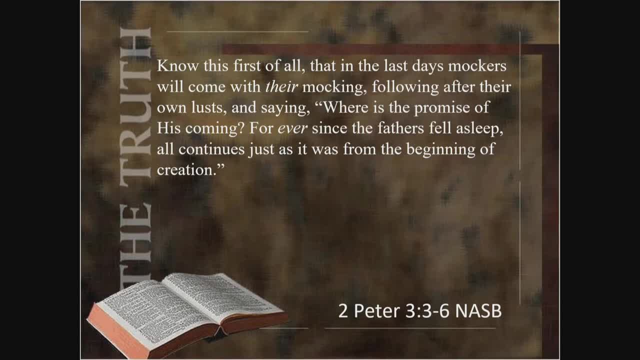 days, mockers will come with their mocking, following after their own lust and saying: where is the promise of his coming? For ever since the fathers fell asleep, all continues just as it was from the beginning of creation. This is exactly what you see in this prophecy. It's not just a 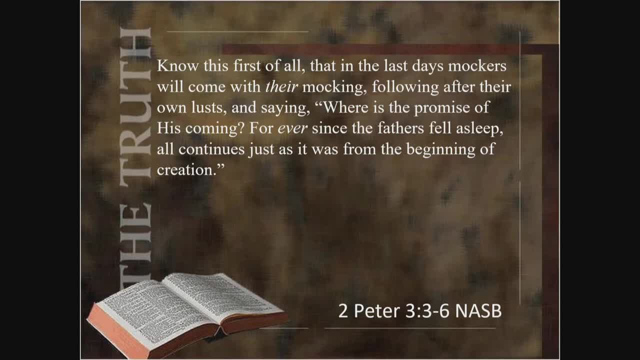 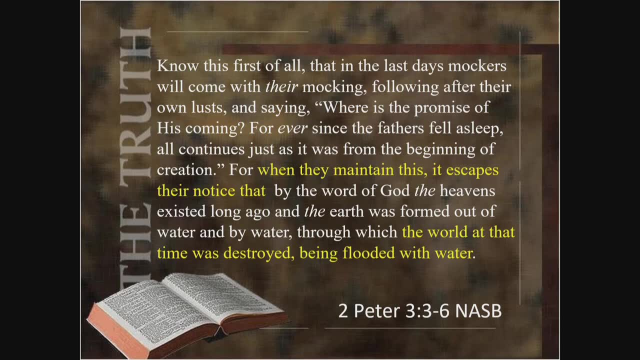 uniformitarian geology argues that geologic processes have not changed over time. All things continued as it was from the beginning. Now let's read on, For when they maintain this, it escapes their notice that by the word of God, the heavens existed long ago and the earth was formed out of. 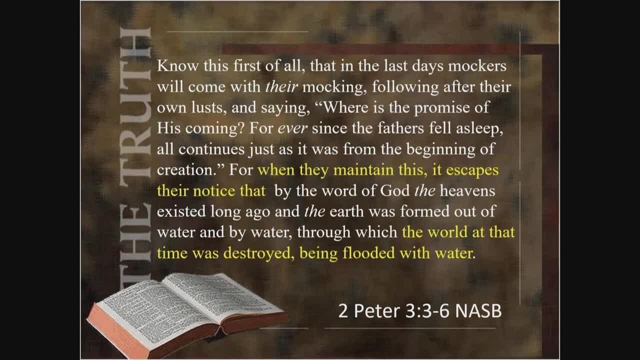 water and by water through which the world at that time was deluged, being flooded with water. This is the world that we live in. This prophecy is coming to fruition as we speak. This is what geologists hold to, that all things continue as they were from the beginning. Cyclic processes. 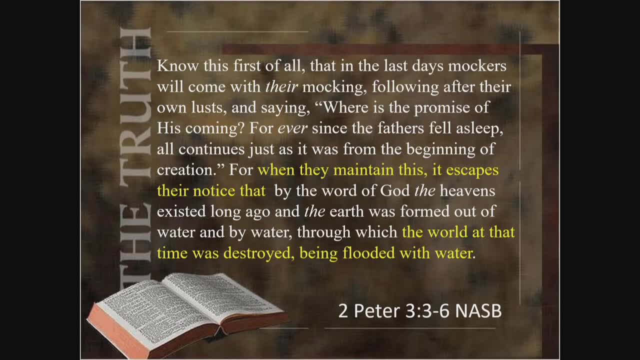 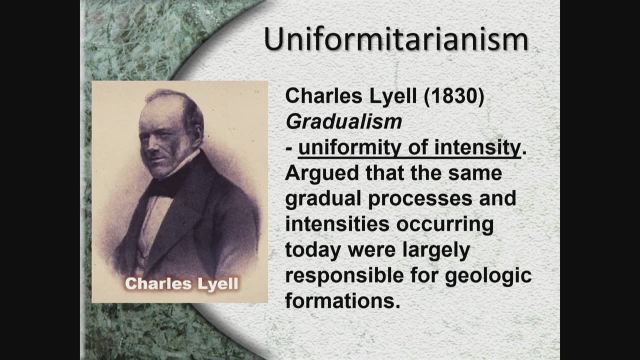 of sediment. deposition, uplift and erosion have been continuous throughout the history of life on earth and are responsible for the vast layers of rocks that we see. In 1830, Charles Lyell argued in his book titled Principles of Geology for uniformity of intensity. He asserted that the 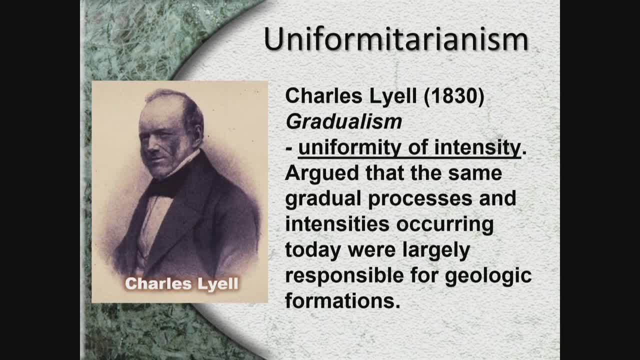 same gradual processes occurring today were responsible for all geologic features. He, his famous quote was that the present is the key to the past. He argued that the same processes we see happening today are responsible for all geologic features. Charles Lyell influenced. 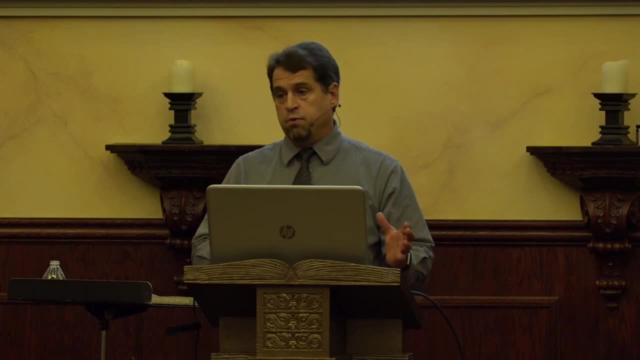 Charles Darwin heavily. They were contemporaries living at the same time communicated regularly. It was said that Charles Darwin had a copy of Lyell's book with him when he took his famous voyage out to the Galapagos Islands. It was said that Charles Lyell actually met him when he returned. They were close friends and 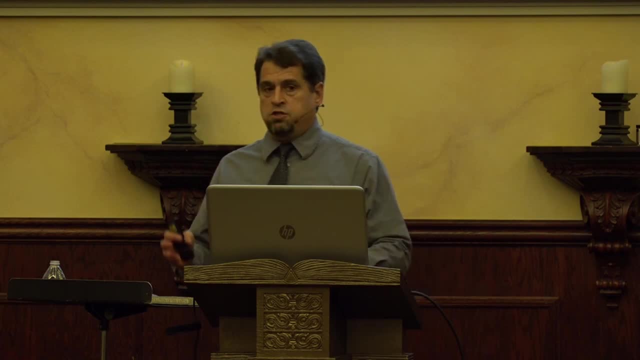 were in constant communication. Charles Darwin's views about the age of the earth were largely due to the teachings of Charles Lyell. These two views- catastrophic versus uniformitarianism- can be debated anytime we look at geologic features like those that you see here in. 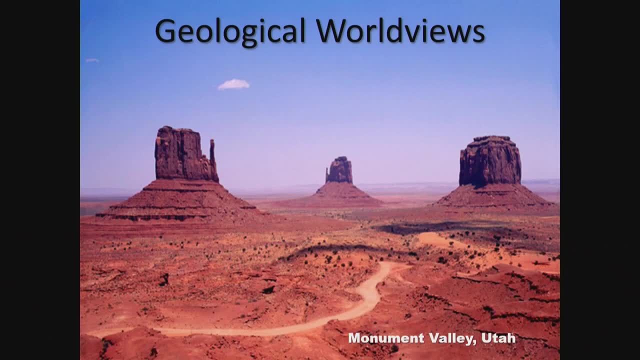 Monument Valley, Utah. All of the rock that you see here is sandstone, a type of a sedimentary rock. We'll talk a little bit about that in a minute, But it's a type of rock that is a new rock. The sand that's in this area was transported to this area. Particles weathered. 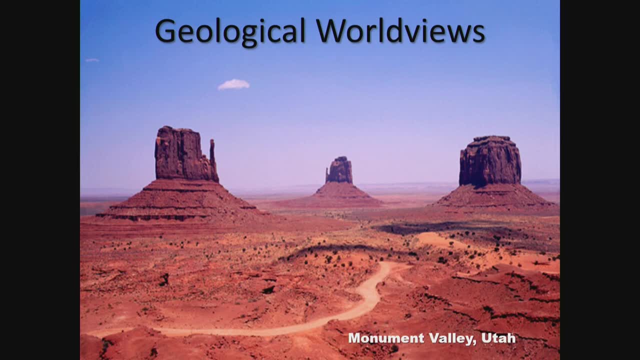 other ancient basement rocks weathered away into smaller particles. Those particles were transported by the actions of fluids and deposited in this location. Originally they were deposited as high as the monuments are today forming a vast floodplain of sedimentary deposits, So something transported these sediments there. 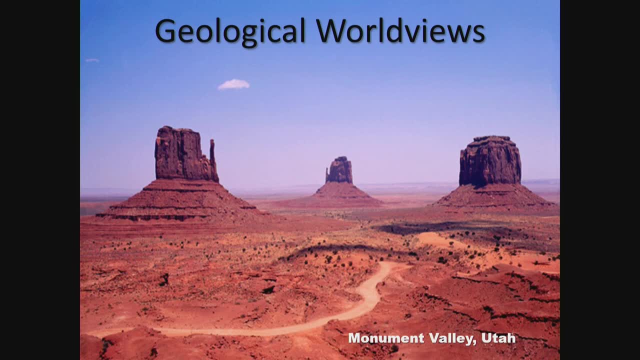 And deposited them there, forming a vast floodplain, And then something eroded away all the material that's now missing. So whether this was through uniform rates of erosion and deposition or whether this was catastrophically done, is the debate A little bit hard to explain? where all the missing? 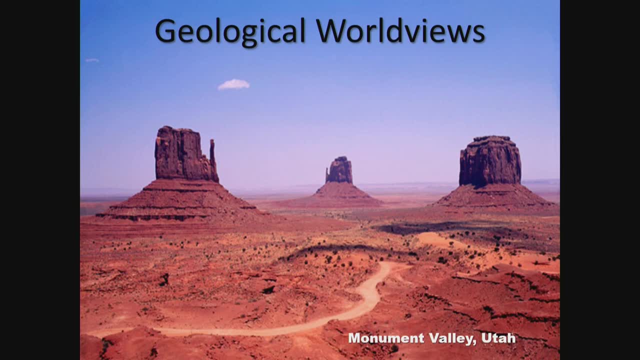 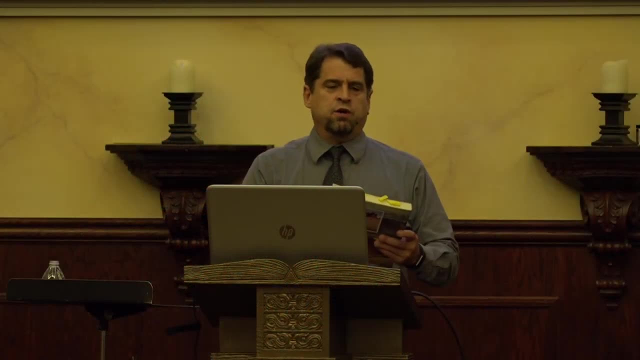 sand is without some kind of a catastrophic sweep away. Let me take a diverge for just a moment, because I want to read you something out of a book that I was assigned when I took a geology in college. When I was at Texas Tech, we were assigned this book. 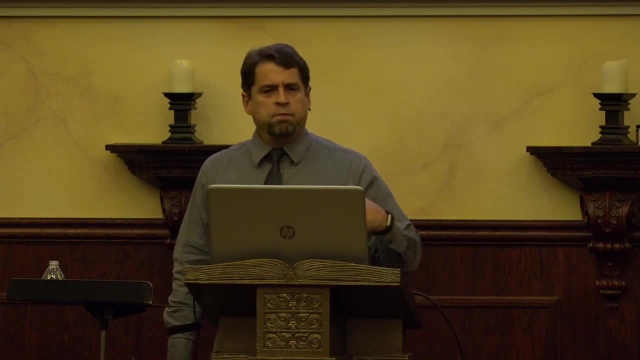 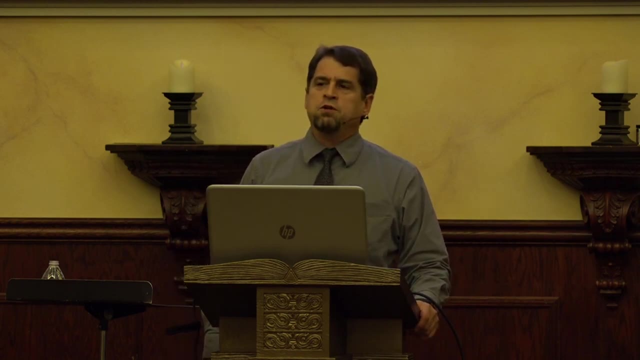 Taking Geology, And I mean I grew up in the church and have always known about the global flood. Growing up, from growing up as a kid, I always knew about the global flood, And growing up in New Mexico, I interpreted the geology that I saw as having come about through the flood of. 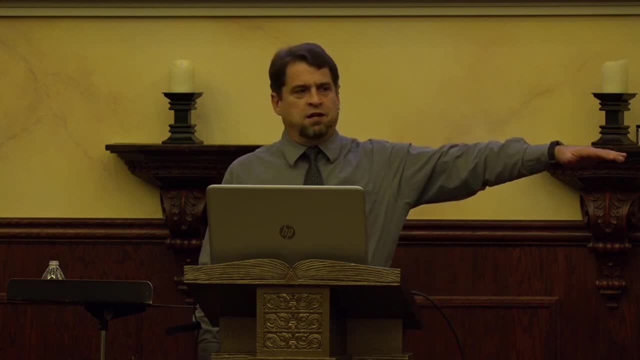 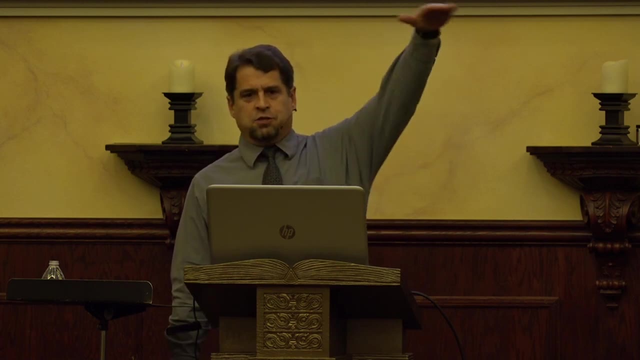 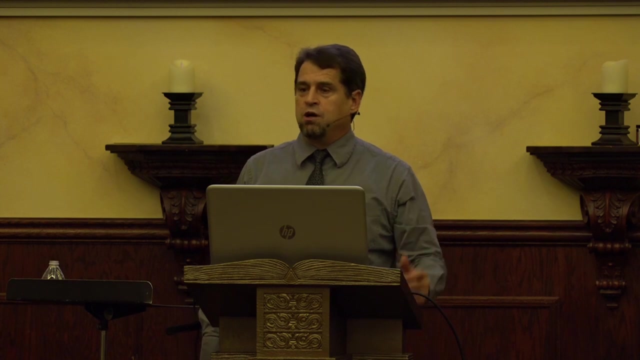 Noah, In New Mexico you have vast salt flats and the cliff faces that you see had rings on them that to me they look like recession rings. Oh look, that's where the water receded. And right outside Roswell, where I grew up, there were saltwater lakes. There's a series of saltwater. 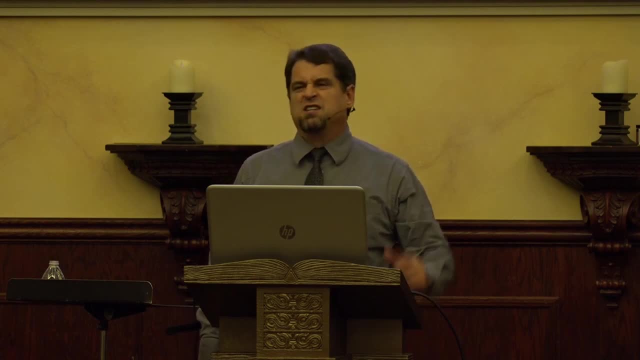 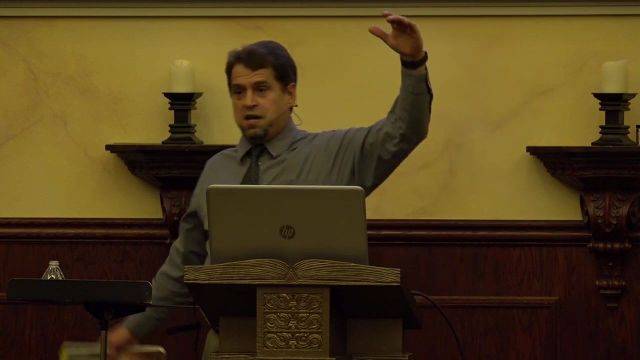 lakes, called Bottomless Lake State Park. And then you got enormous caverns in New Mexico and a huge deposit of pure white sand called the White Sands National Monument, A 200 square mile deposit of pure white gypsum- Literally dunes. 50 feet high, just out in the middle of nowhere. Big 200 square. 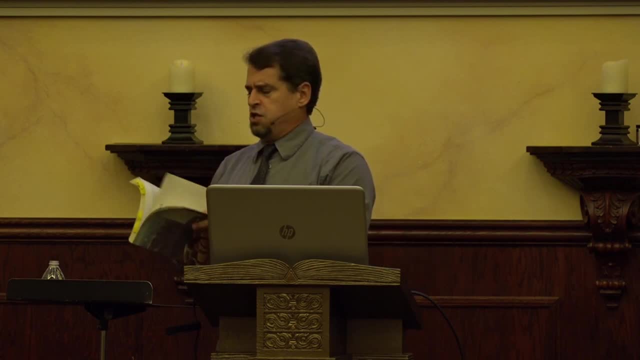 mile deposit of pure white gypsum. Anyway, there was some interesting geology in New Mexico And I always interpreted this as when I saw it, I interpreted it based on my understanding that there had been a global flood. But that's what scientists do. This is what's everyone interprets. 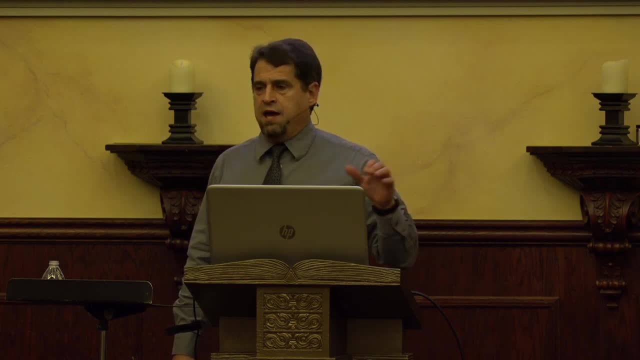 the world around them from their worldview, And informed as we are by the historical event of the global flood, we can make sense of the geology that's around us And scientists that have rejected the biology of the global flood. we can make sense of the geology that's around us And scientists that have rejected the 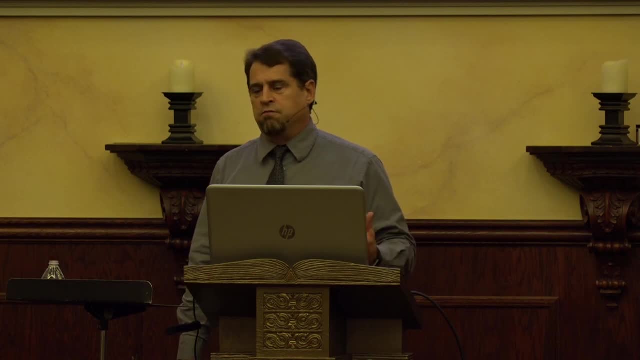 Bible and don't believe in creation. we can't really fault them for interpreting it differently. I mean, they're trying to make sense of the world. Everyone has to make sense of the world. You'd go crazy if you could not. But in my opinion you can't get to the truth without the Bible, And particularly 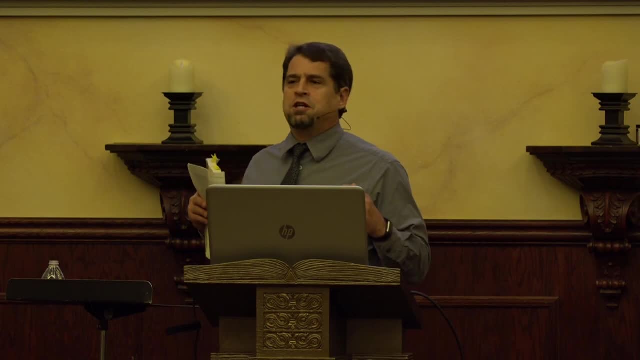 with regard to geology. Nonetheless, I took this class assuming I knew about the global flood, and I knew that they weren't going to be teaching us about the global flood, But I assumed that I was going to be hearing a lot of evidence for it in this class, which I did. Now let me point. 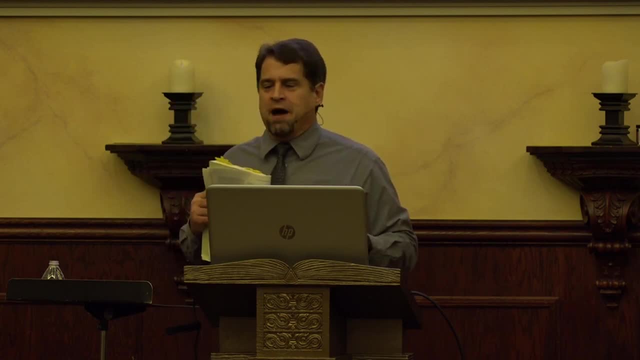 out lots of catastrophic related geology that I didn't know about from this class. But one of the things that kind of surprised me was all the references to the biblical flood. There's tons of references to the biblical flood. The book they assigned us starts off with an attack on 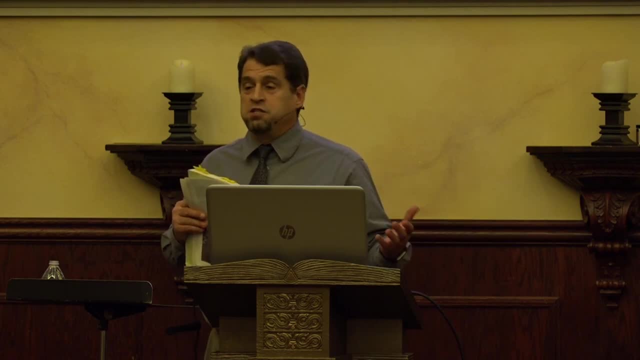 catastrophism on the original interpretation of geology, because they've been fighting against it ever since. And every all these- I don't know if you can see all those yellow tabs- all those yellow tabs in the first two or three chapters were references to the biblical flood, And one. 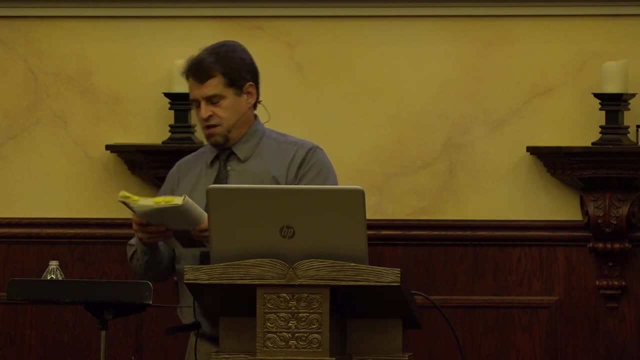 form or another. in this book you made an upcoming upfront attack on the biblical flood. Nonetheless, catastrophism versus uniformitarianism, They say. ancient peoples were quite understandably, or were, impressed only by rapid and violent geological processes. This led to a catastrophic view of the earth, commonly called catastrophism, which dominated European thought until 1850.. Changes were thought to occur suddenly, rapidly and devastatingly by a series of changes. The most famous example of such a supposed catastrophe was, of course, the great deluge of 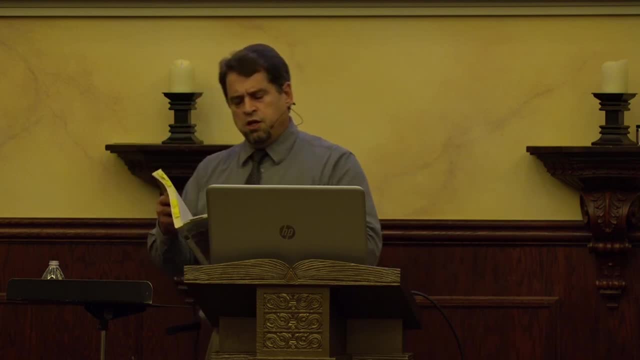 the Old Testament. When geology emerged as a vigorous intellectual pursuit around 1800,, an alternative concept of earth change began to develop. It was now argued that the same common processes observed operating today were largely responsible for all past changes imprinted in the 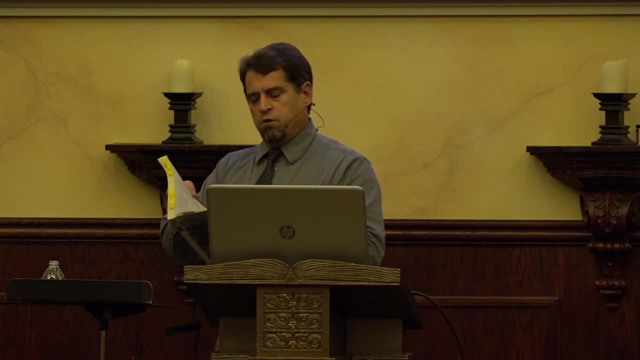 rock record. A non-catastrophic or more uniform view of geological processes was the first to change, thus emerge, which provided no role for unknown miraculous or supernatural processes. No role for miraculous or supernatural processes. Unfortunately, you cannot interpret the geology. 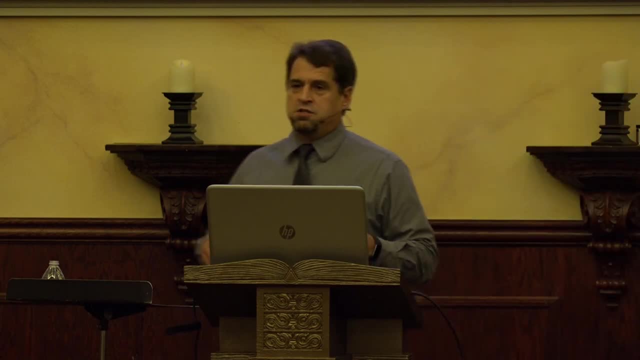 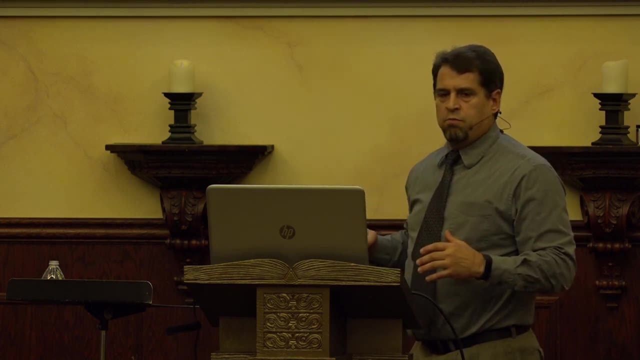 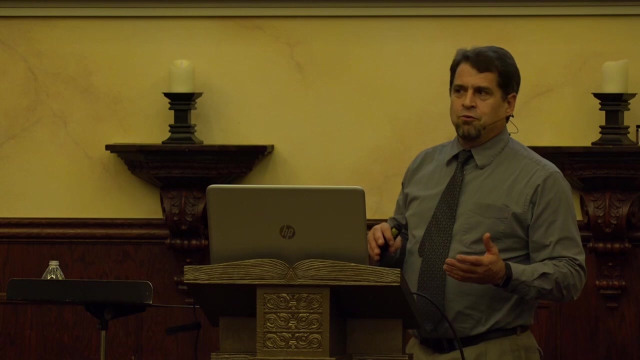 correctly without it. Because, again, what a geologist is doing? they're not just trying to interpret the world as we now see it, covered in these vast, monumental bodies of sedimentary rock, but you have to explain how that sedimentary rock got there, with life that still exists today, Because running around 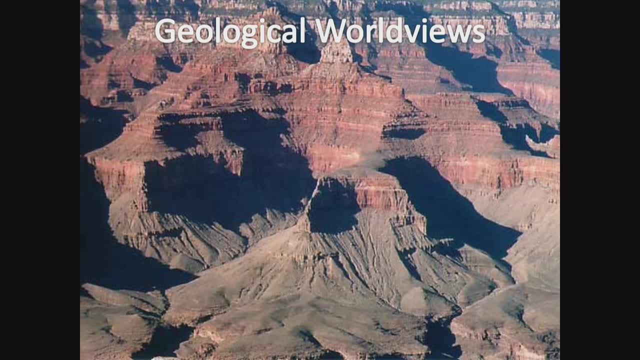 on top of those vast layers of rocks are lots of little fragile creatures. You've got cold-blooded animals that can't survive changes in temperatures, amphibians that can't survive exposure to salt waters, lots of little butterflies and things. Fragile organisms are alive today that could. 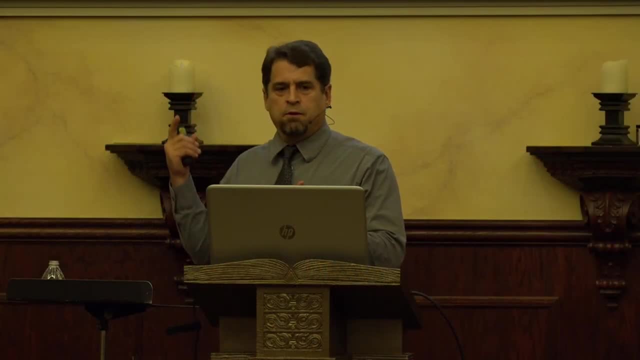 simply not survive an event capable of laying down such monumental deposits. But there they are. It creates an inexplicable situation for naturalists. They cannot interpret the world as it now exists, Because life only exists due to this act of supernatural intervention. How else can they explain it? Oh, those layers were due to some massive, catastrophic flood, but 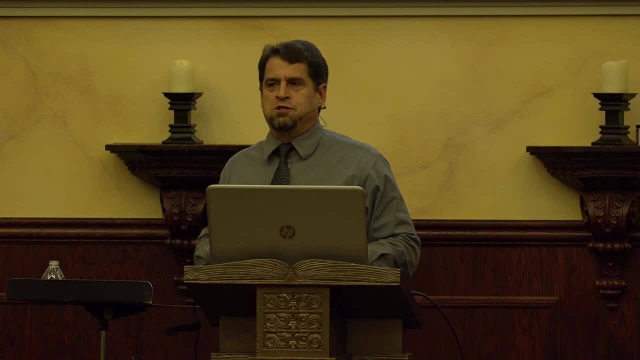 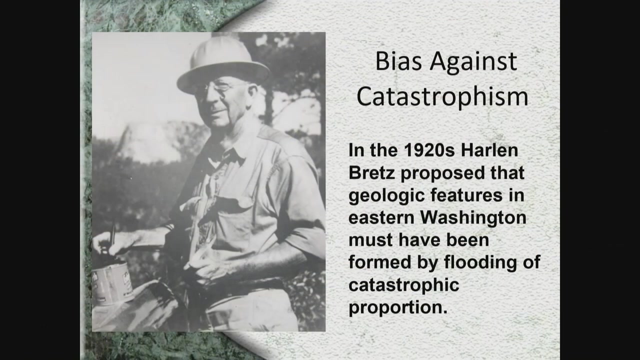 and that covers those sediments, cover the entire planet, but life, somehow, life miraculously, is still here. It's crazy. Well, because of this, geologists have been highly biased against catastrophism, highly biased against catastrophism, And this is best illustrated by the story of Harlan Bretts. Harlan Bretts was a 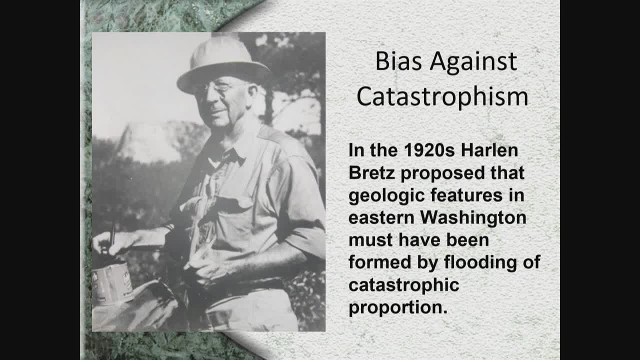 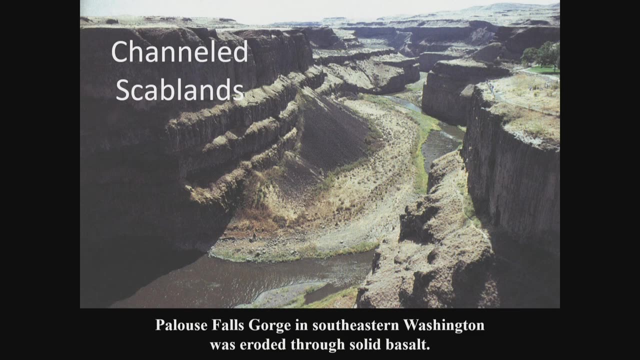 geologist here in Washington state And in the 1920s he proposed that Eastern Washington had been destroyed by a major catastrophic flood And he named this area of Eastern Washington the channeled scab lands, Because out in Eastern Washington you find these massive channels cut. 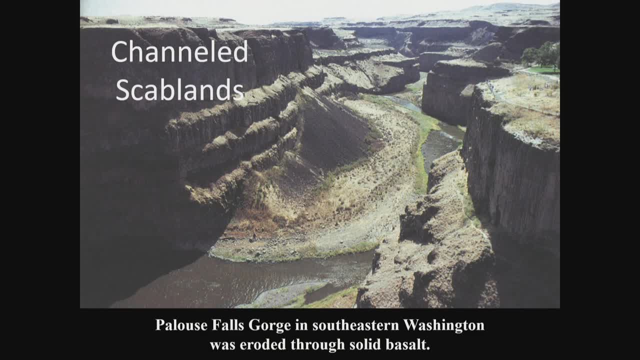 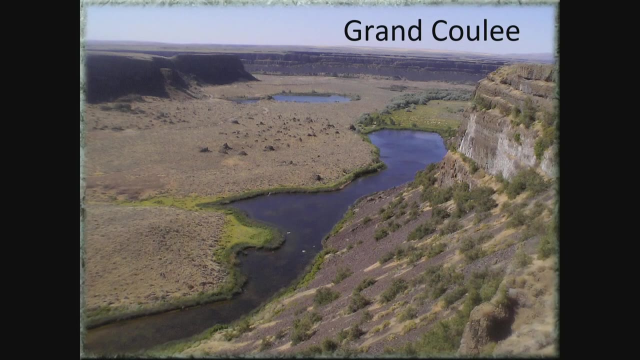 down, cut deeply into the ground through hard volcanic rock. This entire area is covered in massive layers of volcanic rock. The walls of this canyon are solid volcanic rock, But these canyons are gorgeous, have been cut into this And some of them vast in size, Massive geologic. 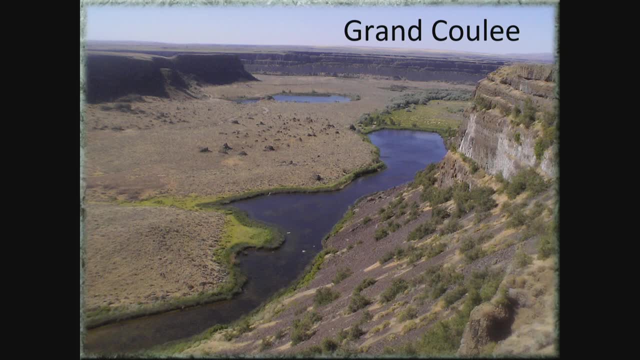 features like the one you see here. this is called a coulee. The Grand Coulee reaches, at its maximum, four miles wide and 900 feet deep. Now, this was one of Harlan Bretts' most important examples. He argued that these coulees could not have been formed unless they were full of water. 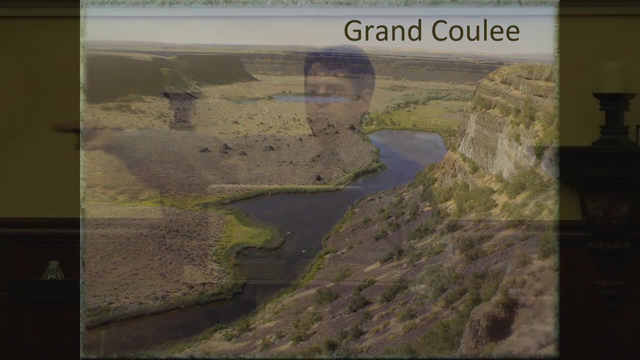 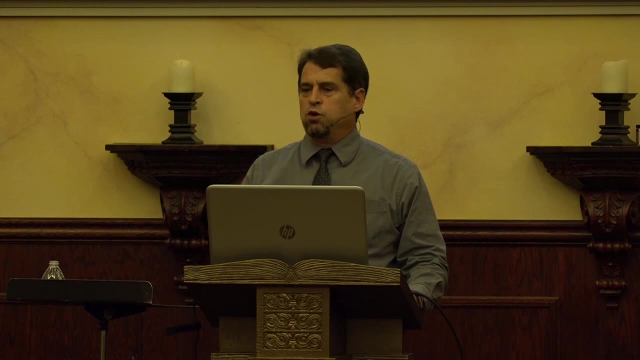 at one point in time, Because the bottoms are really super flat And the walls are very straight. He argued the only way a formation like this could form is if it was full of water at one point in time. That it was completely full of water at one point in time, But again this thing is at its 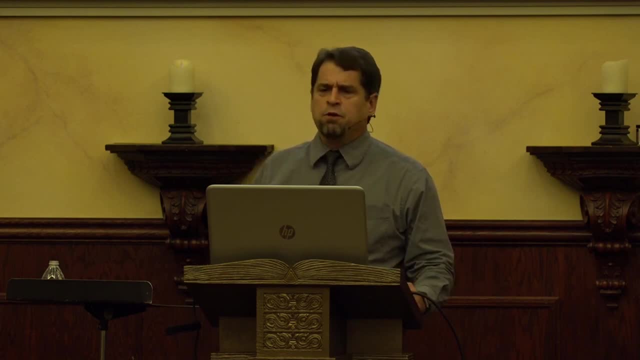 widest, four miles wide, 900 feet deep. The entire thing completely full of water, at one point in time Inconceivable. This is a region that sees very little of water. This is a region that sees very little rainfall today, But Harlan Bretts argued it was all of these features were the 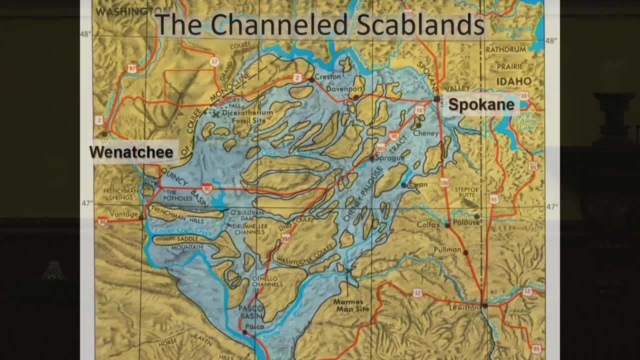 result of a catastrophic flood. This map gives you a good indication of how much water would have been necessary. You see the span of the land that's involved here between Wenatchee and Spokane. Everything in blue there was what would have been underwater at one point in time during. 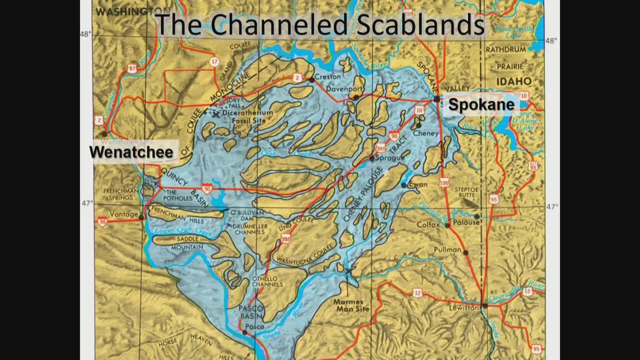 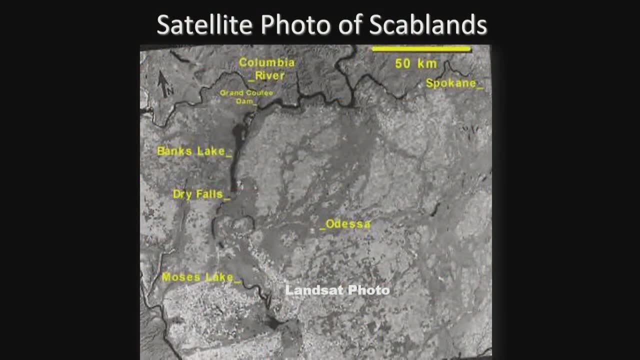 this flood. The darker blues, if you can make those out, are where water is today. You can even see these, these channels, these gorges and canyons from satellite photos. This is a satellite photo. You can see the dark lines cut into it. This is where the channels are today. Well, Harlan Bretts for the. 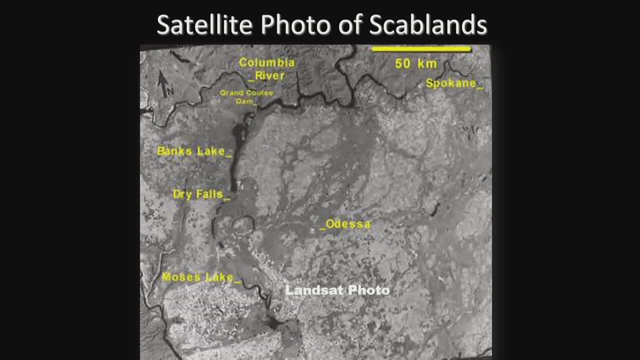 proposal, found himself ostracized by the scientific community. Ostracized Because they've been fighting against catastrophism since the mid-1800s And here comes this guy in the 1920s talking about catastrophic floods. That sounds a little bit too close to biblical kind of stuff Can't talk about. 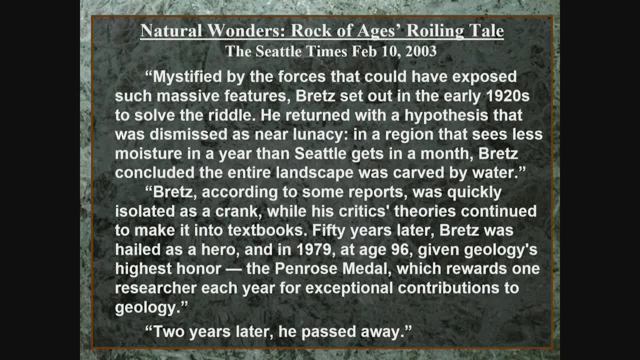 it Can't explain geology today. This is an article from the Seattle Times 2003.. Mystified by the forces that could have exposed such massive features, Bretts sat down in the early 1920s to solve the riddle. He returned with a hypothesis that was dismissed as near lunacy. 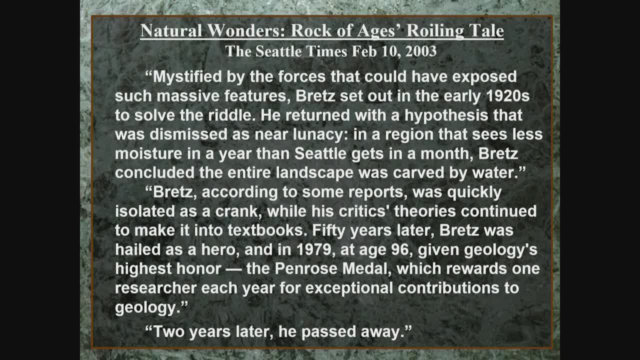 craziness. In a region that sees less moisture in a year than Seattle gets in a month, Bretts concluded that the entire landscape was carved by water. Bretts, according to some reports, was quickly isolated as a crank, A crazy person, While his critics' theories continue to make it into textbooks. 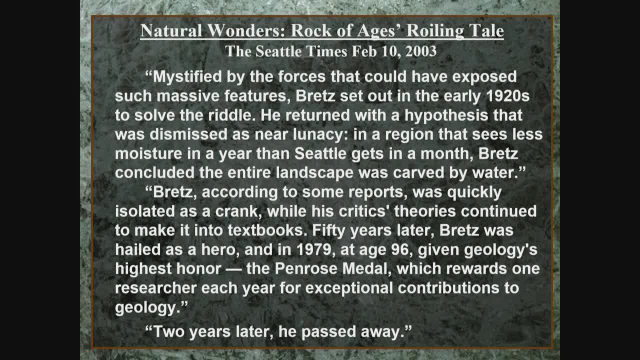 50 years later, Bretts was hailed as a hero And in 1979, at the age of 96,, he was given geology's highest honor, the Penrose Medal, which rewards one researcher each year for exceptional contributions to geology. Two years later he passed away. He was ostracized by the geological community for 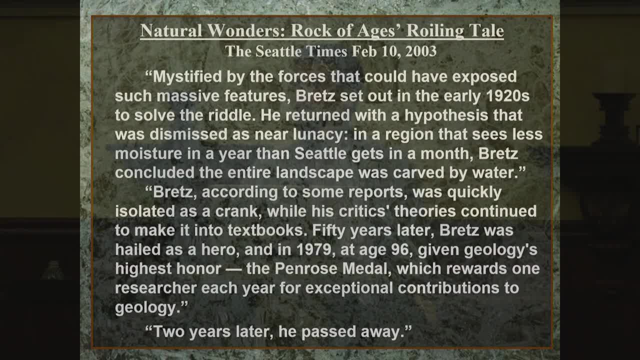 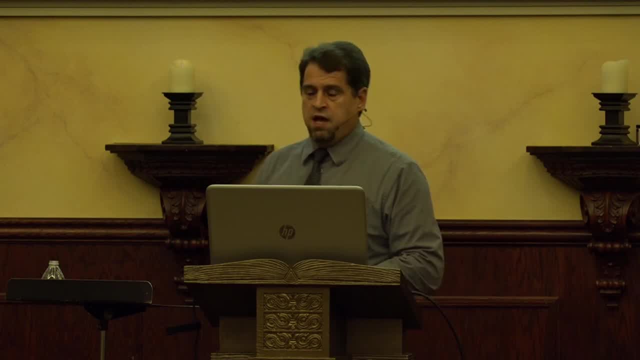 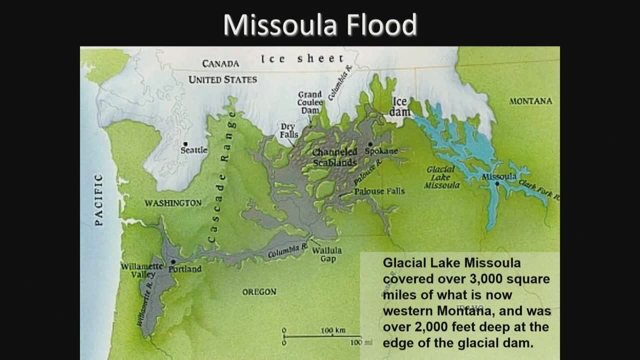 50 years And finally hailed as a hero Two years before he passed away. We now know, because obviously he was eventually recognized for this, that eastern Washington was destroyed by a major, catastrophic flood. It is today called the Missoula Flood, And this map gives you a pretty good idea of what happened. 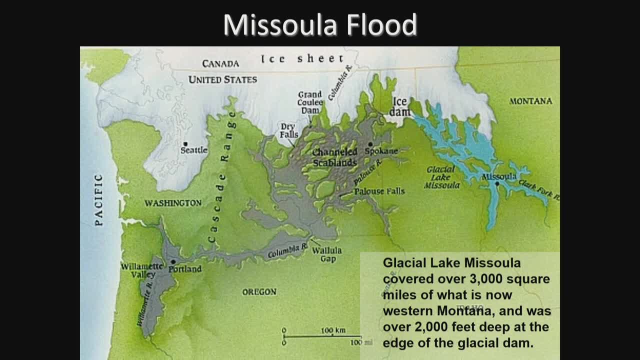 The floodwaters are believed to have come from a large ice age lake that is centered around what is today Missoula Montana, Thus its name, But the lake itself was building high-altitude, higher and higher due to the melting of glacial waters, and was unable to run off. 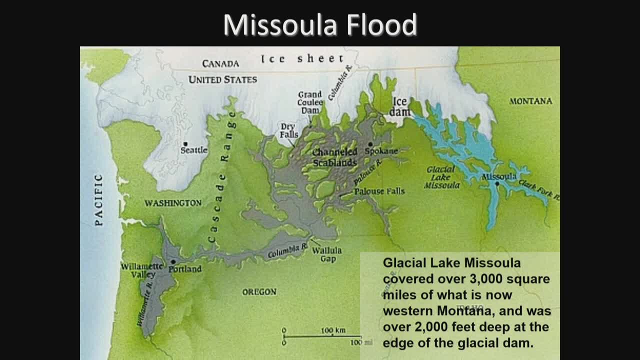 There wasn't either. They argue that an ice dam was keeping it in place. We believe that the ice age was caused by the global flood, And after the global flood there were no drainage systems. yet The continents would have been vast floodplains without significant 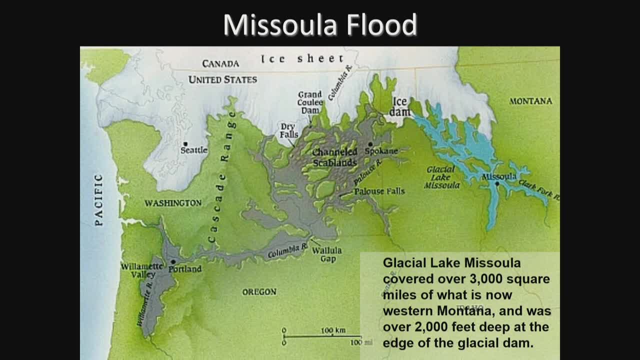 drainage systems, And it's just possible this lake did not have a drainage system, an outlet for it to the ocean, yet, But it is said that it was held in place by the people of Missoula By an ice dam And at some point that ice dam breached and the entire body of water contained. 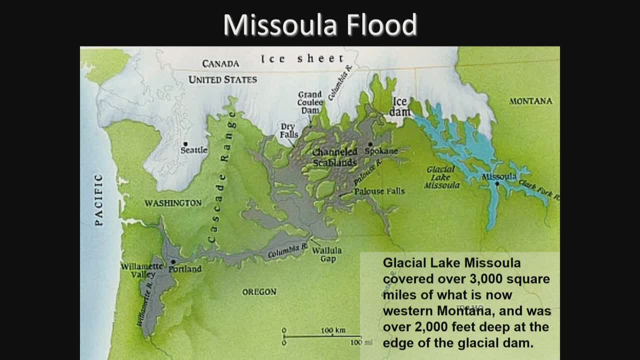 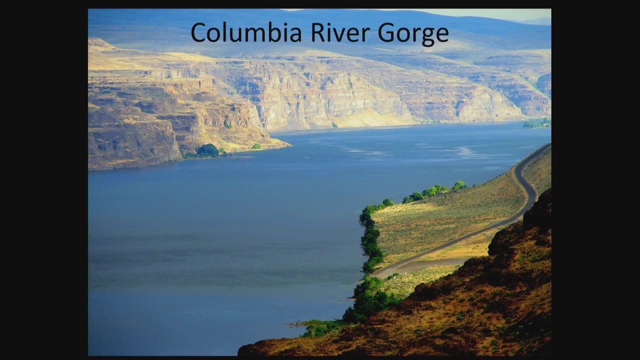 within the Missoula Flood. 3,000 square miles, 2,000 feet deep lake plowed its way across eastern Washington. in a couple of days It carved out the Columbia River Gorge. If you've ever been stopped in one overlook of the Columbia River Gorge, you know the mass, the size that you're talking about. 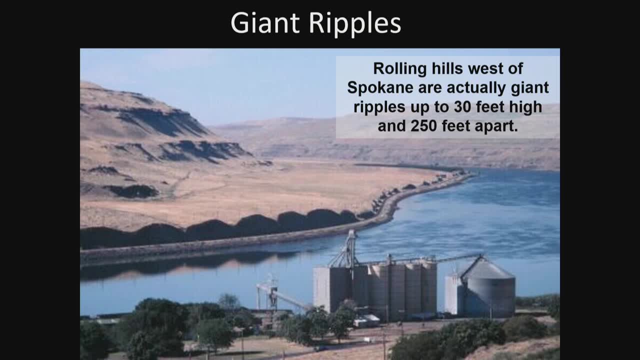 here And it formed features That only from the airplane were recognizable as flood. features Like the rolling hills that you see here outside of Spokane are 30 feet high, 250 feet apart from the ground They're just hills, But from the airplane asymmetry became apparent And they finally recognized And in fact, 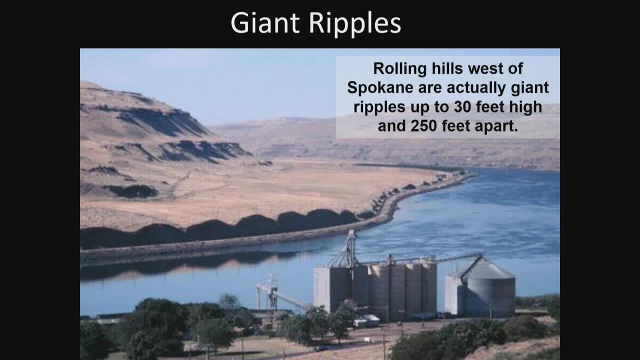 much of the area was. They only finally came around and acknowledged Hardin-Bretts after viewing the area from the airplane sufficiently. The rolling hills around Spokane they then recognized to be ripple marks. They were features that are gigantic in scale, Things they saw on much smaller scale they were able to finally recognize once they saw them from. 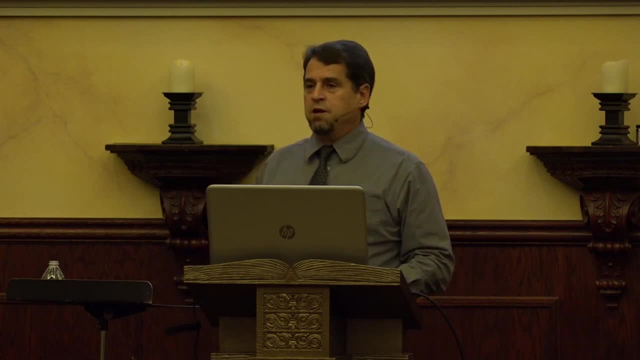 an airplane, But it was seeing the area from an airplane. that finally convinced them. It hauled massive boulders. In fact, huge gravel bars around the Willamette Valley are due to the Missoula Flood. It deposited mass, mass, monumental amounts of gravel in the area, as well as the 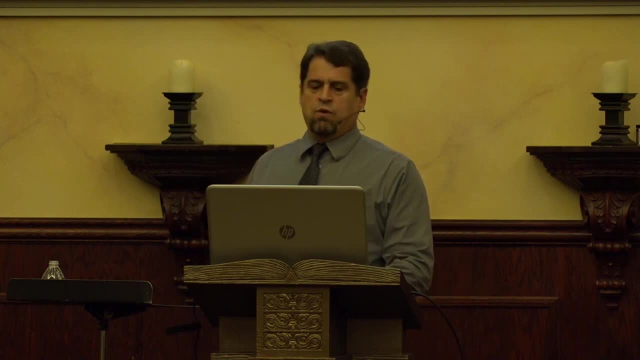 huge boulders called erratics. This is from the erratic rock state natural site in the Willamette Valley, Oregon. The rocks that you see there were carried there from the Missoula Flood. Flood water is so powerful, so much force behind them. they were carried, huge boulders, along with 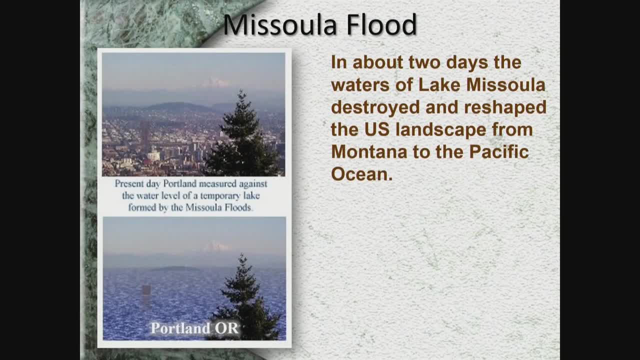 them. Portland, during the flood, would have been completely underwater. It's estimated it was 400 feet deep. Portland would have been 400 feet underwater or the flood waters were over 400 feet deep at this location And, traveling At 90 miles per hour, it is estimated that they were equal to 10 times what is found in all the 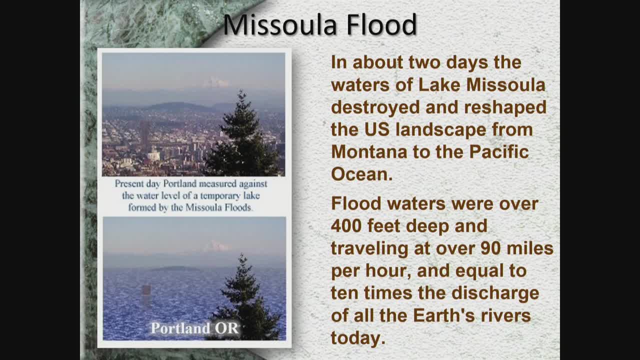 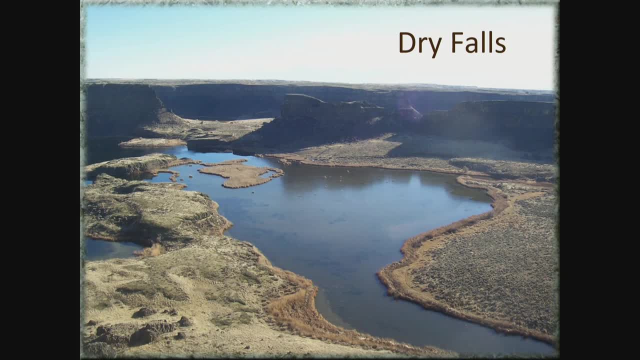 Earth's rivers today. That's a monumental flood. It formed during this flood. there would have been a huge waterfall at this location. There's a state park out in eastern Washington called Dry Falls State Park where you can stop in and overlook and look at the remnants of what was a 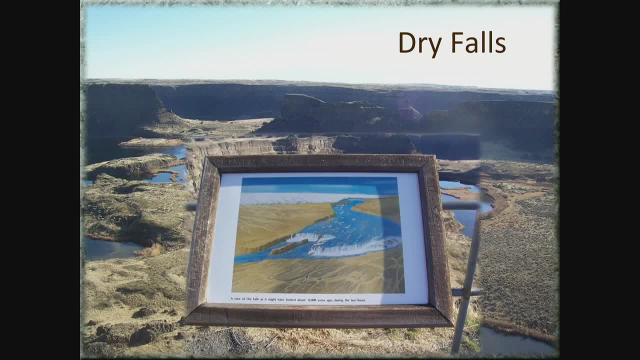 massive waterfall. There's an artist's conception on the railing Just at one of these overlooks. that gives you an idea of what the waterfall would have looked like. But this is a really massive geologic feature not well captured by photograph, So I took a video out. 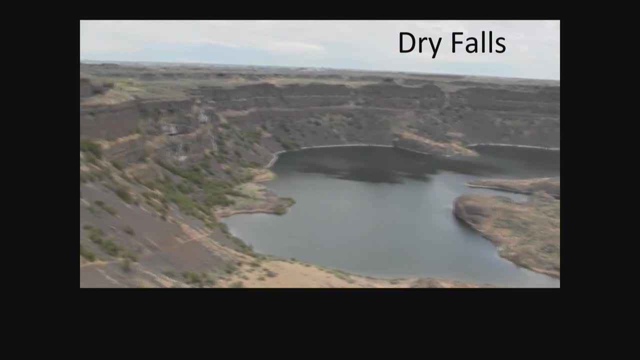 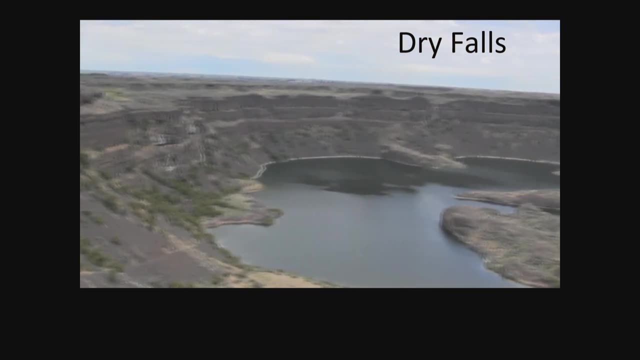 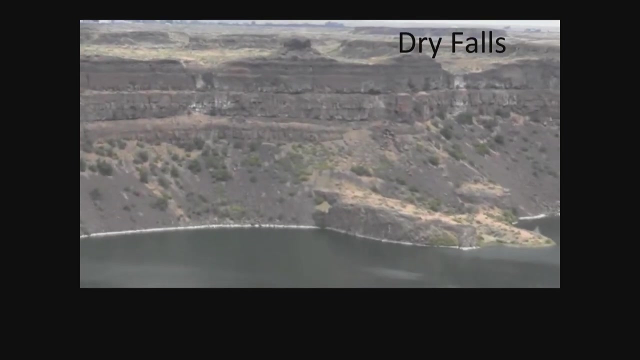 there when I was there a few years ago to try to get a little better idea of what you're looking at here. This is a massive, massive waterfall. It is estimated that it's close to three and a half miles wide, with a drop of 400 feet. 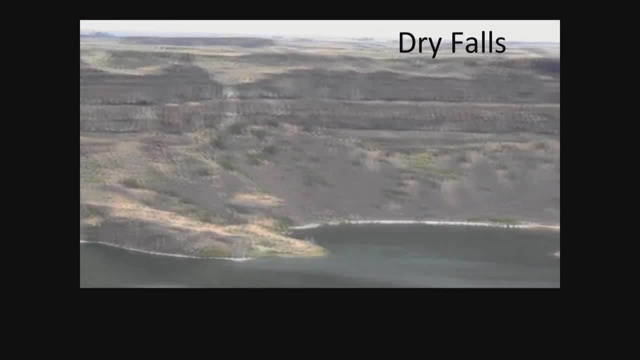 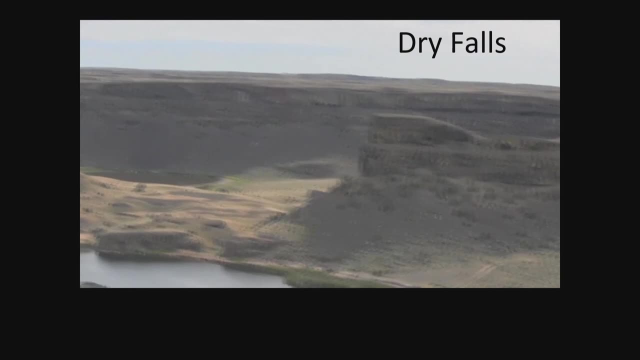 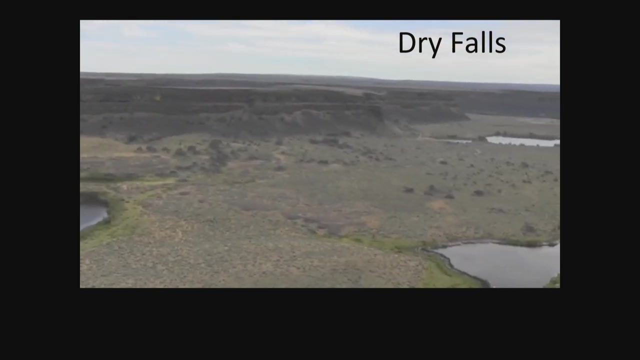 By comparison, Niagara Falls is one mile wide and drops 165 feet, So this is three times the size of Niagara Falls. As I pan to the right, what you'll see is the Grand Coulee, The picture that I showed you previously- the Grand Coulee. the Grand Coulee actually exists on both sides of Dry Falls. There's. 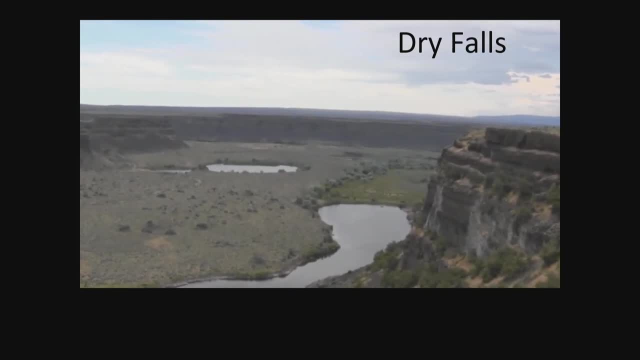 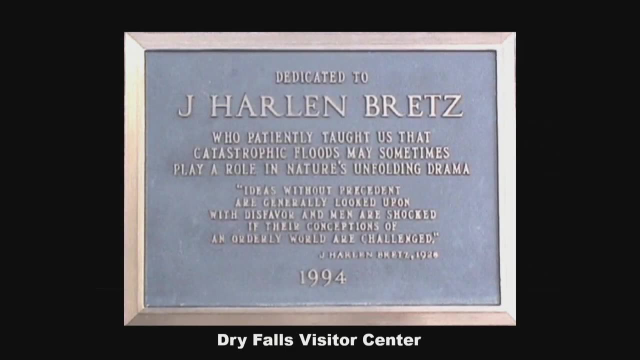 an upper and lower portion, but that's the Grand. that's what I showed you in the photograph board. that's the Grand Coulee, Massive, massive canyon that was formed by this flood. The Dry Falls Visitor Center was dedicated to Hardin-Bretts in 1994.. The plaque there can be found just outside. 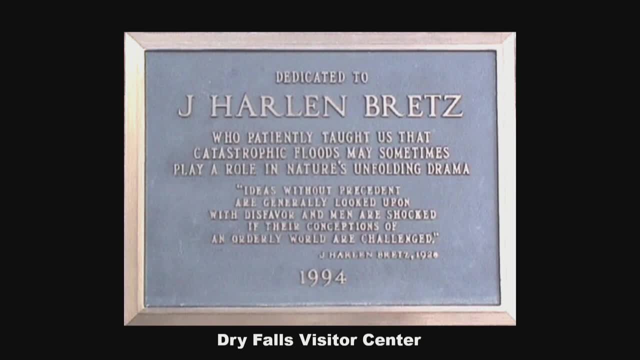 the facility, It reads, dedicated to Hardin-Bretts, who patiently taught us that catastrophic floods may sometimes play a role in nature's unfolding drama. And there's a quote there from from Bretts. He said: ideas without precedent are generally looked upon with disfavor and men are shocked. 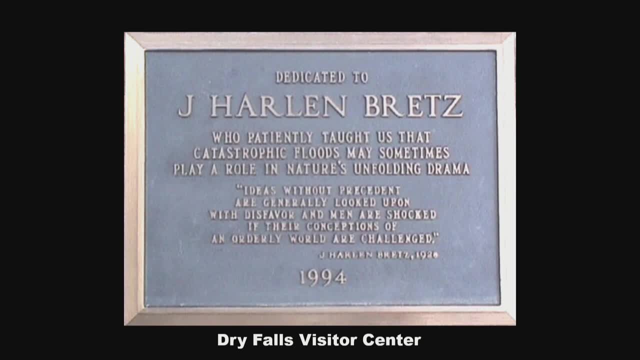 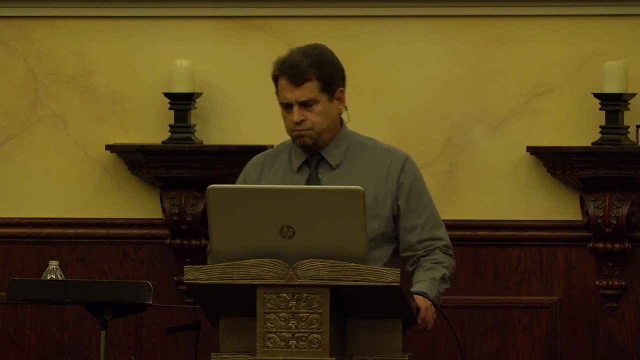 if their conceptions of an orderly world are challenged With such bias influencing the interpretations of geologists today it's it is assumable that all geologic features formed during the global flood would be misinterpreted And it would have been argued that they have formed through other mechanisms. 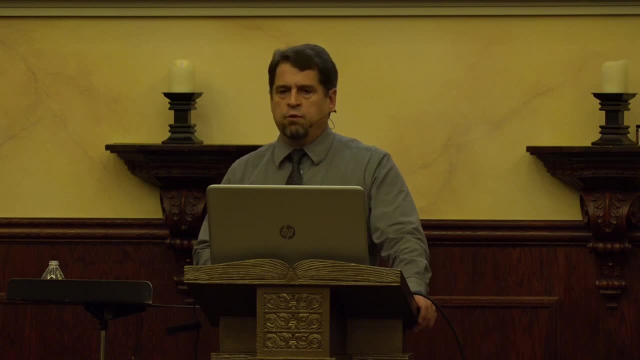 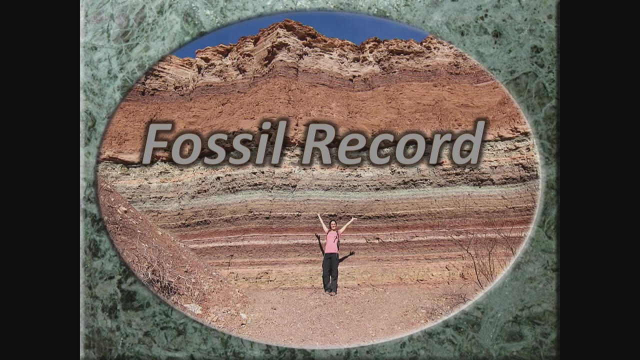 than a catastrophic flood. This is assumable. So, with this in mind, we're going to kind of take a tour of some geologic features and I'll try to, as best I can, argue for a different interpretation. That is, that what you're looking at is a geologic feature that has been formed during the global flood. 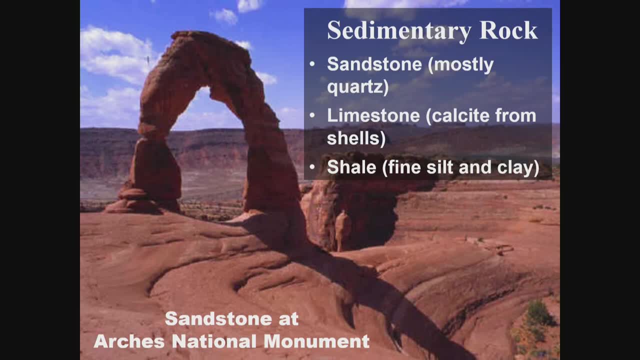 Looking at by way of these geologic features is, in fact, a monument to the devastating flood brought about by God for the judgment of the people on the earth in those days. Sedimentary rocks are a key part of geology today. Sedimentary rocks form when sediments 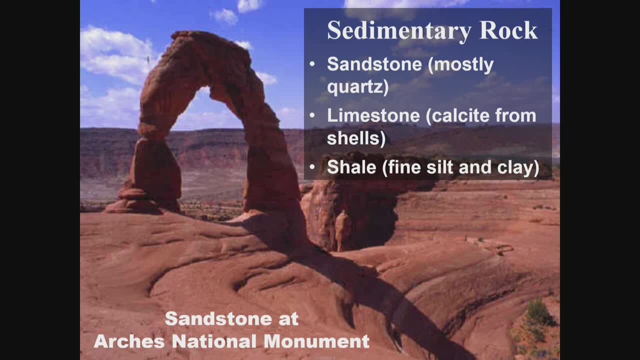 these are just eroded particles that are suspended in fluids, settle out of the fluid and then harden into a rock. There are three main types of sedimentary rocks: Sandstone, which is made up of sand particles shown here at Arches National Park. 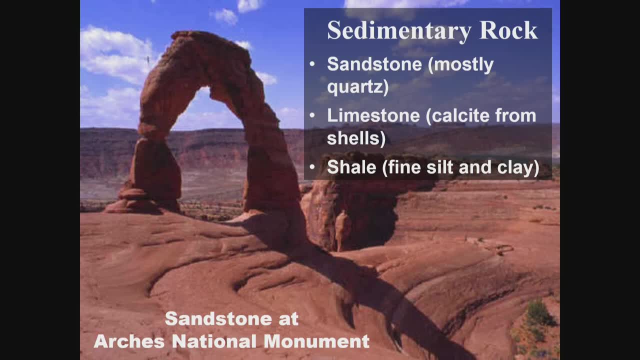 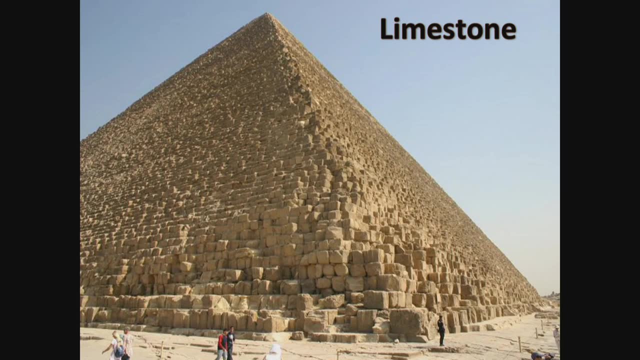 Shale is another type that is made up of finer particles of silt and clay, And then you have limestone. Limestone is a sedimentary rock composed of calcium carbonate or hardened by calcium carbonate from the invertebrate exoskeleton debris. So it's a rock. that's. been cemented together by calcium carbonate That's coming from the exoskeletons of vast invertebrates. Pretty much all of them have calcium carbonate as part of their shell. In most places, sedimentary rocks are hundreds of feet thick. In places they reach kilometers of. 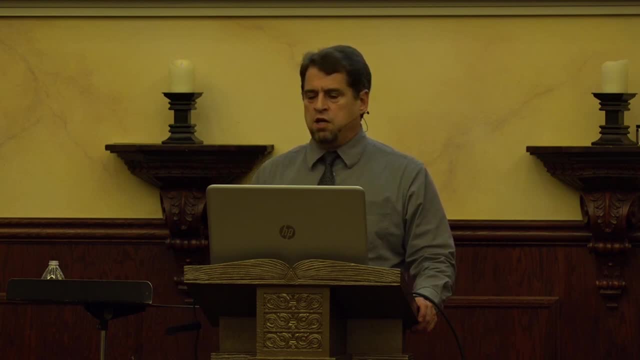 thickness, And so vast and monumental are these sedimentary rocks that they have been used as building materials since the flood. The pyramids, as you see here at Giza, as well as the Sphinx, were entirely made out of limestone. If you've ever been to Israel, in Jerusalem, all of the 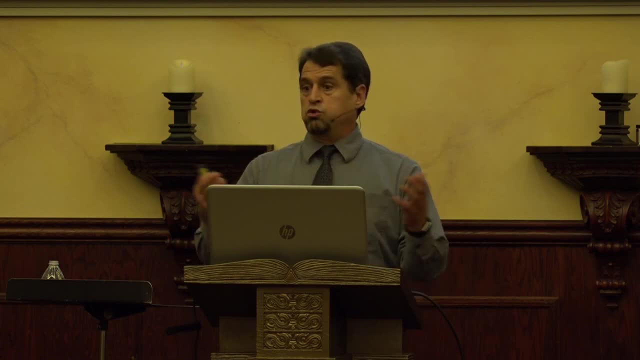 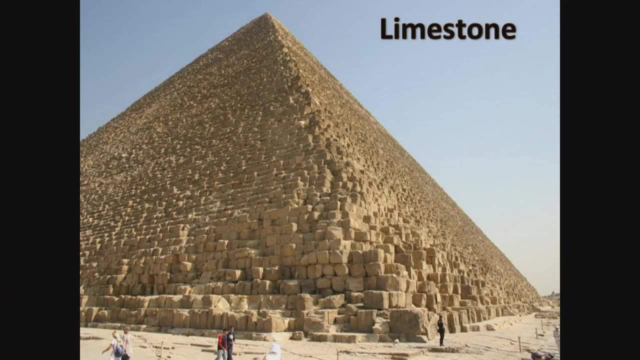 stones that you see there in Jerusalem are it's what they call a Jerusalem limestone: All the pavement stones there and the stones that were made to build the walls, the retaining walls, and all that's all limestone. Massive amounts of sedimentary rock exist. It is a powerful. 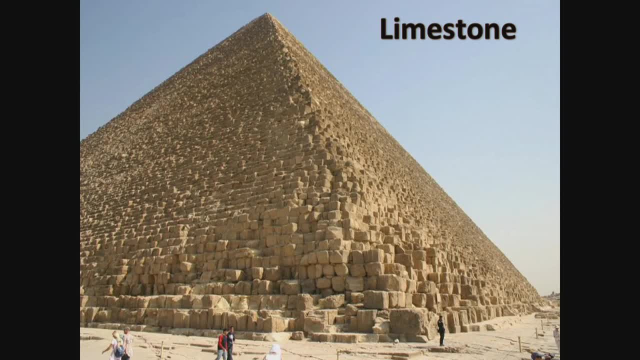 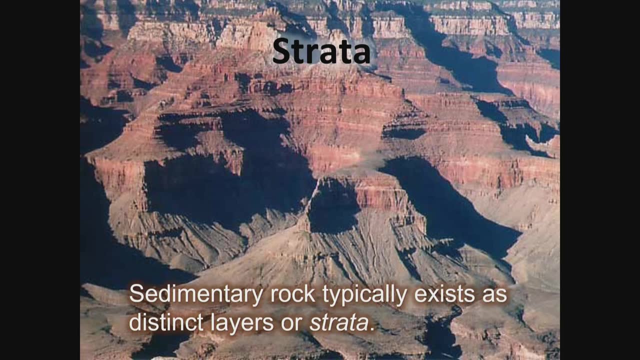 and monumental body of evidence to support a major global scale catastrophe. This sedimentary rock exists in distinct layers, that is called strata. Now, geologists generally view these various layers of rocks as forming in different depositional environments, Meaning so when something is deposited. so there's different kind of environments that these 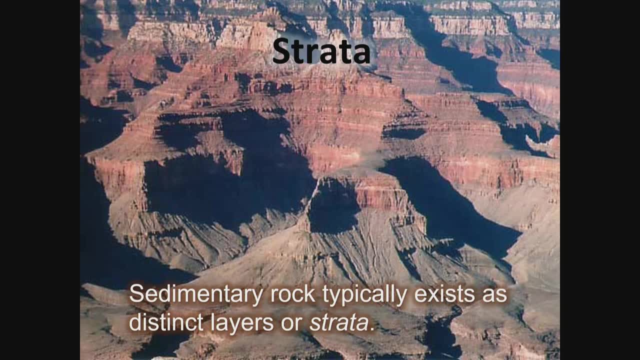 sediments could form in. It can be a desert, or it can be a lake, or it can be a swamp, or it can be a ocean- can came in and inundate, But- and these various layers are believed to be due to a changing depositional environment- It was a desert there for a while. Then the ocean came in and 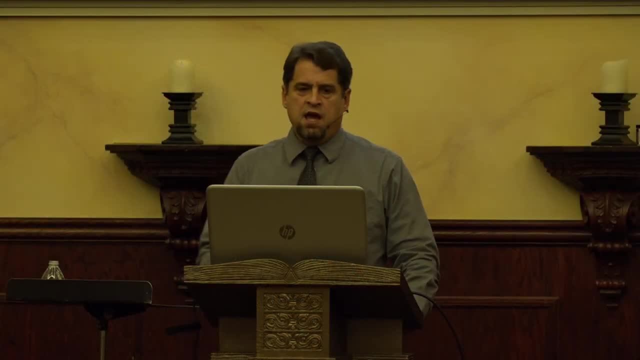 flooded and deposited some limestone on top of that desert sand, And then the ocean receded and it was a swamp for a period of time, producing silt And then maybe a sand. some sand was deposited later. This is their interpretation of the layers of rocks, Like you see here in the 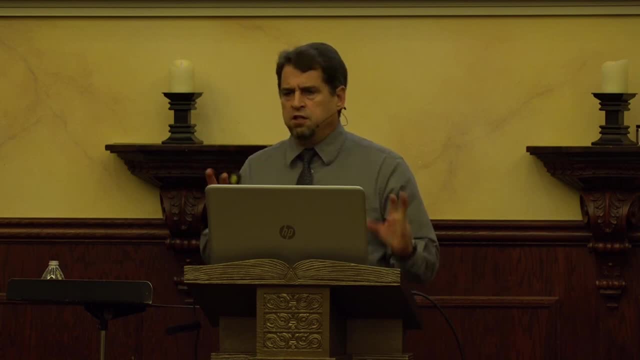 Grand Canyon. It is this fossiliferous or fossil containing strata that is referred to as a fossil record Because the layers are. it's called a fossil record because these layers are believed to be a recording of periods of time, Much like tree rings or ice cores have layers that can 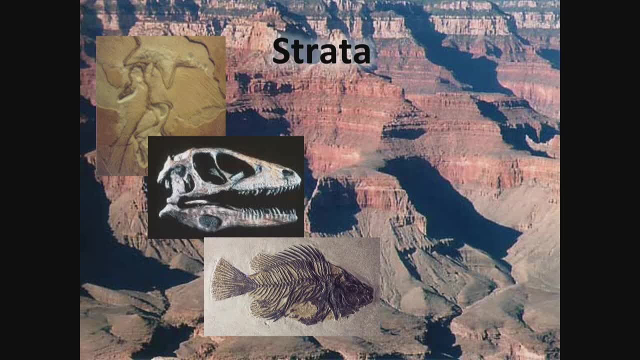 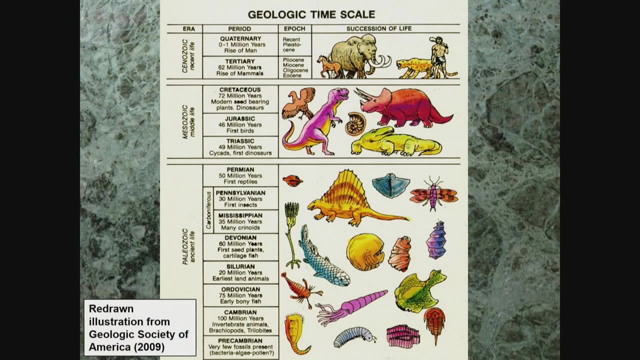 record a sequence of events. These layers of rocks are are recording a sequence of events as well and are thought to be chronologically distinct from one another. Therefore, the fossils found in these layers of rocks are interpreted as being separated by vast eons of time and representative of the life on earth over what is called geologic time. 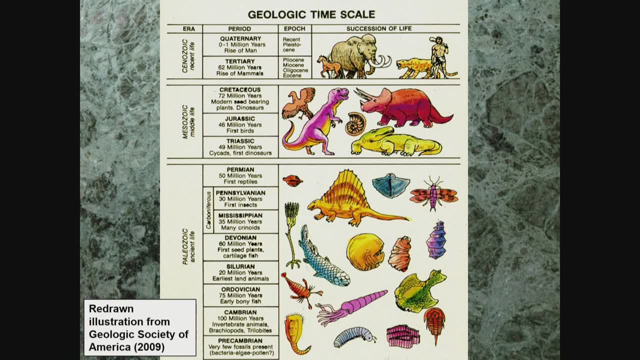 The sorting of fossils, the fact that the fossils are- are they there are typically, what you find are certain fossils below or above other fossils. And to a uh, to an evolutionist, this is proof that life on earth has changed over time And it's changed. 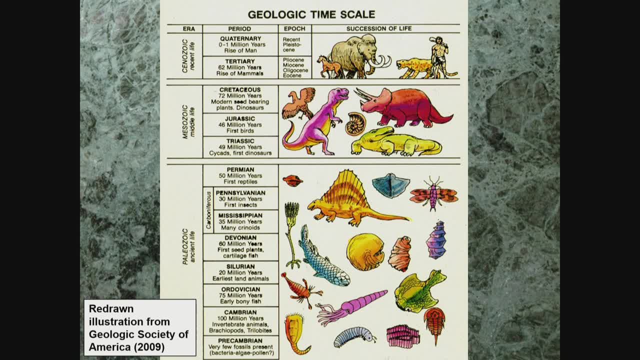 from simple to complex forms. Um, when it was realized that fossils were sorted, this was a great source of confusion to many Christians, many Bible believers, who had previously assumed that what they were looking at was a result of a global flood When they when geologists started. 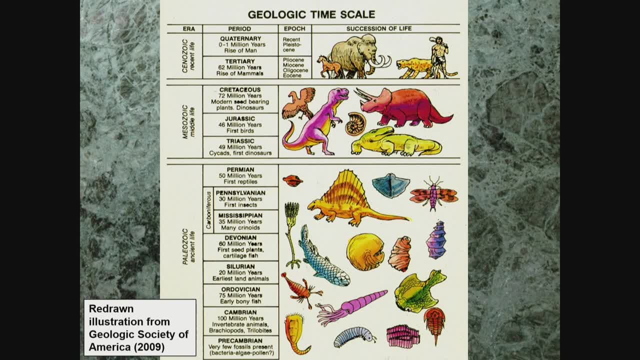 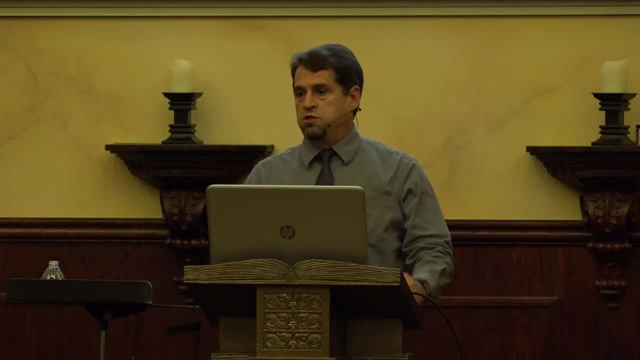 illustrating that fossils are often found below or above other fossils, and they argued that what you were looking at was, uh uh uh, the history of life on earth represented in rock layers. This was a great source of confusion, because I guess they believe that, uh, from a global flood, all the fossils would be just all found, jumbled together in one great big mass. But we got to remember that the flood itself lasted an extended period of time, a full five months. The flood lasted from the 17th day of the second month of Noah's life to the 17th day of the 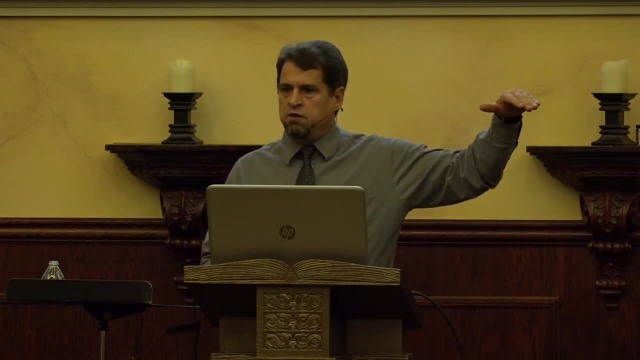 seventh month of Noah's life. That's how long it took before the, the flood reached its climactic height And and the last animals died as close to five months after the beginning of the flood. Flood was an extended event, And we believe that what we're 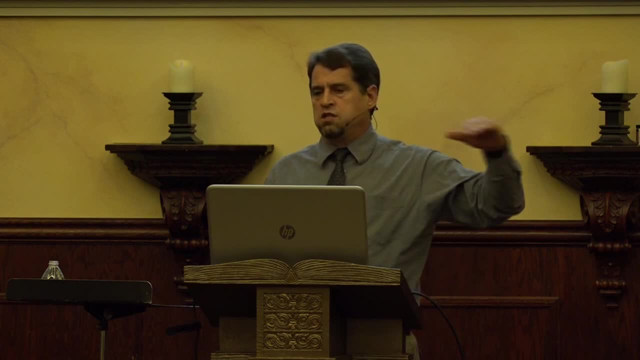 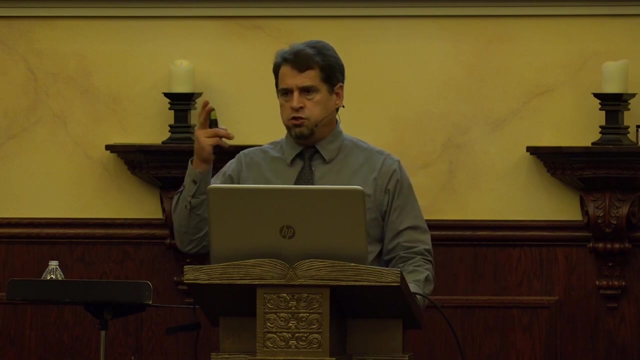 looking at by way of the fossil record, is just the destruction of successive life zones, destruction of successive habitats. Different communities of organisms live at different elevations. They your different habitats or biomes on earth are largely due to two different, two main abiotic factors. 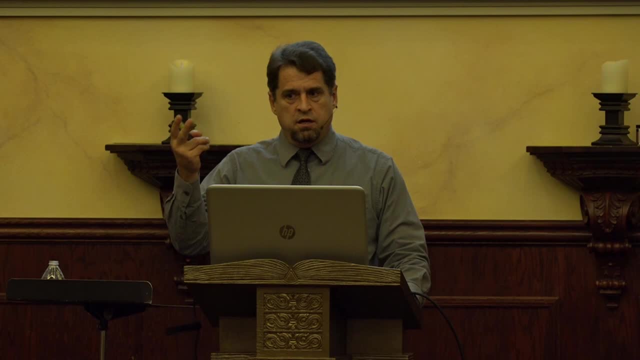 Temperature and water. The amount of the amount of water in an area and the temperature of that area largely determines the communities of plants and animals that will live there, And the temperature and amount of water is heavily influenced by elevation. So these different habitats generally are correlate by elevation And we believe that what you're looking at there 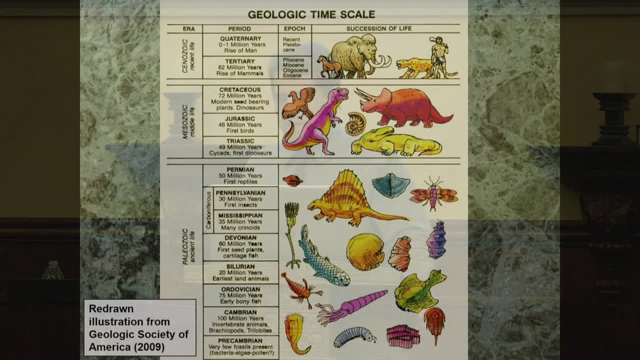 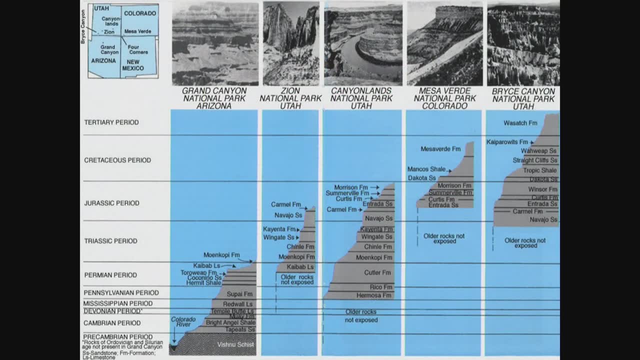 is just the destruction of successive habitats during the flood. That's all it is now. but, unknown to many, the fossil record like you see here in this diagram, which is more formally called the geological column, was actually assembled by correlating layers of strata for many different locations. It is said that the entire fossil 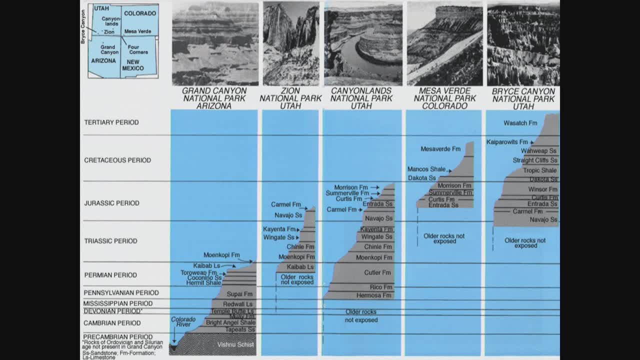 record doesn't exist, except maybe on less than 1% of the earth's surface. Just a little piece of it exists here and a little piece of it over there. but I'll show you what they did. This is a graphic that was made by the US Geologic Survey to illustrate this point By correlating layers. 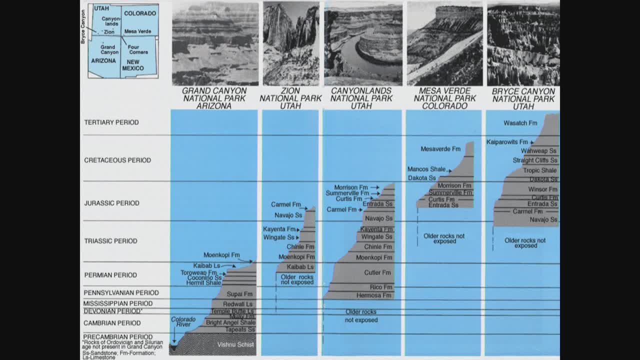 that are exposed in different areas. they eventually came up with the entire geological survey, And so this is the entire fossil record, or what we call the geological column. So, for example, the Kaibab limestone- I don't know how well you can see this diagram, the Kaibab limestone that I've circled. 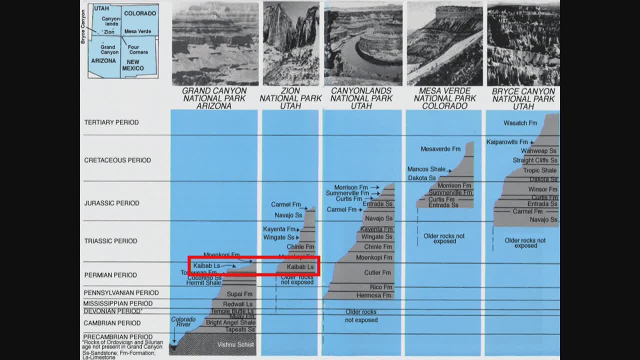 there can be found close to the top of the Grand Canyon but on the bottom of the exposed layers at Zion National Park in Utah. The Navajo sandstone that I've circled here and some other formations can be found both at Zion National Park and Canyonlands National Park there in Utah. 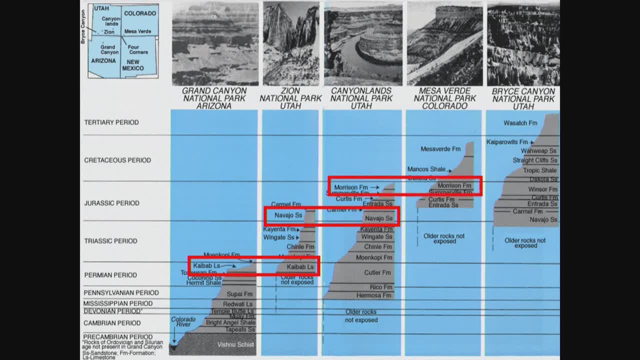 the Morrison Formation circled there, which is rich in dinosaur fossils, And Morrison Formation is a dinosaur graveyard massive. literally thousands of dinosaur fossils can be found in Morrison Formation. It can be found at both Canyonlands and Mesa Verde. The Curtis Formation. 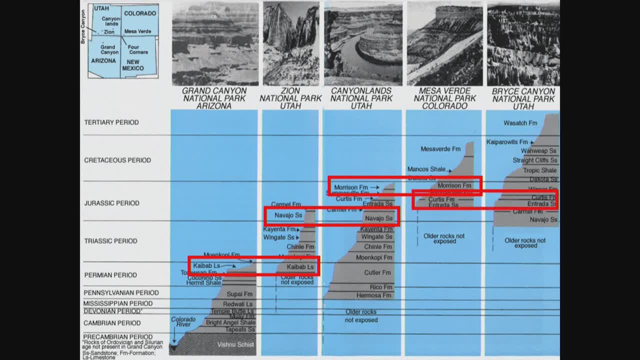 and the Entrata Sandstone can be found in both Mesa Verde and Bryce Canyon. By comparing these layers at various locations, they eventually put together what they believe is the view of the history of life on earth, represented by the Kaibab limestone. And so this is the 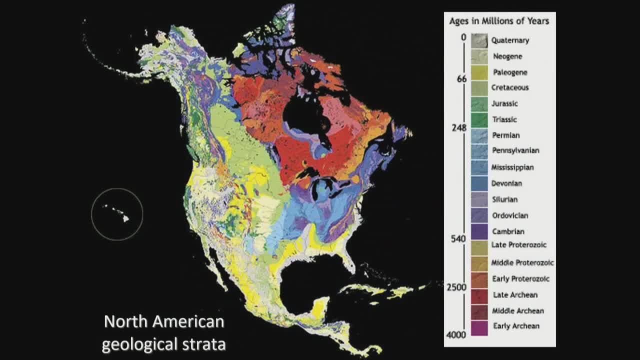 map of the Kaibab limestone that I've circled here. All the layers again of the fossil record, though, are said to be found in much less than 1% of the earth's surface, And this is well illustrated by this map, also made from the US Geologic Survey. Now, I didn't point out the names. 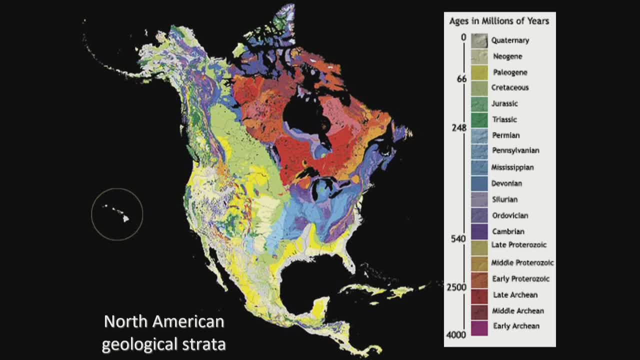 to you the various names of these geologic periods, but you can see them on this map of the Jurassic period, the Triassic period, the Permian period. These are periods of time, geologic time, And these are color-coded for you to show which periods are on the surface in. 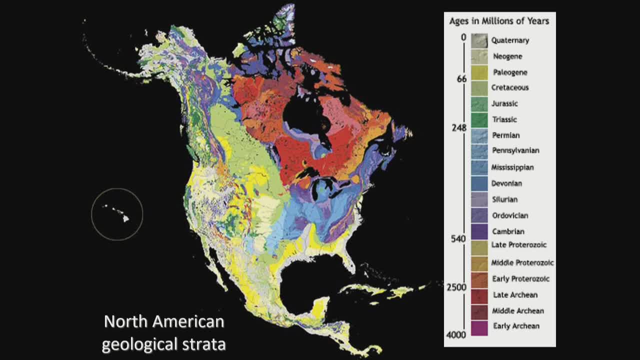 North America. Now, one of the things I want you to note on this diagram: take a look at where the reds are on the map and take a look at where the reds are on the scale on the right. So all of this. 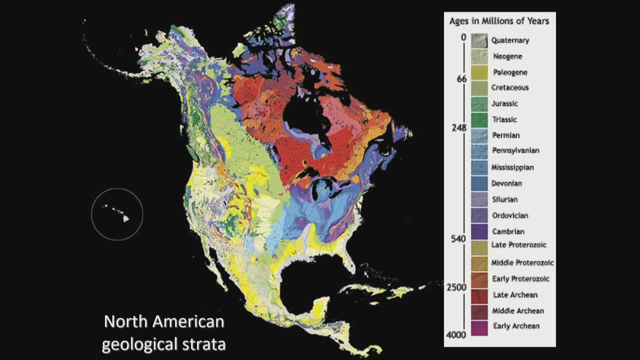 area up in northern Canada where you see reds. look at now the scale of geologic periods. All of those geologic periods above the reds are all missing from that entire region. The entire fossil record cannot be found except in a few places. They say even like less than 1% of the earth's surface might contain. 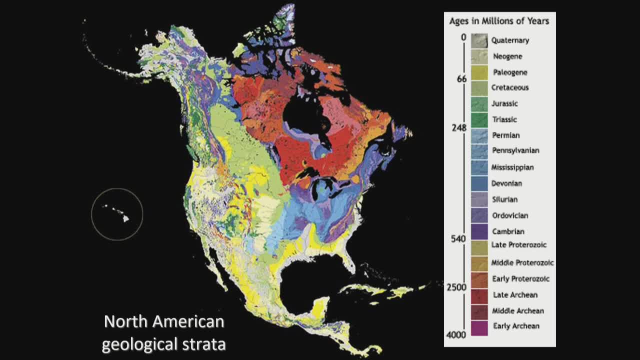 the entirety of this geologic record, but the reality is you only see a piece of it here or there, But that it's missing from that entire area of Canada is very telling. There's something else I want to point out while I have this map up, and that's this: Remember the reason why they. 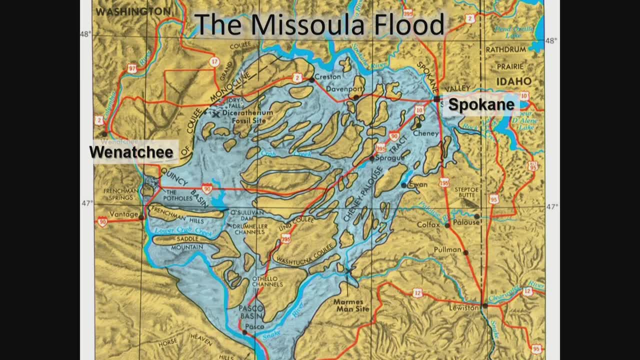 couldn't recognize the reds. They couldn't recognize the reds. They couldn't recognize the mausoleum flood. The reason why they couldn't recognize that eastern Washington was destroyed by a major flood is because it was too big. The geologic formations out there were too large for. 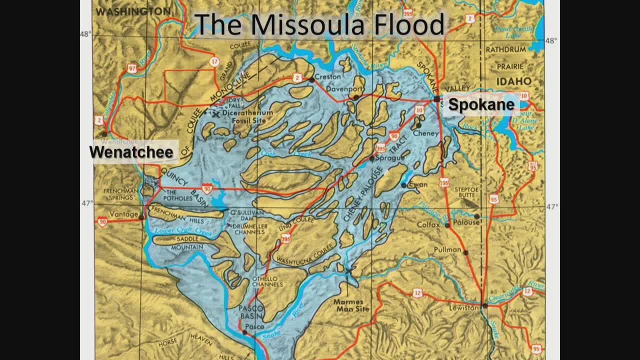 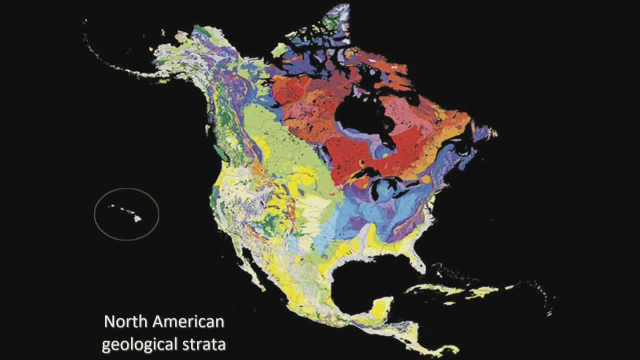 them to recognize that they were catastrophic formations until they viewed them from the airplane. But if they couldn't recognize that the mausoleum flood was a result of a catastrophic flood, how are they going to recognize that something like this is the result of a catastrophic 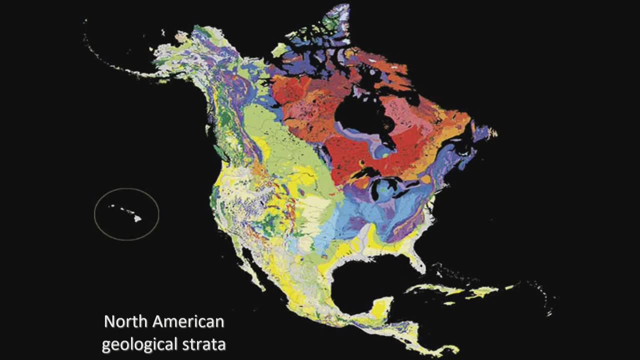 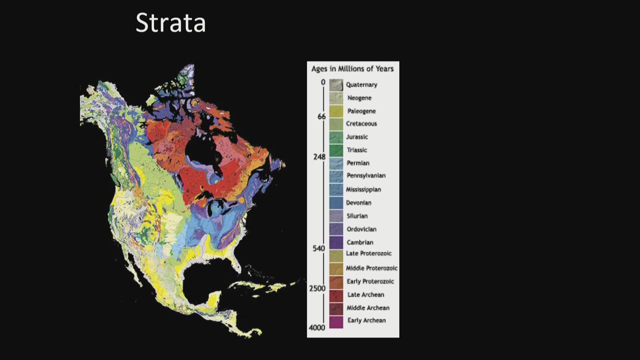 flood. I mean, they're so far from the truth in this matter that it's ridiculous. There's. I want to show you I had actually used this map for years in a talk on fossils and geology like this, And then suddenly, like it was last year, suddenly this map reminded me of something that 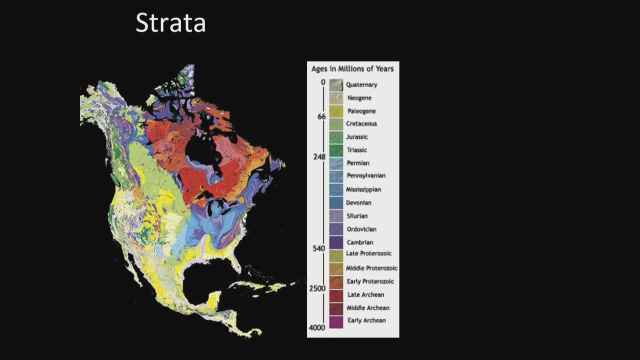 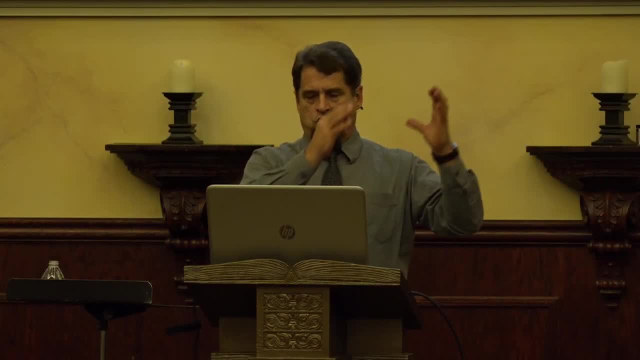 I use in my biology classes. When we're talking about ecology, one of the things we get into are the different biomes. So a type of habitat is what we call a biome. Like there's grasslands and you've got your coniferous forest and you've got your alpine meadows, the great. 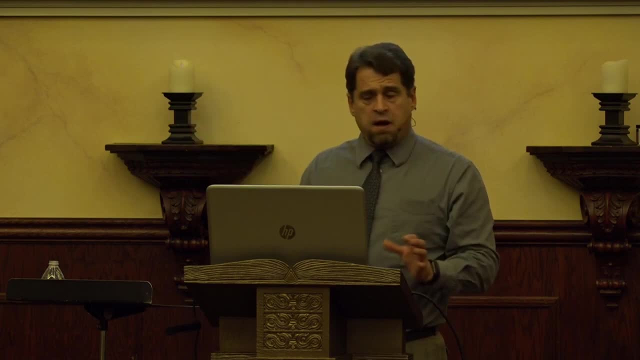 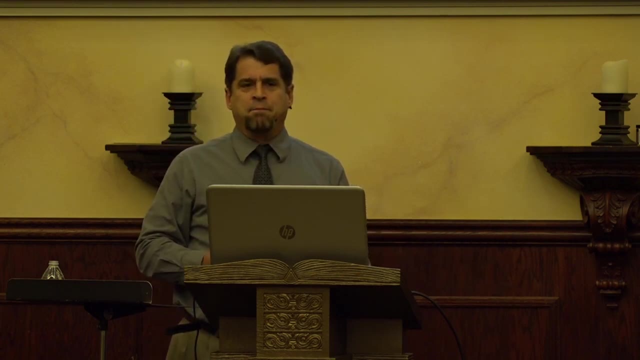 plains around the United States. These are the various biomes, And at some point, having used this map for years, suddenly this map reminded me of a biome map, a map of the biomes that we see in North America. And so, just to see, I did a quick search on Wikipedia and found a biome map. 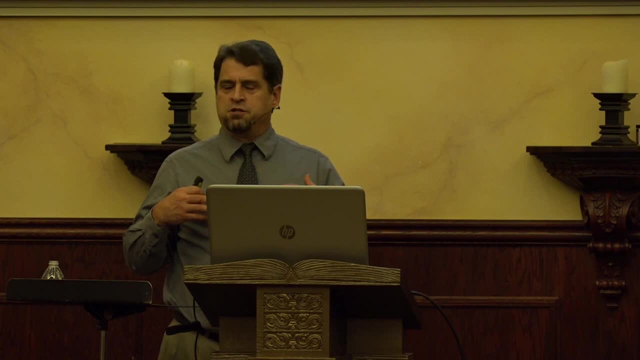 of North America And I want you to remember, if our interpretation is correct, to the fossil record, what you're looking at is the destruction of successive habitats And if that interpretation is correct, then perhaps we're going to be able to see the destruction of successive habitats. 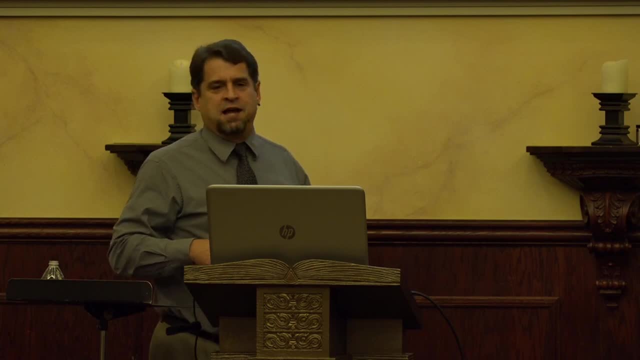 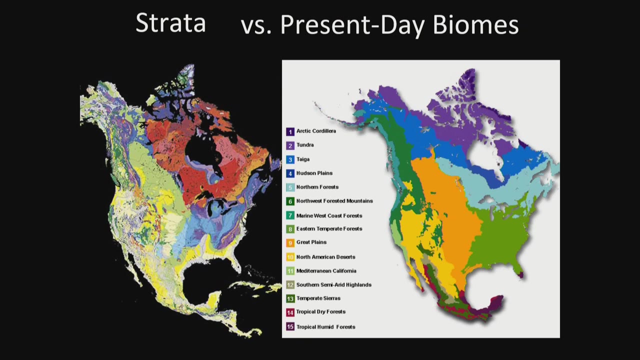 Perhaps it will very closely match the present-day habitats found in North America. So I found a map, and there it is. That's a map of the various biomes that are present in North America, And just look how eerily similar these two maps are. I mean you can see where some of the lines are. 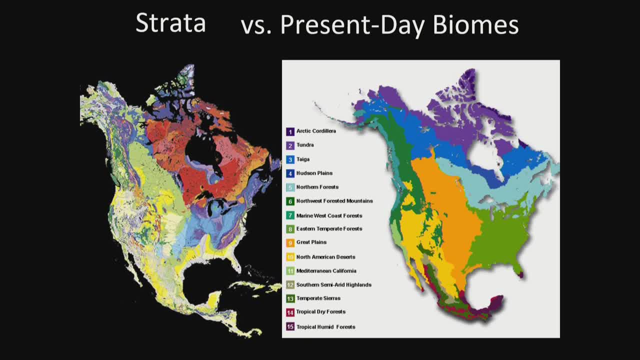 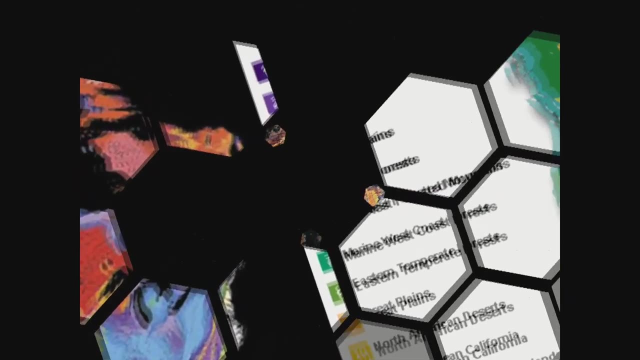 just in the exact same place, the line that goes to the Great Lakes, for example. I mean, that's all you're looking at in the fossil record really is the destruction of successive habitats. That's all you're looking at. Okay, let's analyze strata formation. Okay, remember, strata is just 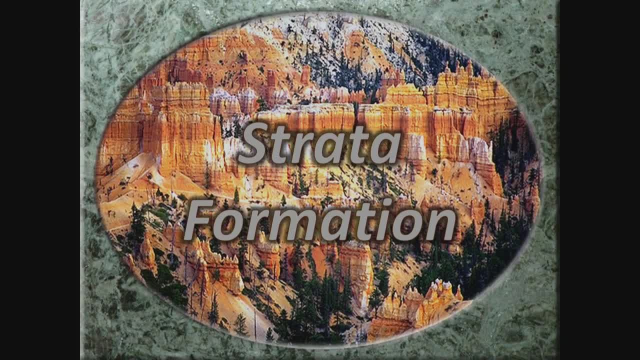 the fancy name for these layers of rocks that sediments are found in. And remember, as we said before, geologists generally view various layers of rocks as having formed in different depositional environments. So you had a desert there once, and then you had ocean, came in and inundated. 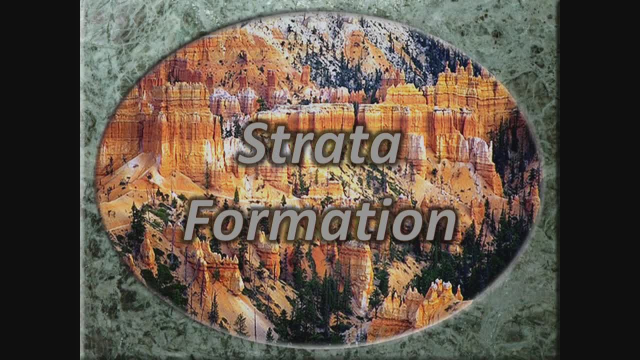 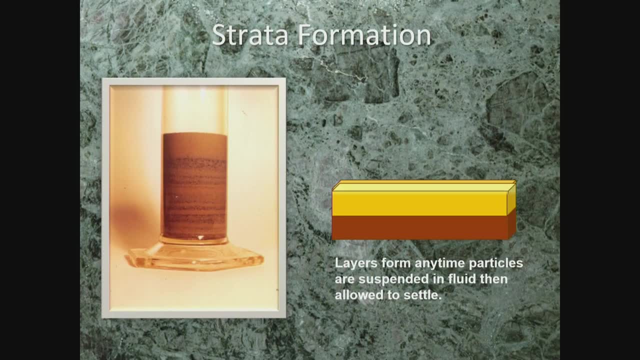 and laid down limestone, or then it became a swamp for a period of time. That's the general interpretation, But experimentally we know that layers do not require vast periods of time and they don't require changing in depositional environments to form. All you have to do is take a column of dirt. 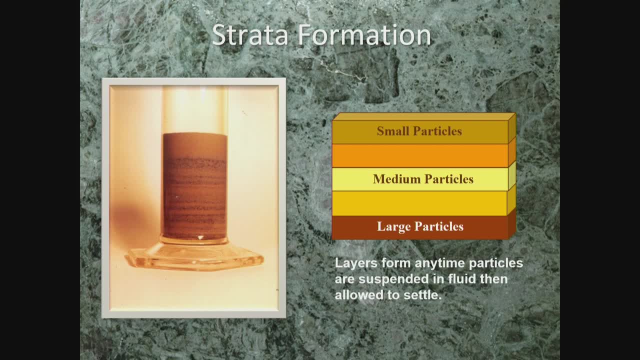 like this and shake it up and it will settle out into different layers automatically. The different size of particles, the different mass of these particles, the different shapes of these particles, all three of those factors will affect the rate at which they settle out, cause them to settle out. 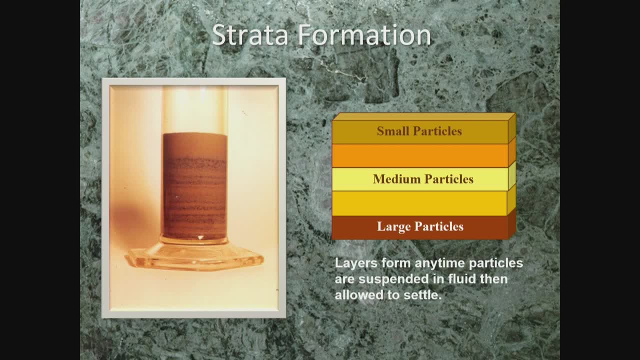 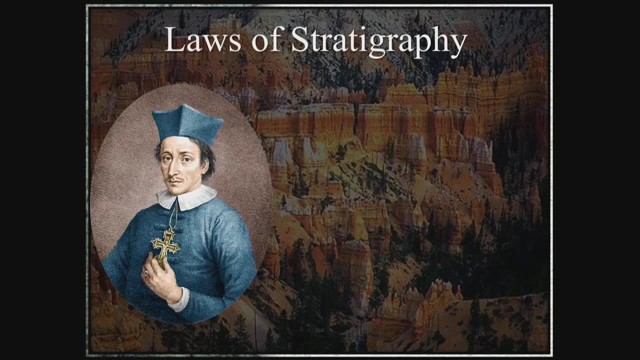 at different rates and you have different layers forming automatically. And I want to illustrate this for you a little bit better. In 1669, Nicholas Steno, shown here, outlined the principles of stratigraphy, strata formation. the principles of strata formation. 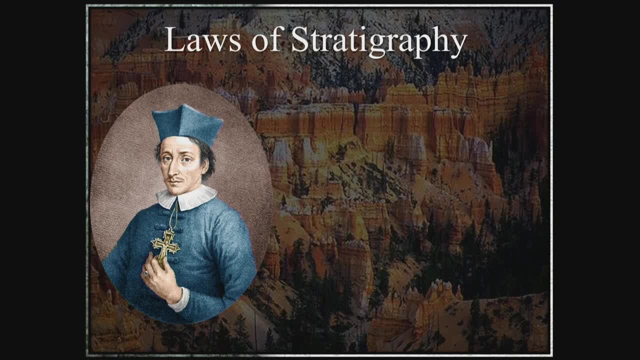 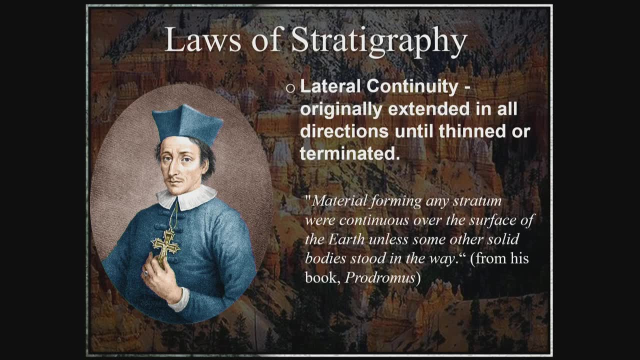 which are now more commonly called the laws of stratigraphy. These include number one, the principle of lateral continuity. It is believed that originally, this stratigraphy strata that we find on the earth extended in all directions until it either thinned at the 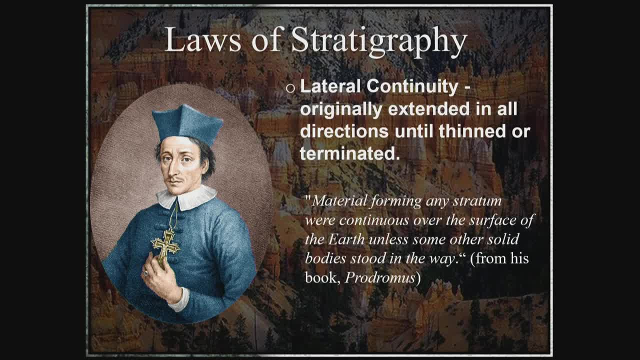 continental shelf at the ocean, or was truncated by another geographical barrier, like a mountain range. It is believed that all the strata was laterally continuous or horizontally indefinite. This law of stratigraphy is due to the observation that the layers of sedimentary rocks that are 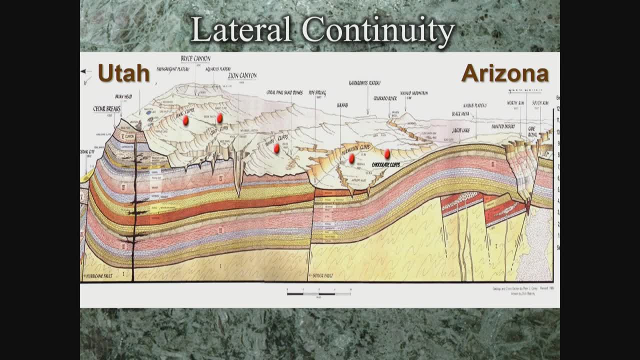 exposed in places like the Grand Canyon, etc. can be traced for hundreds and in some thousands of miles. The grand staircase that you see here, the grand staircase that you see here, the grand staircase, is an immense sequence of sedimentary rocks layers that stretch from Bryce Canyon through 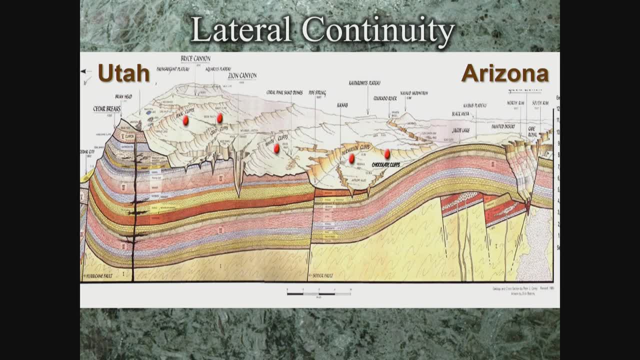 Zion National Park and into the Grand Canyon. These layers are laterally continuous or horizontally indefinite. It's a monument to a devastating catastrophe and it seems so obvious to us. Steno's other principles of stratigraphy were the principle of superposition. 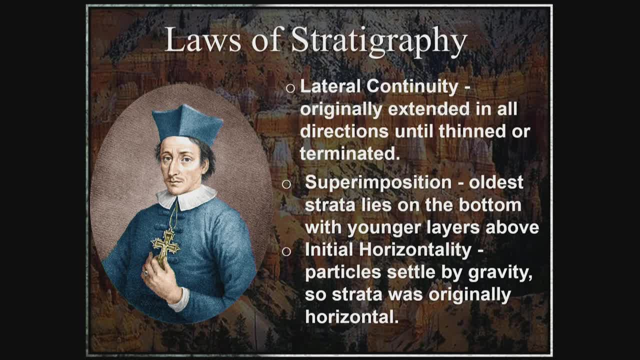 That old, the oldest strata lies beneath younger strata, That the layers that you see here are oldest to youngest. Older one has to be on the bottom before a newer one can be laid above it. This makes great, perfect sense, And also the principle of initial horizontality. 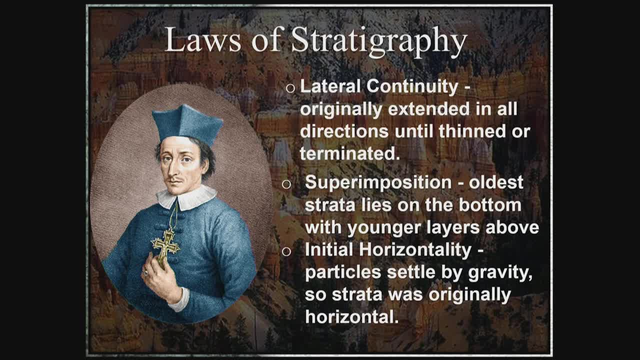 Because these sediments are drawn by gravity. it is argued that originally they were laid down horizontally, And this is important because many of them are not horizontal. today We can find a lot of them that are horizontal, But the principle of initial horizontality is that they are. 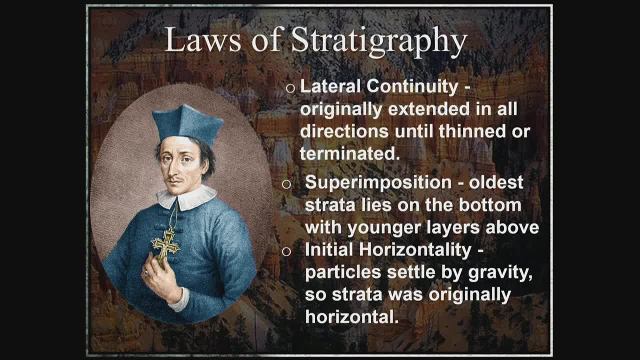 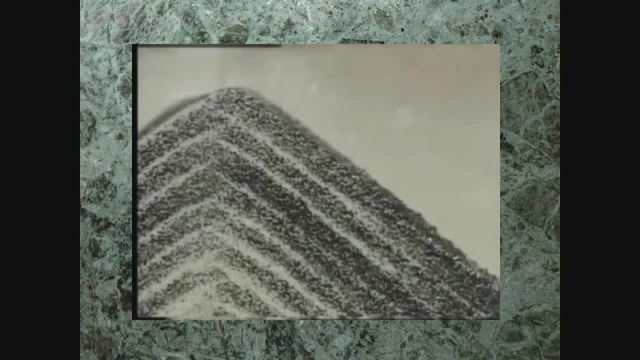 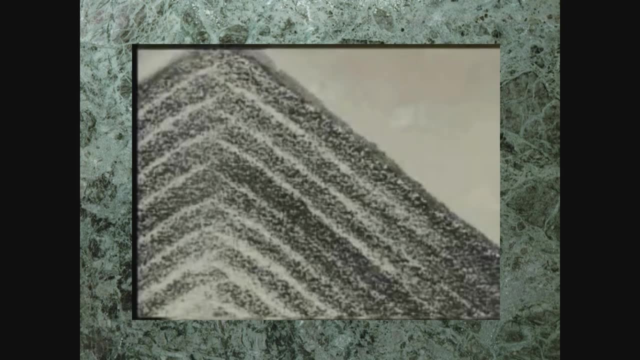 seriously bent and uplifted, But a simple demonstration can show that these laws are often not true. Look at this simple video. These light and dark particles that are being poured down not only form distinct layers at the exact same time, but the layers are not forming. 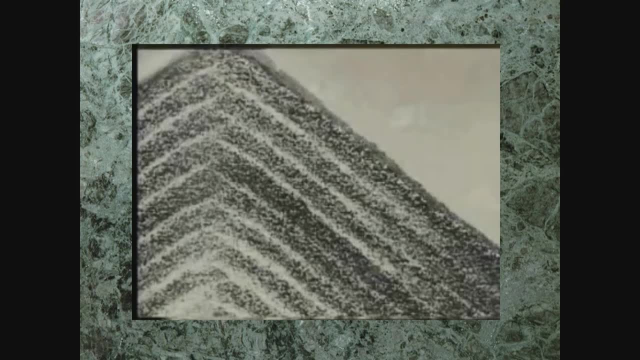 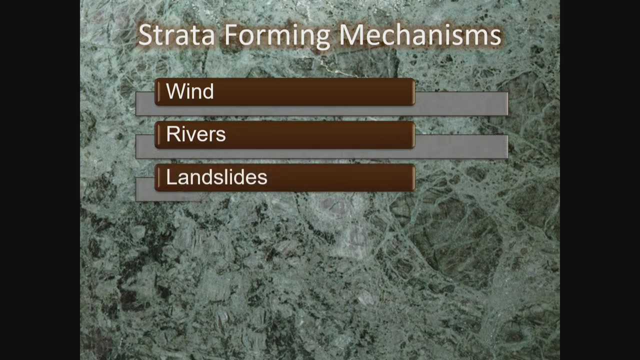 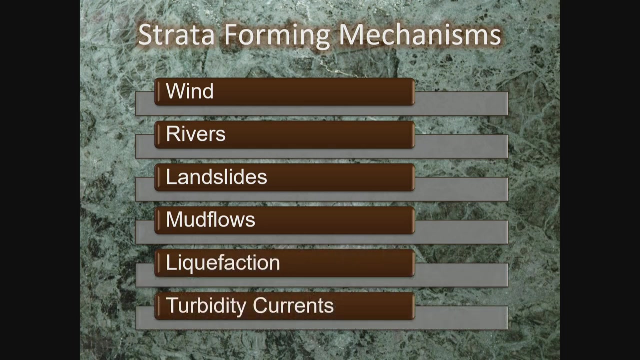 horizontally. either Particles of different densities or sizes or shapes will separate into layers when simply rolling downhill. There are a number of physical properties, processes, that will suspend particles And, by just suspending particles for a brief moment, the different sizes of those particles, the different masses of those particles. 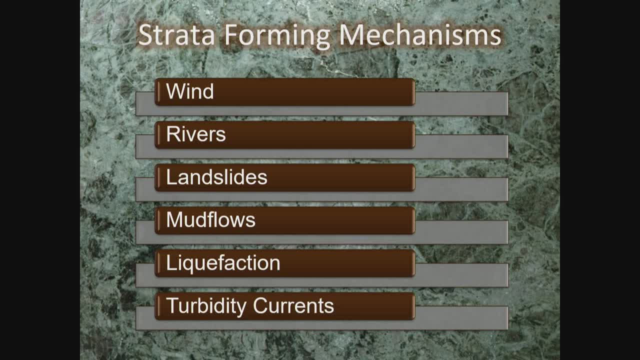 the different shapes of those particles will allow them to settle out into distinct layers. Many physical processes will allow strata or layers of rocks to form quickly. We already know some of these Wind river. you guys all know what some of these are. 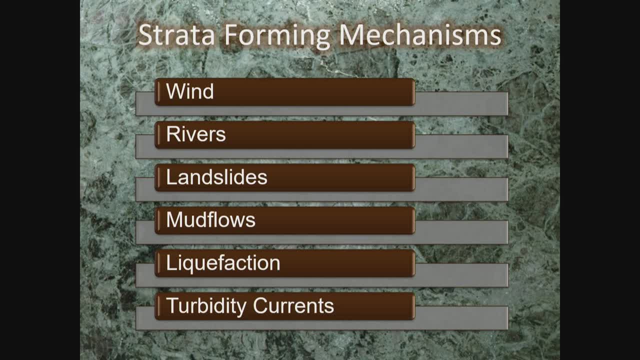 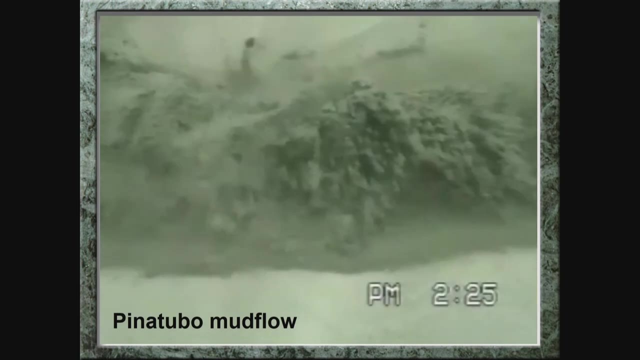 Liquefaction and turbidity currents. I'll show you what those are, But let me show you mud flows. Most people don't realize just how significant mud flows are in being able to form distinct layers of strata. Mud flows are themselves terribly, terribly damaging events. It can cause massive erosion, very, very powerful. 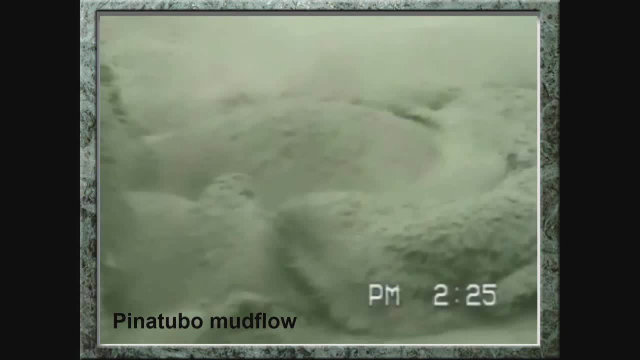 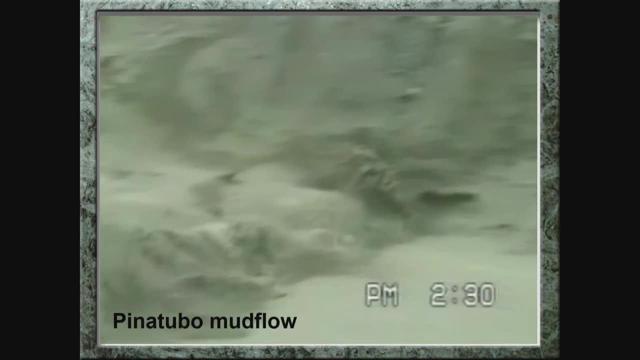 erosion forces with mud flows, But they can form strata instantly. Mud flow is basically a landslide that's just in a slurry saturated by water and flowing through the air, And it's a very, very dangerous event, And it's a very, very dangerous event, And it's a very, very dangerous event. 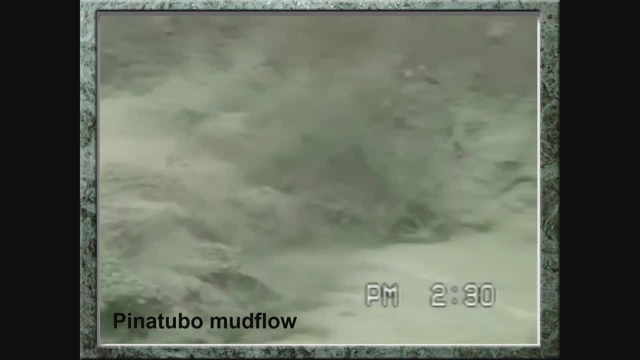 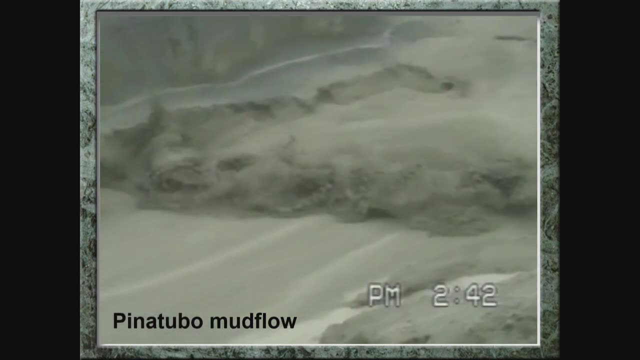 This is actually a mud flow at Pinatubo, But we had mud flows at Mount St Helens. I'll show you some of the layers of rocks that were laid down by mud flows at Mount St Helens as well. Those mud flows not only powerful erosion forces but, as this body of material is flowing, 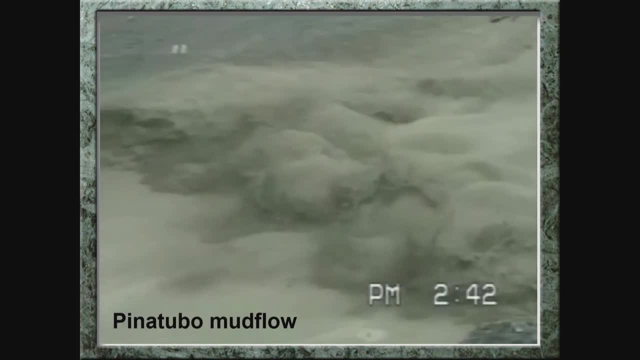 those particles are suspended And that suspension gives them time to settle out at different rates. And all mud flows, all landslides form strata, Form layers of rocks that when you come back afterwards you can see these layers of rocks. Liquefaction is another that is able to produce layers of rocks. Liquefaction occurs when 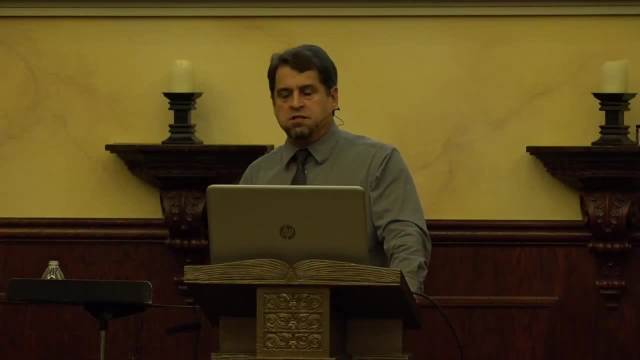 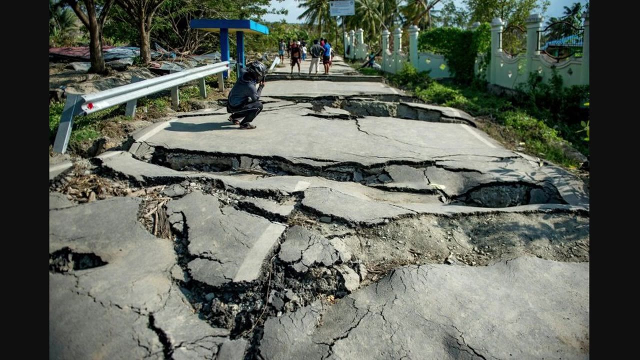 vibrations or water pressure within a mass can cause soil particles to lose contact with one another And then they behave like a liquid. Liquefaction is usually a very temporary thing and is often caused by earthquakes, vibrating, water saturated or water filled or unconsolidated. 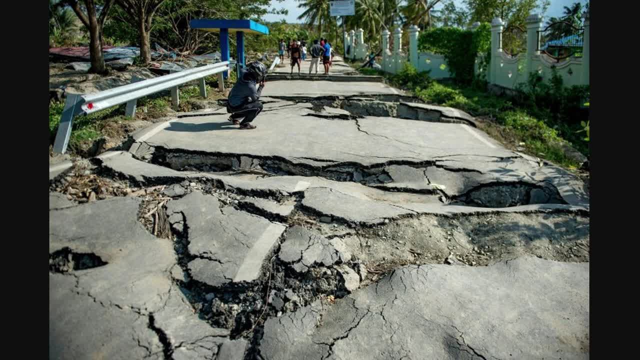 soil And it's a very, very dangerous event. And it's a very, very dangerous event And it's a leading to rapid stratification. When they come back into those soils later they find that it's all stratified. It doesn't take long. Any physical process that's able to suspend particles will. 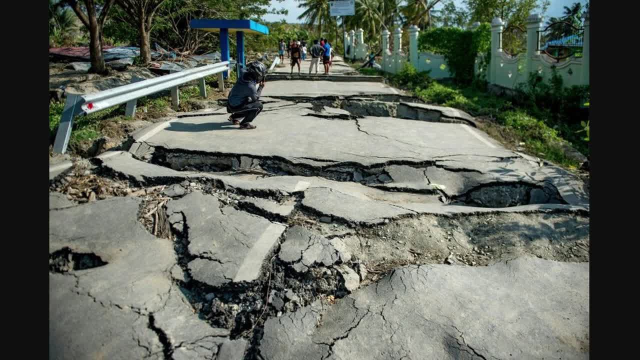 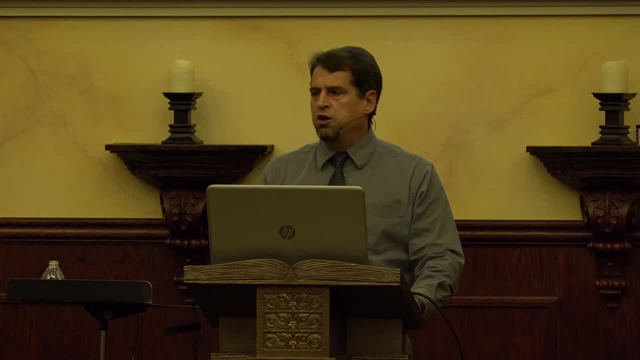 accomplish stratification of those materials. It doesn't take long periods of time and it doesn't take changing and depositional environments. Turbidity currents is another. Turbidity currents are underwater landslides, Here demonstrated in a laboratory flume, one of the 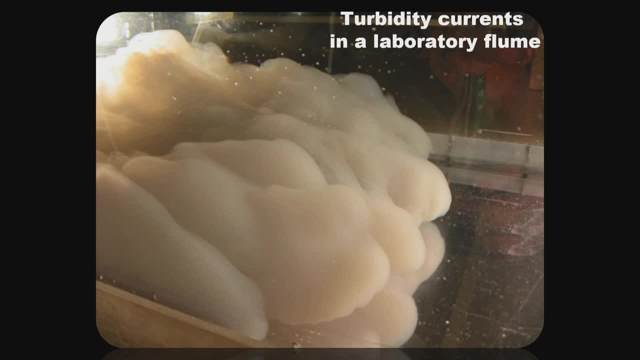 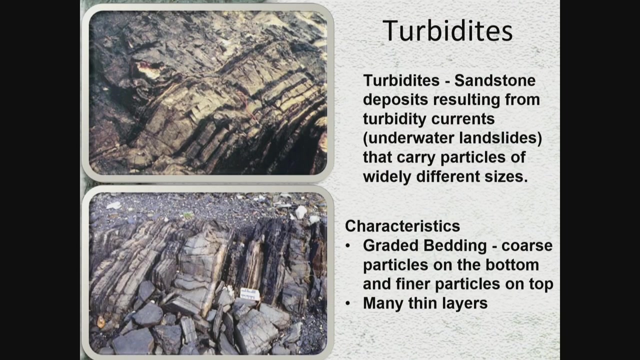 experimental apparatuses that is used to explore both sedimentation- how sedimentation occurs- as well as erosion. But sediments that form from turbidity currents form a particular type of sandstone called turbidites, And turbidites have a very particular characteristic that allow them to. 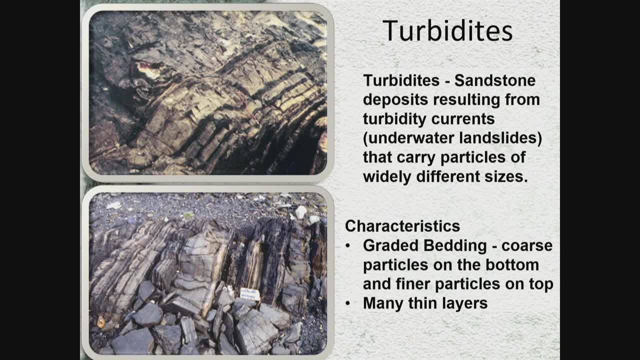 be identified as being due to a single flow. One of them is that they have a graded bedding Within a specific bed of sandstone. the particles go from bigger particles to smaller particles. There's a grading to the bedding so that they know it formed as a single bed. And you'll tend to find 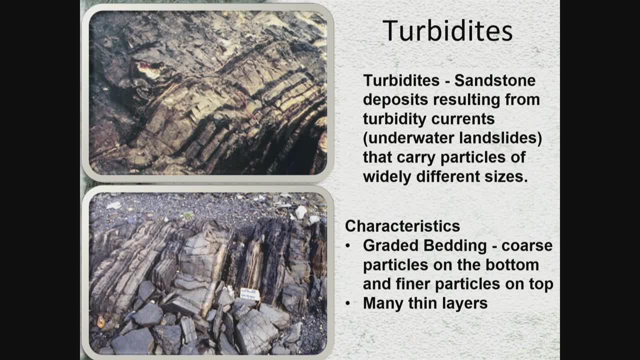 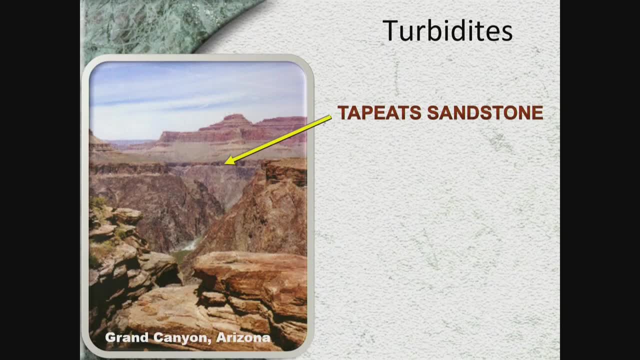 increasingly finer particles as you move upward, But these are just a couple of pictures of some turbidites found high up in the mountains. The sandstone layer identified here at the Grand Canyon is a turbidite, And this layer, called the Tapeats Sandstone, ranges in thickness from 125 to 325 feet thick. 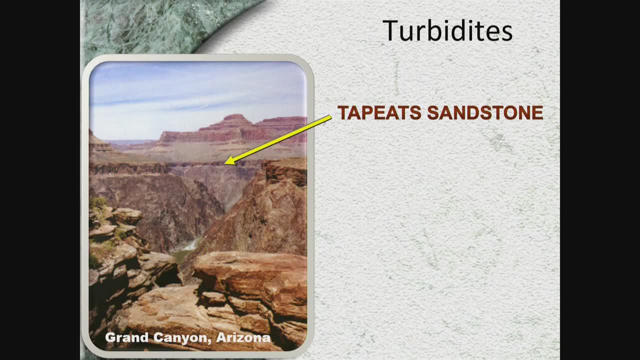 And it's the smallest: It's 125 feet thick. Now imagine the underwater landslide able to lay down a posa that's 125 feet thick. Geologists have concluded that the Tapeats Sandstone was due to a series of underwater flows of sand racing along at upwards of 90 miles per hour. 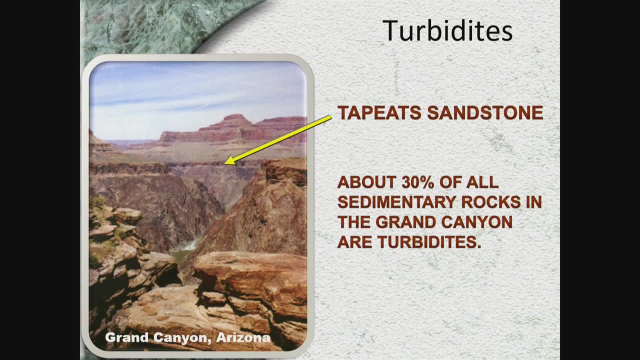 A devastating flow comprises a very highly energetic event that must have been caused by even a greater causal event. Scientists in fact estimate that about 30 percent of all the sedimentary rocks exposed at the Grand Canyon might in fact be turbidites. 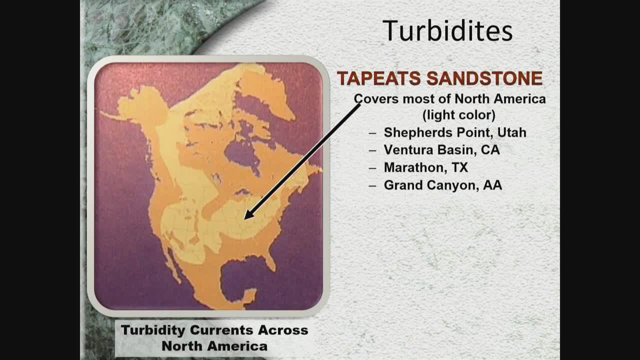 This map of the Tapeats Sandstone locations across North America, based on some oil well drilling information, illustrates the extent of this deposit covering most of North America at the base of the Tapeats Sandstone. It's noteworthy that at the base of the Tapeats Sandstone, 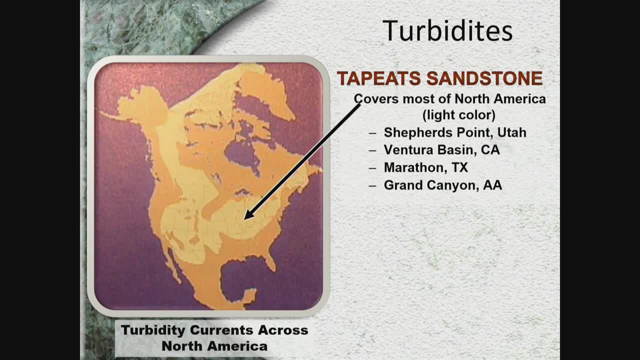 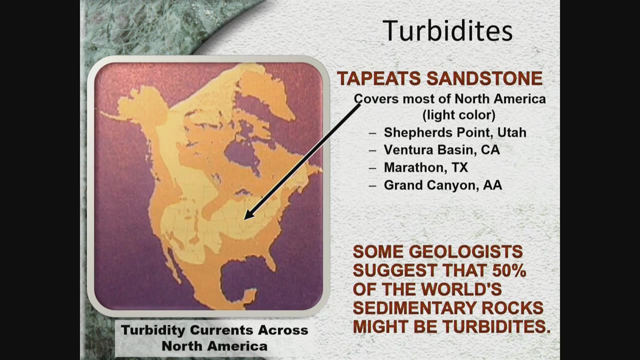 layer is an incredibly flat erosional surface from which all previously deposited material had been eroding away, leaving a very flat surface on which the Tapeats Sandstone was deposited, And today some geologists estimate that as many as 50 percent of the world's sedimentary 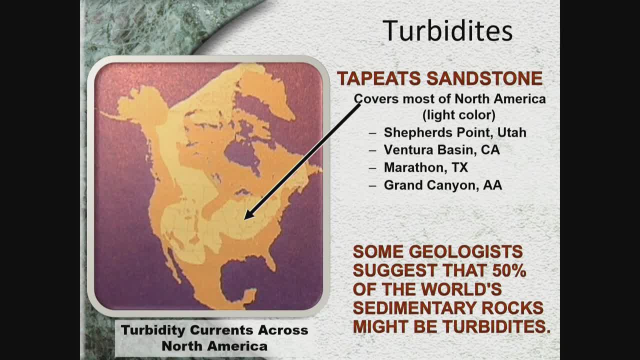 rocks might, in fact, be turbidites, which is just what we would expect if these sedimentary rocks were formed by a turbidite, And so, in fact, this is a very high-level, very high-level, global-scale flood that the vast majority of those deposits would have been through underwater. 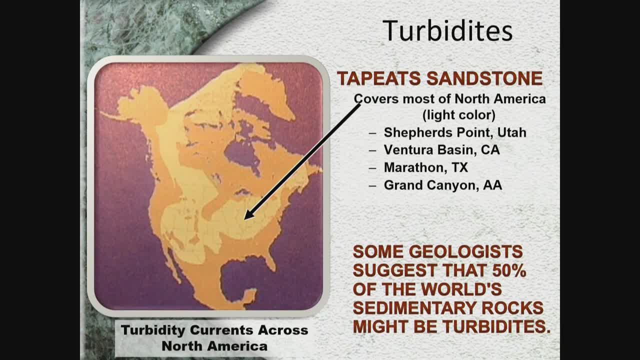 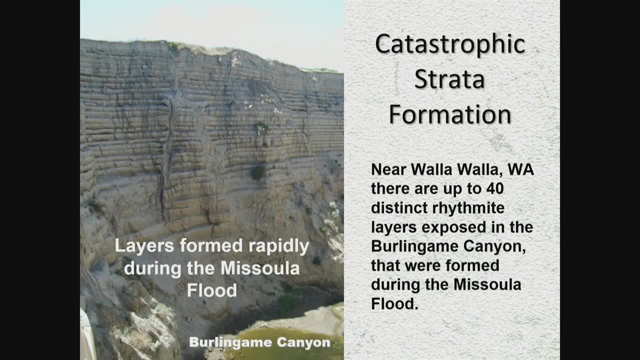 landslides. We can also point to a number of known geologic events that were able to produce strata rapidly. For example, these layers of rocks you see here near Walla Walla were formed during the Missoula Flood. That's a type of layering called a rhythmite deposit, believed to be due to rhythmic 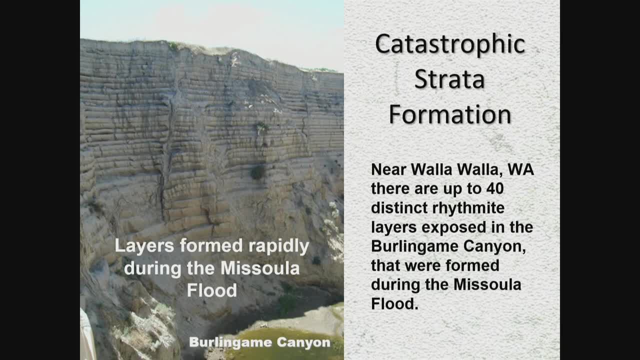 activities like the Ebb and Flood, And so, in fact, this is a very high-level, very high-level. the actions at a beach, The Ebb and Flow of a beach, can deposit rhythmic deposits or rhythmite deposits, And that's what these are believed to be due to: is some kind of rhythmic activity taking? 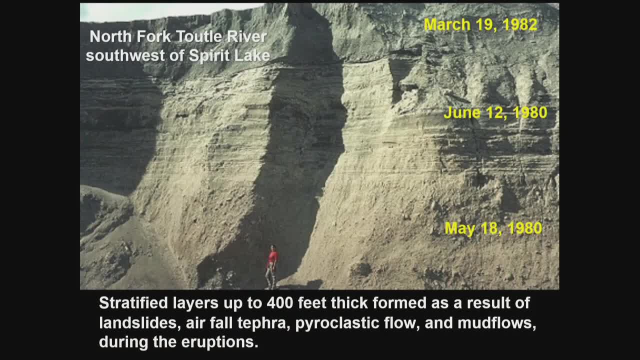 place during the Missoula Flood. The eruption of Mount St Helens, as I mentioned previously, also produced some significant strata. Here there are three separate geological units, all that were formed catastrophically during the initial eruption of Mount St Helens and subsequent mud flows. 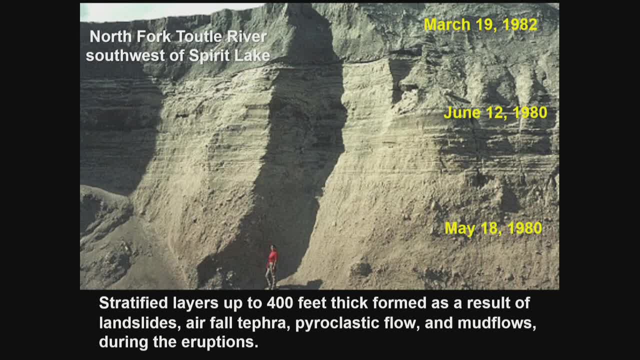 The bottom one is the Ebb and Flood, which is a very high-level. very high-level layer from May 18, 1980, is what's called airfall tephra material, That's from the afternoon of the initial eruption. The middle layer was created by what's called a pyroclastic flow, basically a. 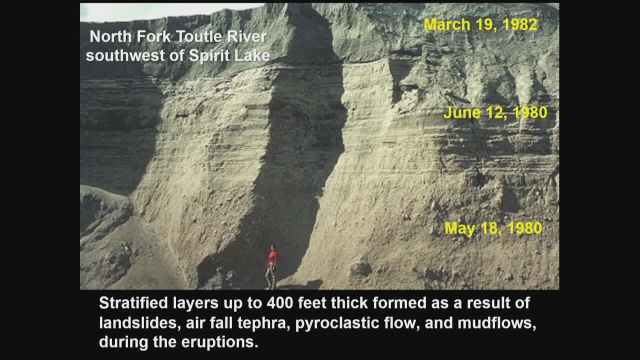 landslide during a volcanic eruption- Very, very hot, very, very nasty. And then the upper layer formed two years later during a mud flow that deposited a layer on the top. The middle layer in particular is very interesting. The Ebb and Flood layer is a very high-level, very high-level. 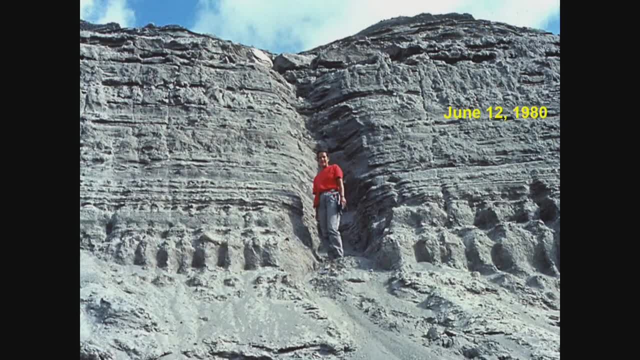 interesting. Look at it here And remember that we're taught in geology that individual layers like this take a long time period to form. But here you see a deposit more than 25 feet in thickness, containing upwards of 100 separate layers that accumulated in just one day during a pyroclastic. 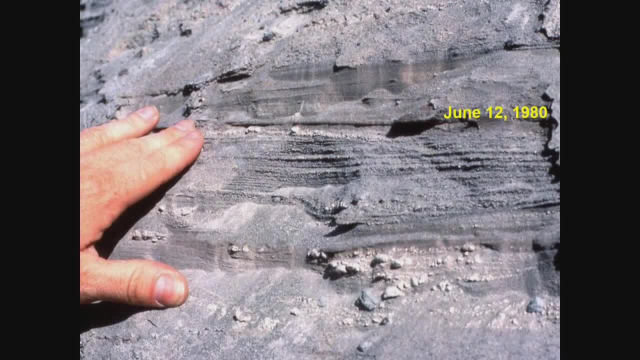 flow, which again just is a type of landslide Fine lamina, only a millimeter in thickness to some more than a meter high, formed in just a few seconds, And here you see a deposit of more than 20 seconds. Another powerful piece of evidence that points to a global catastrophe resulting in 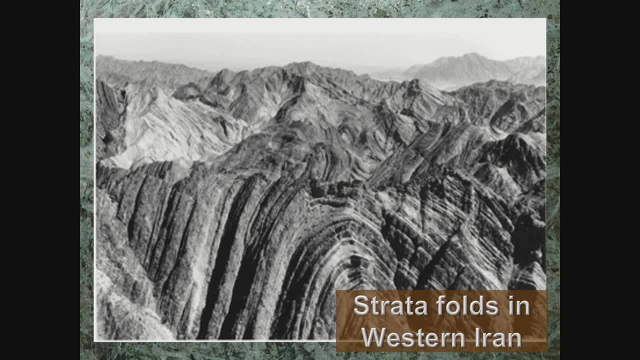 these strata are the fact that in many mountainous areas we can see these rock layers that are thousands of feet thick, that have been bent and folded without fracturing. How can that happen? You've got to ask if they were laid down separately over millions of years and had 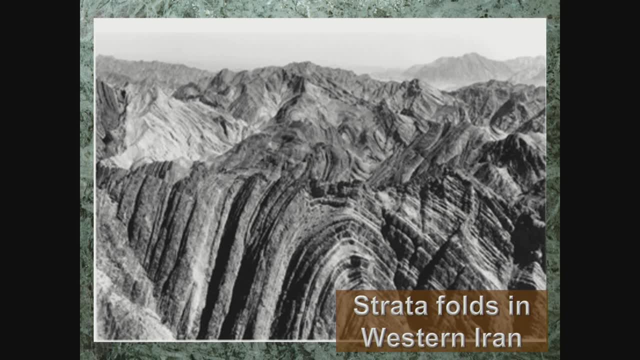 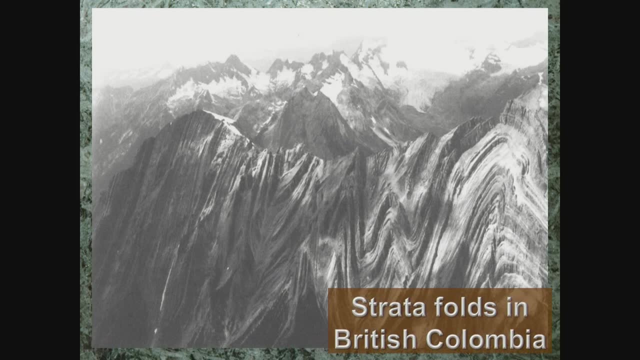 already hardened. These layers that you see here are in the Zagros Mountains along the southwest coast of Iran. These shown here are from the Sullivan River area in southern British Columbia. But again, hardened rock layers are brittle And in particular, limestone is hardened by. 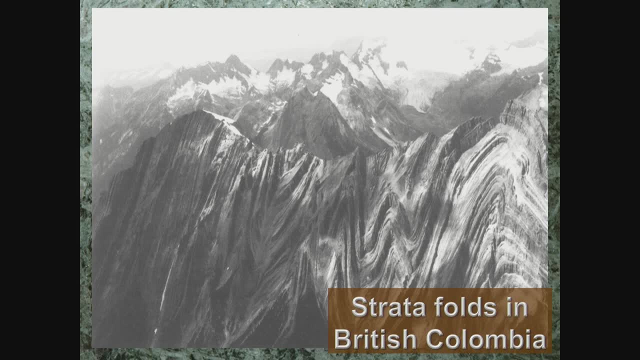 mineral deposits, calcium carbonate, which is again what we use to harden concrete. So try bending a slab of concrete like this to see what happens. But again, if concrete is still wet and pliable, you can bend it. The same principle applies to sedimentary rock layers. 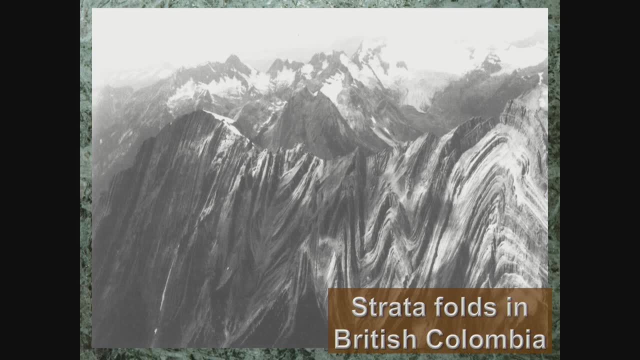 They can be bent and folded soon after the sediment. The cement has been deposited, before the cement hardens, but not brittle rocks. You can't get brittle rocks, ancient rocks like this, to fold in this way. Polystrate fossils are another example. 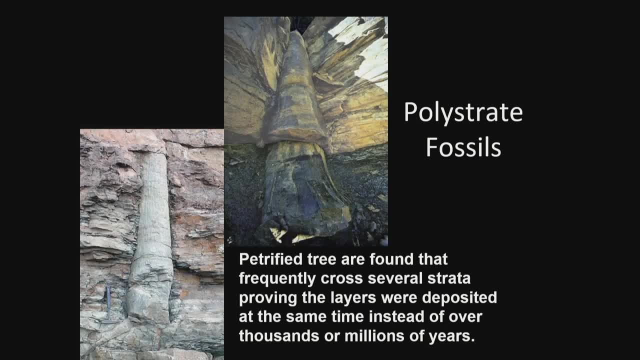 of rapid strata formation. Many polystrate trees- trees that pass through multiple layers of strata- have been found that span multiple layers, And it's just not possible for fossils to be buried gradually over many thousands of years. So it's not possible for fossils to be buried gradually over. 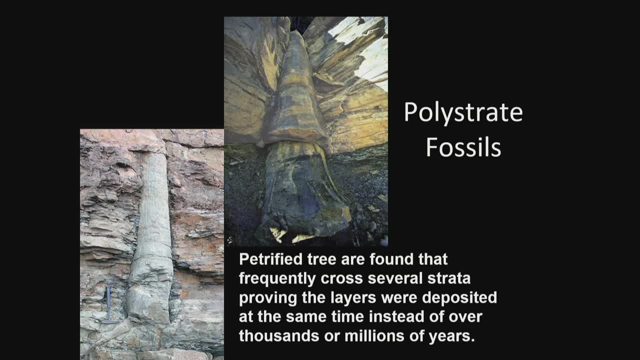 many thousands of years And it's just not possible for fossils to be buried gradually over many thousands of years. So it's not possible for fossils to be buried gradually over many thousands or hundreds of thousands of years due to the speed of decomposition During slow uniformitarian-type. 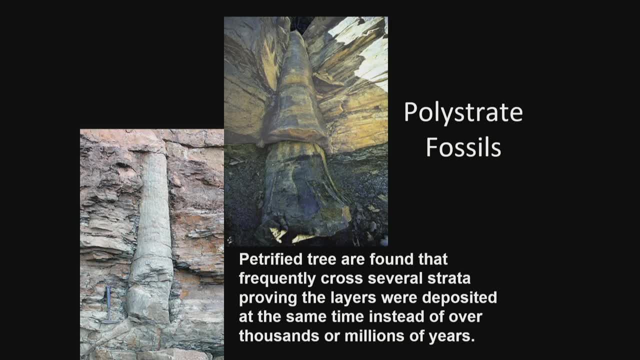 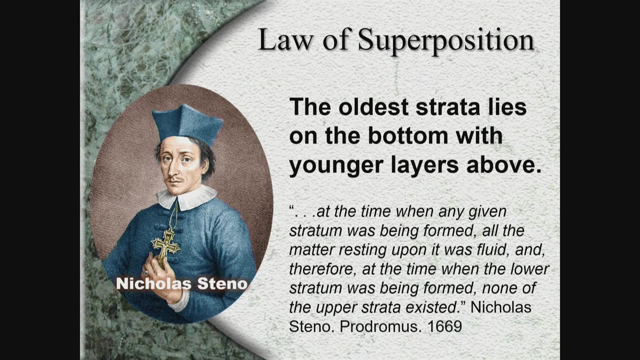 burial, the top part of the tree would rot away before it could be protected by sediments. Polystrate trees like these point to one thing, and that's the certainty of rapid burial. Now let's revisit the law of superposition just one more time. 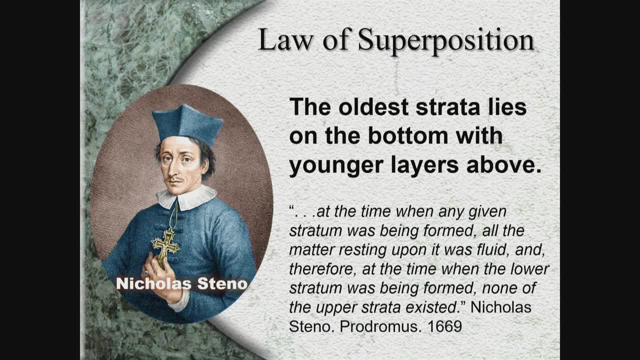 and evaluate it against some experimental results. Now again, this law states that the oldest strata lies on the bottom, with younger layers above. But this law of stratigraphy has been shown experimentally to not be true in certain types of depositional environments, such as when sediments are flowing. 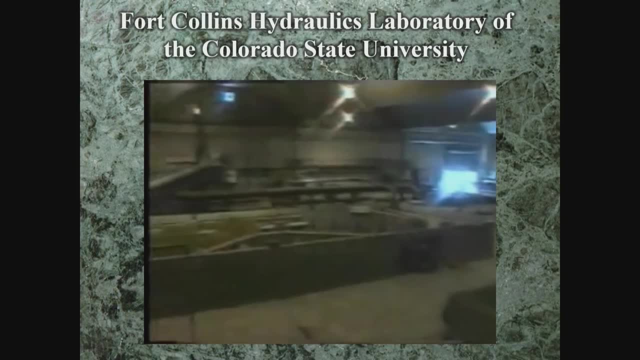 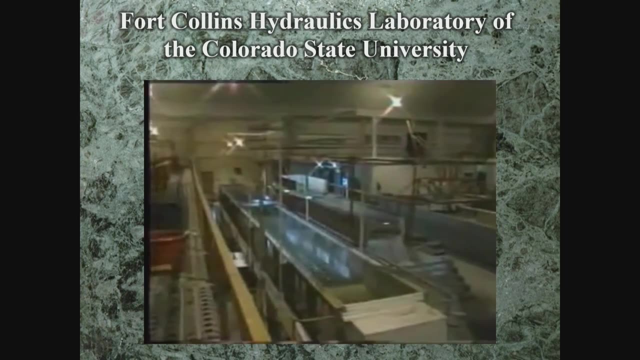 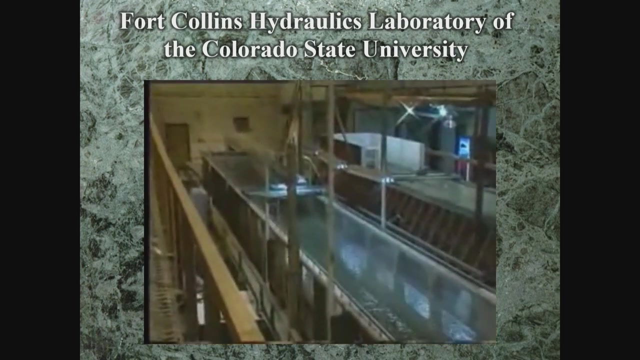 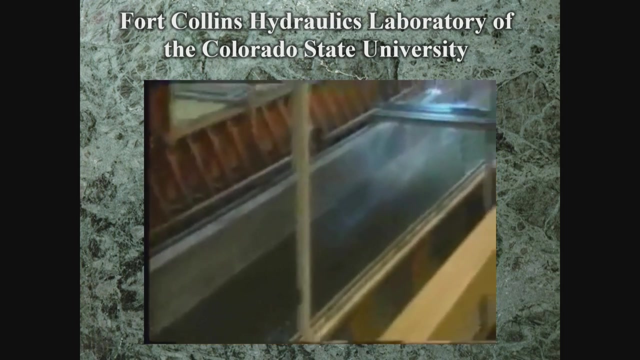 Now, laboratory flumes like the one I showed you previously are used to simulate erosion and deposition environments and thus explore the factors that are influencing these processes, including strata formation. Large-scale flume experiments were conducted at the Fort Collins Hydrologic Laboratory at Colorado State University with Professor of Hydraulics and Sedimentology. 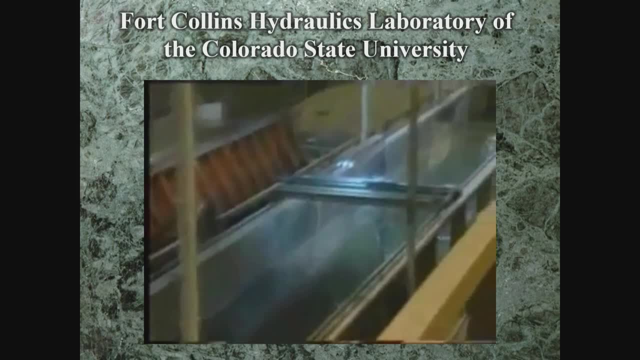 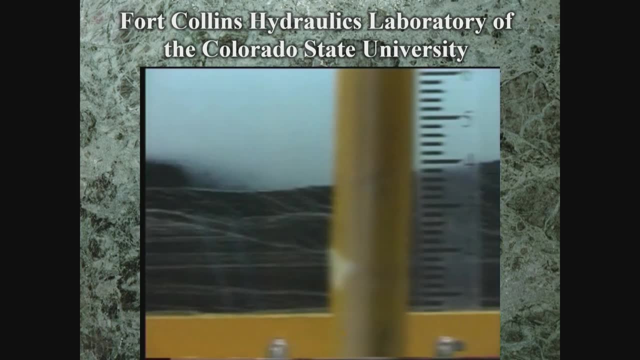 Pierre Julien, and the work on this was published in the Journal of Creation back in April of 1988.. In these laboratory flumes they observed stratified sediments forming in minutes to hours under simulated sediments. So in this laboratory flumes they observed stratified sediments forming. 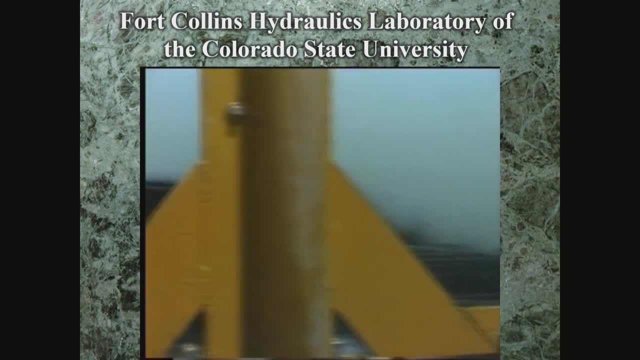 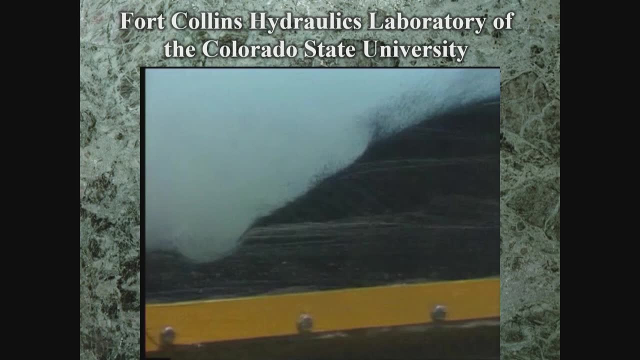 under simulated conditions, Heterogeneous mixtures of particles of different sizes and densities were used to determine how these particles would behave in various depositional environments. What they did was they mixed sand, limestone and coal that had different colors to help with the visualization, and what it demonstrated was that both fine lamina and thick beds 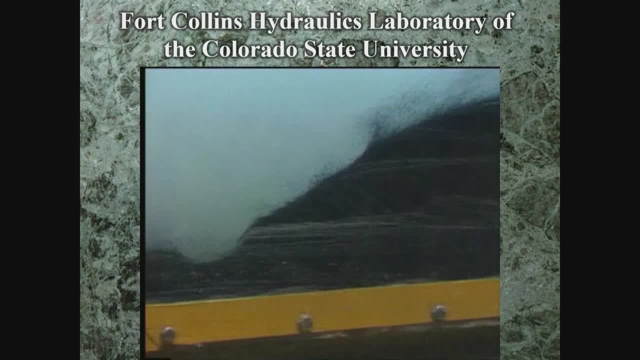 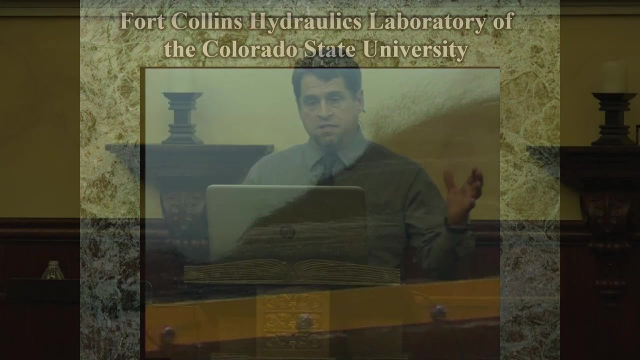 would form during lateral motion. Fine particles would fall between coarse particles and the coarse particles would roll across the finer particles, causing different layers to form simultaneously. They didn't form sequentially, but these layers formed simultaneously as these sediments were flowing. And perhaps one thing that was most interesting about this: 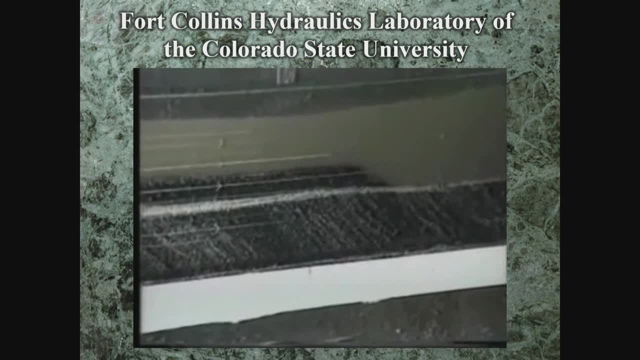 I don't know how well this video captures it, but what they found was, again, with the two particles that you see here, you have a darker sand mixed with coal, and then the white layer is the limestone that they mixed in there with it, And it was. 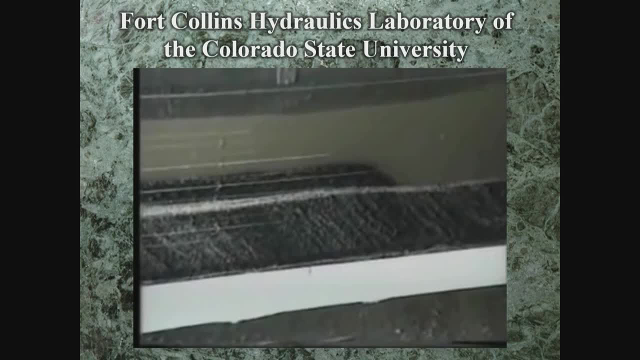 separate out into two layers. but what they? what would happen if they change the rate of the flow of the water? another pair of layers, another black and white pair of layers, would start forming on top of the previous pair if they change the rate of the flow. so if they increase the rate of the 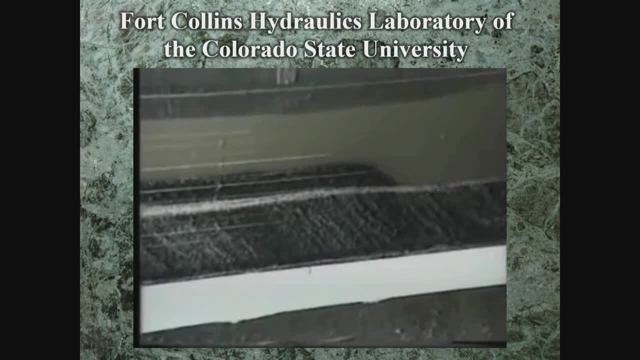 flow or decrease the rate of the flow, another pair of layers would start forming on top. and if they change the rate, again another pair of layers would start forming on top. but all of those pairs of layers would keep developing in a prograding manner every time they change the rate of the 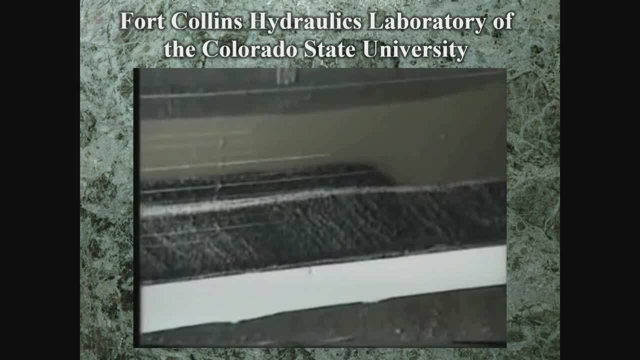 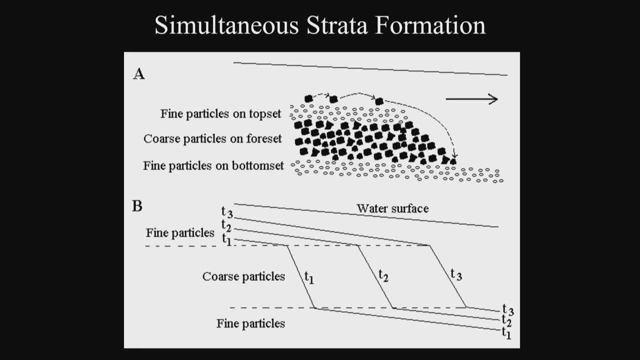 flow, another pair would start forming, and but all of them will continue to form the prograding manner. so what these experiments showed is that when sediments are flowing, the law of superposition just does not hold true. fine particles again would fall between coarse particles and the coarse. 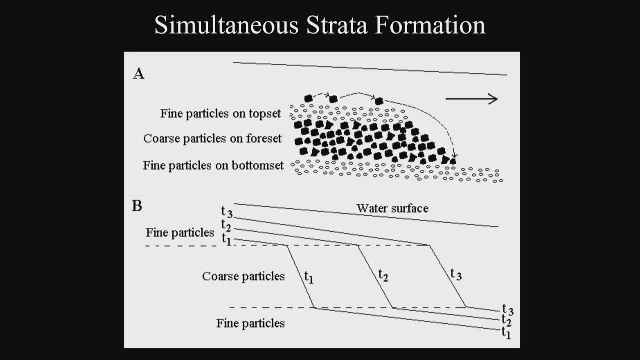 particles would roll across, the fine particles becoming embedded in the layer beneath. and, more importantly, as this diagram tries to show, the time sequence related to the flow of the water would continue to develop in a prograding manner every time they change the rate of the flow. the relationship of the strata is much less bottom to top, as is argued by. 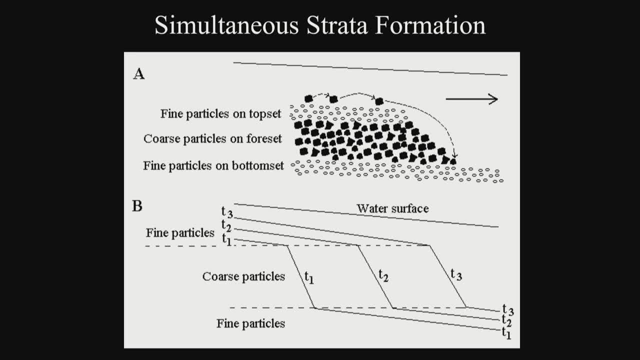 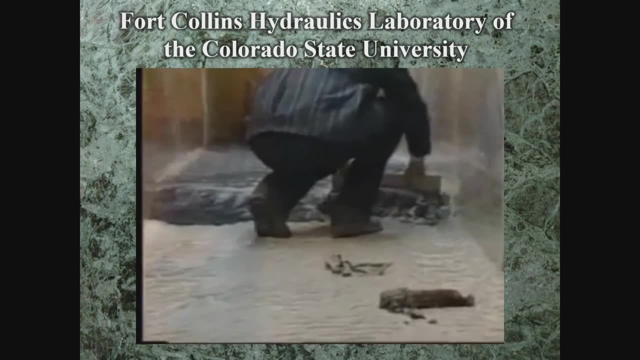 the law of superposition, but is instead more front to back in the direction of the flow, with the newer sediments being on the forward end of the flow, not on the top, but in the forward end. it's very interesting. a cross section of the sediments from these experiments reveals the significance of the 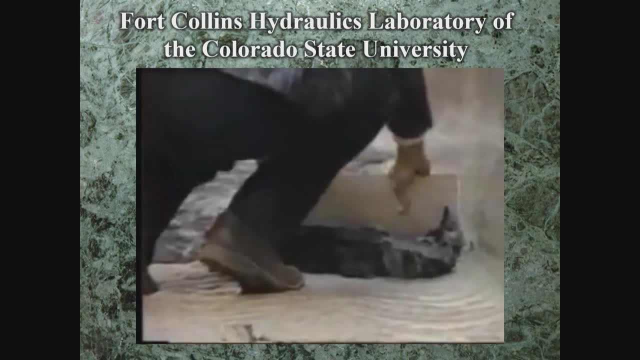 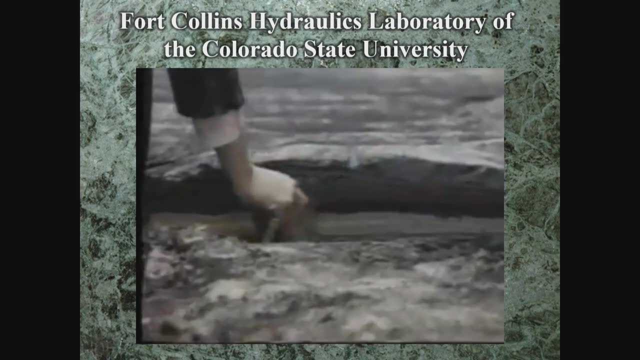 types of layers that are produced by laterally flowing sediment. watch here as this researcher cuts the sediments from the flow of the water and the flow of the water and the flow of the sediments through the accumulated sediments to reveal strata that formed rapidly again. both fine. 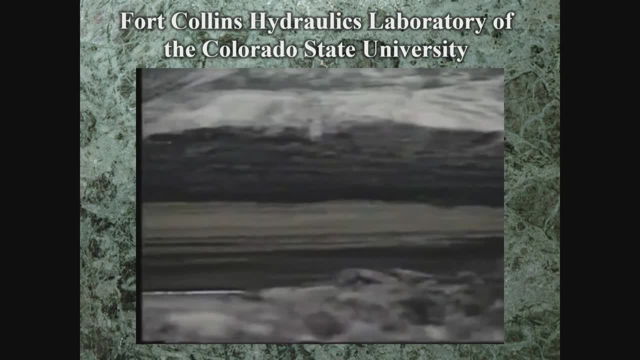 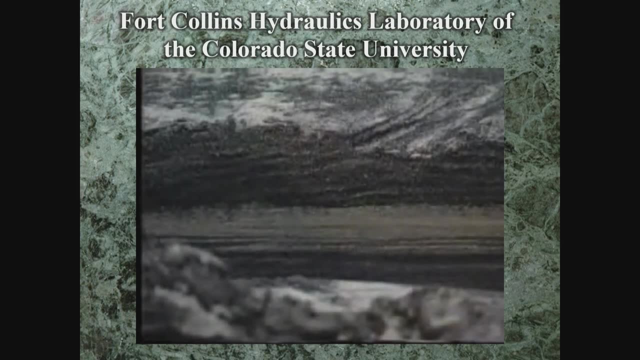 lamina and thick beds of sediments. you can see there, including a thick layer of white limestone. that's limestone. that white layer is white limestone strata simply doesn't require changes in depositional environment. remember, they argue that limestone formed when the oceans inundated the continents, depositing the. you know these, uh, these fragments of the exoskeleton, fragments of a? 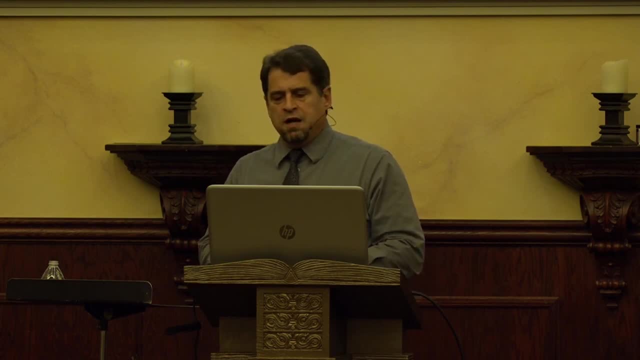 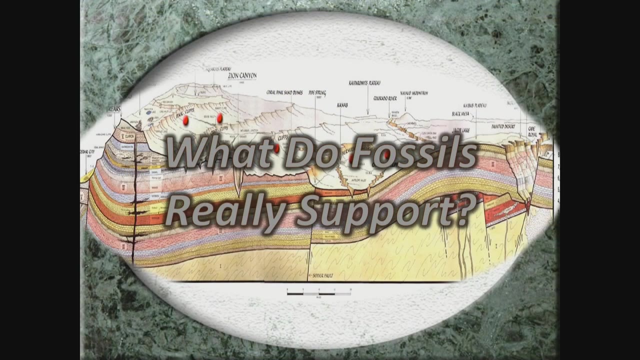 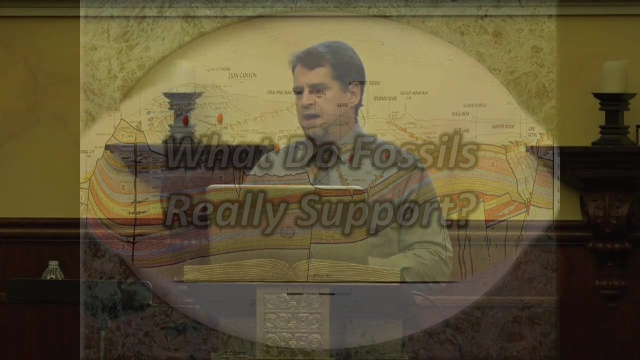 shellfish. so let me kind of change subjects just a little bit and ask this question: what do fossils really show? i believe that the geology is clear that what you're looking at is the result of a major, catastrophic flood. but again, fossils are used by evolutionists today as their main supporting. 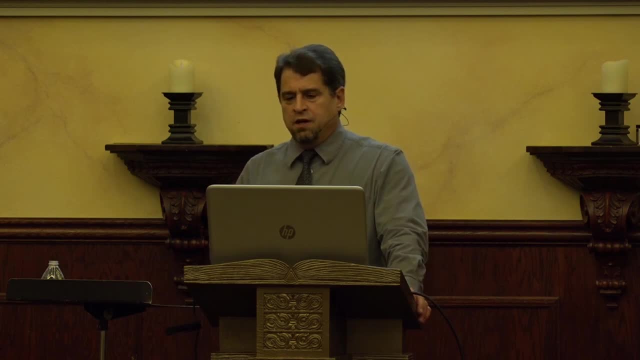 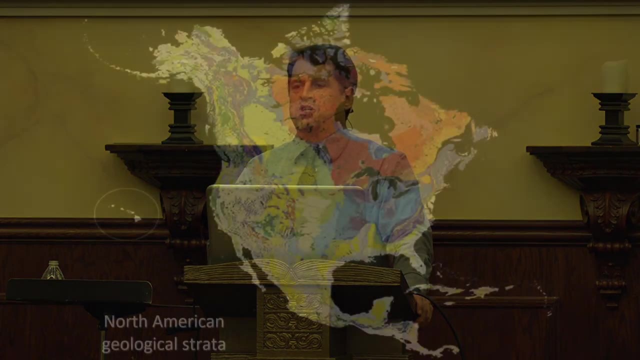 evidence. but what is? what do fossils really show? well, sedimentary rocks blanket the entire earth again, except where uplift and erosion has removed this layer. the earth is not a shellfish, it's a covered in monumental layers of sedimentary rock, fossil beds that are thousands of feet thick in. 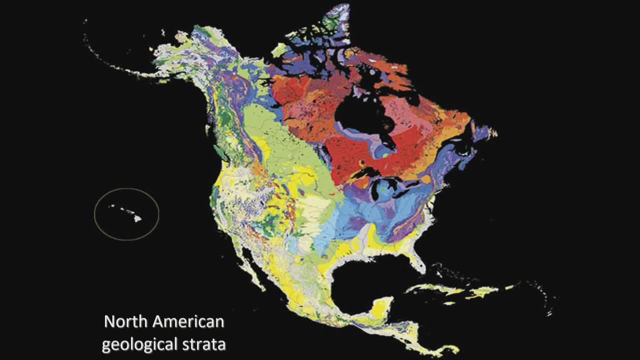 some places, however, we do not see sediments forming like that. today. we see sediments forming in little local deposits, such as when when a river lays down its uh its load, and forming a river delta. when a river slows, the sediments that it's carrying will be deposited when it enters a larger body of. 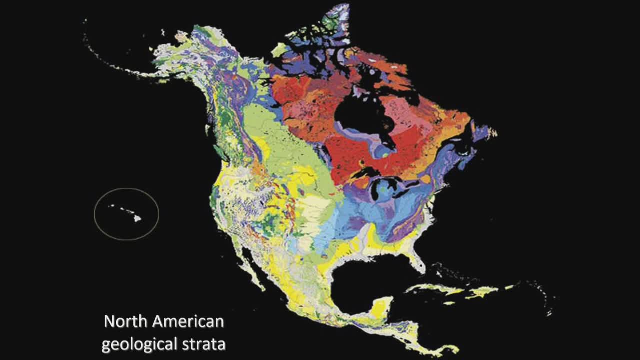 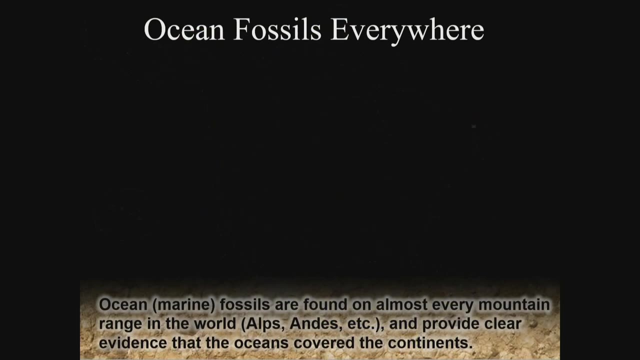 water producing a river delta. we don't see sediments forming like this today. so if the present is truly the key to the past, as lyle argued, our observations only find local deposits of sediments forming. the fossil records suggest a worldwide catastrophic depositional event. we find 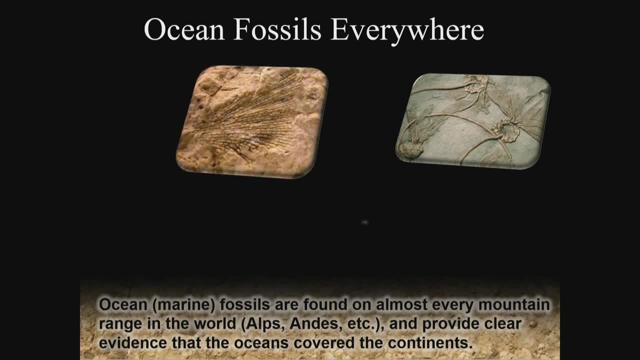 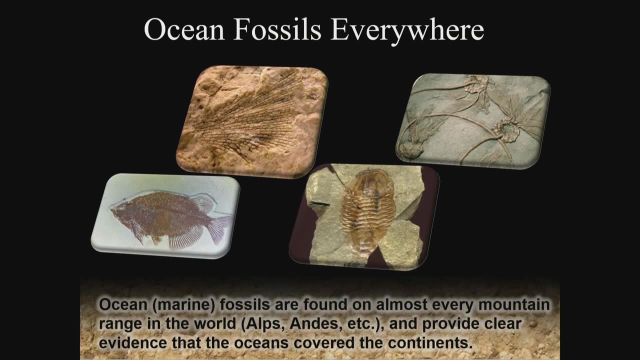 ocean fossils on the tops of every mountain train in the world. we should find ocean fossils everywhere, not just on the top of every mountain chain, but in every single layer of the fossil record we find abundant ocean fossils. this proves that the ocean ended, inundated the continent. 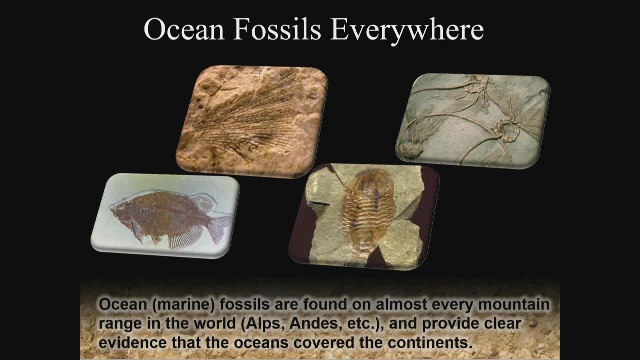 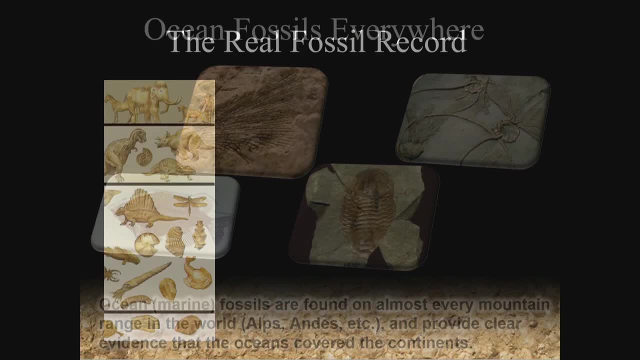 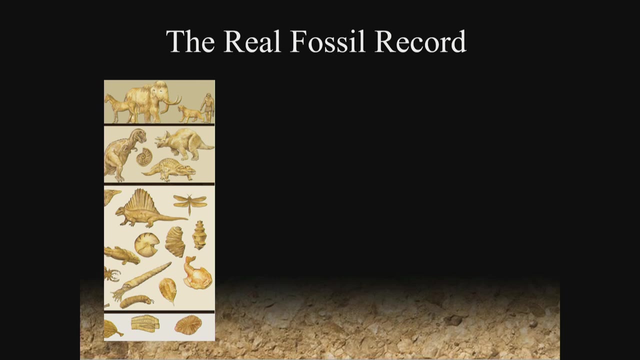 but that it didn't just uh do so once during geologic history. we can find ocean fossils in every single period of the geological column, the uh. unlike this diagram that you typically see to illustrate the fossil evidence for evolution, what the fossil record truly is is a record of ocean. 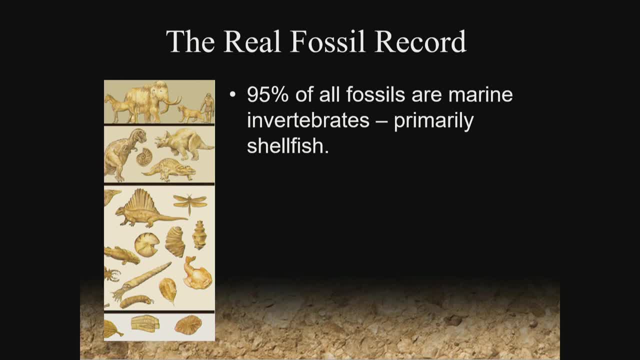 deposits. it's a. i mean, it's just full of clams. you could. you could call the fossil record a record of clams, because it's blue and what it seemed like most of fossil record is, but it's not. 95 of all fossils in the fossil record are marine invertebrates, primarily shellfish. 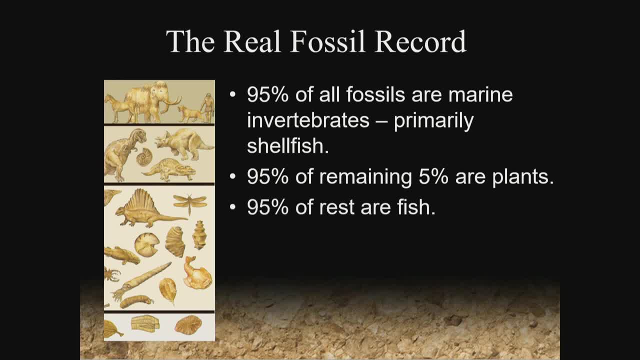 95 of the remaining five percent are plants, 95 of the rest are fish. most of the rest are insects. much less than one percent of the fossils in the fossil record are, in fact, land vertebrates. it's a record of a monumental global scale flood, not the history of life on earth over hundreds. 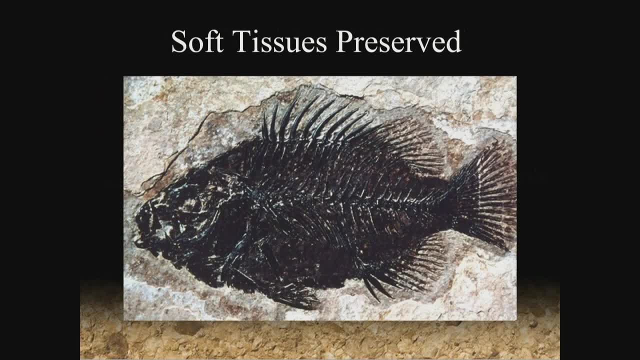 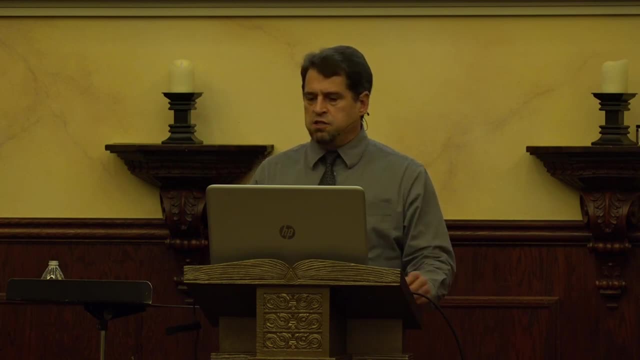 of millions of years. that's what it is. there's lots of evidence from the fossil record to speak to this event. we find fossils of with soft tissues. soft tissues just should not survive any kind of fossilization process due to the rapid speed of decomposition. but we find lots and lots. 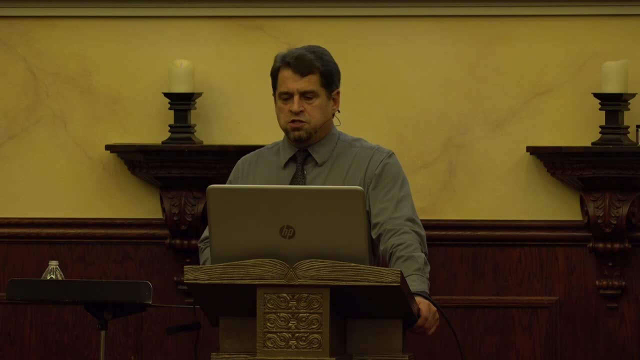 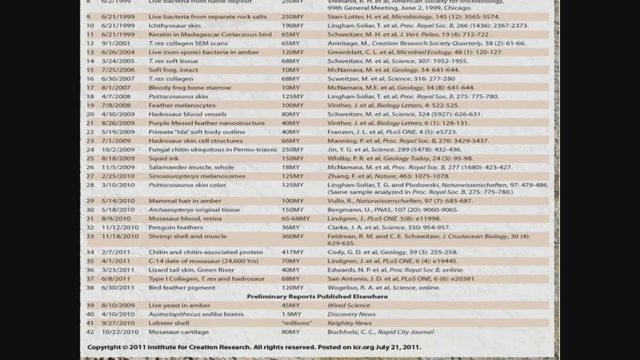 of soft tissues um fleshy parts, skin, cartilage. we find unborn fetuses. stomach contents have been used to identify what fossils have eaten. the number of soft tissues that have been discovered at this point in time is just enormous, and ranges beyond 100 million years. we in fact find dinosaur bones that aren't even mineralized. this is a dinosaur. 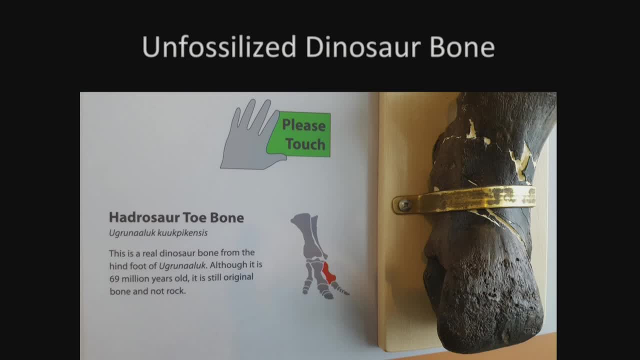 bone that's on exhibit in uh at the university of alaska in fairbanks. that's real bone. it's not rock, it's real dinosaur bone. the the on the. on the caption. it says: this is real dinosaur bone from the hind foot of a, a type of hadrosaur. although it is 69 million years old, it is still original. 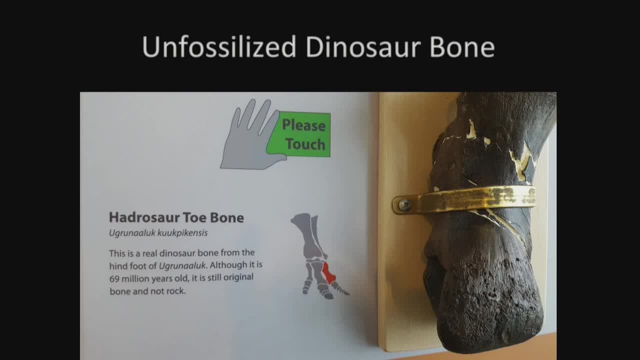 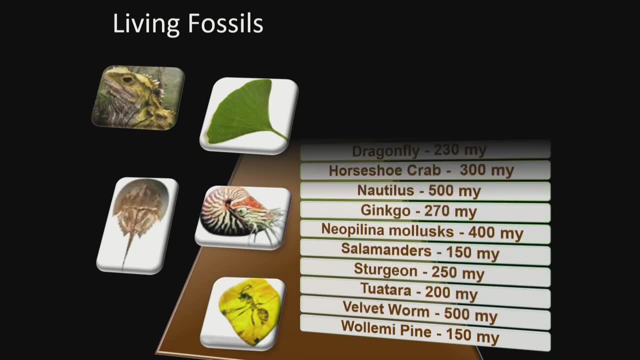 bone and not rock. it's not 69 million years old. it was an animal bone. it was a dinosaur bone that died during the global flood, a recent global scale catastrophe. we also find that that the vast majority of the fossils could be categorized this way, but we find lots and lots of fossils that are 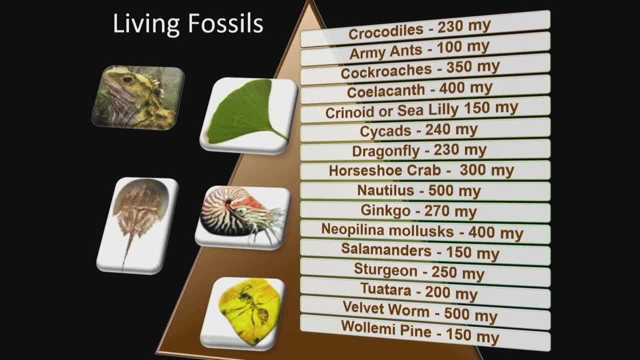 identical to living animals, identical plants and animals. both. lots and lots of fossils are categorized as living fossils because they're identical to animals we find alive today. life on earth hasn't changed through time. it's they've just interpreted the fossil record incorrectly. we find the same animals alive today that we find in the fossil record, and we find fossils in massive 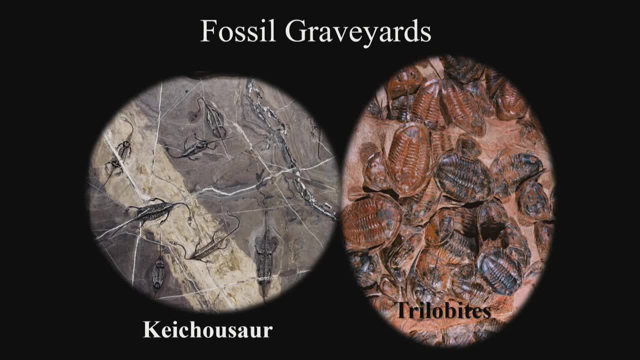 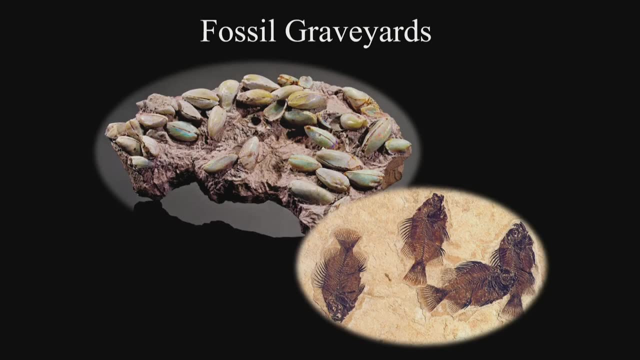 graveyards. this is just a typical characteristic of the fossil record that organisms are often found in mass. whole communities of organisms are found buried together. i mentioned the morrison formation previously, where you find the dinosaur national monument. thousands of dinosaurs are found buried together in one massive formation up in uh. up in canada they found a 10 000 centrist. 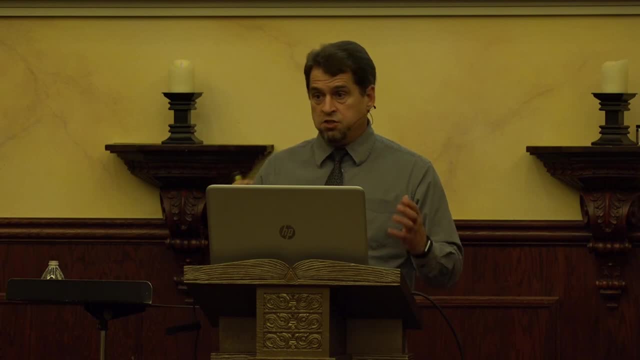 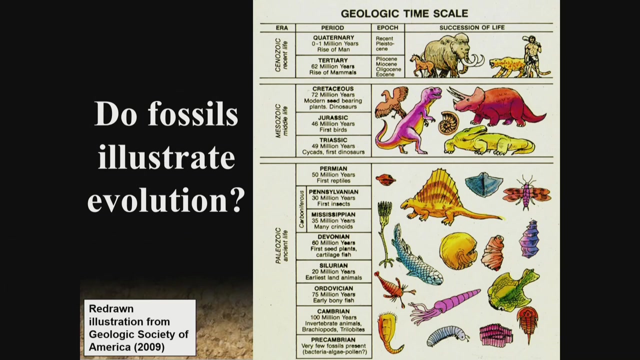 sources buried in one formation, a type of a ceratops dinosaur. this is such a general characteristic of the fossil record. but again, fossils are used to prove evolution. they use these diagrams and try to argue that the fossils show that life on earth has changed over time. 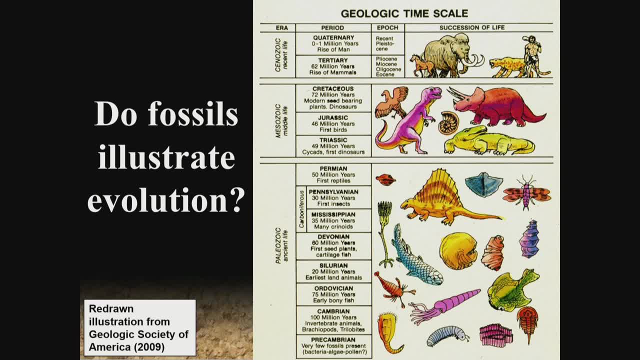 from simple to complex forms, we would acknowledge that there are different fossils found in different layers. again, our interpretation of this is that what you're looking at is this just the destruction of successive habitats during the flood. the fact that there are different fossils in different layers, though, doesn't prove evolution, what and what they must be able to show through. 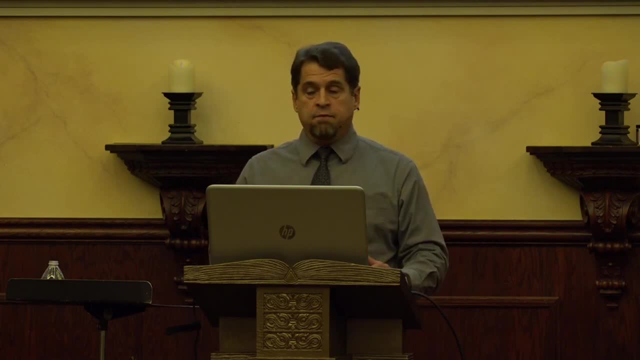 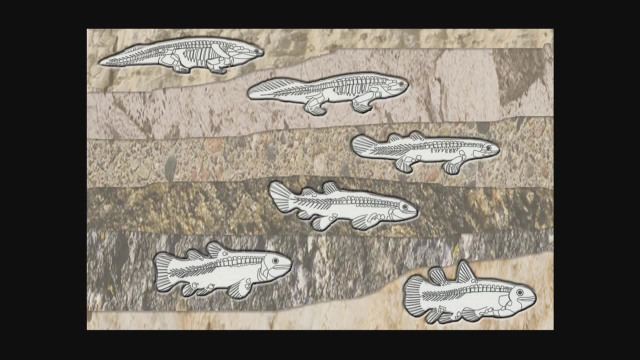 the fossil record is that an organism changed through time by way of fossil forms. can they show an organism that changes slowly and gradually from one form into another by way of fossil forms? answer: this is no. now i want you to understand something that, uh, darwin himself did not. 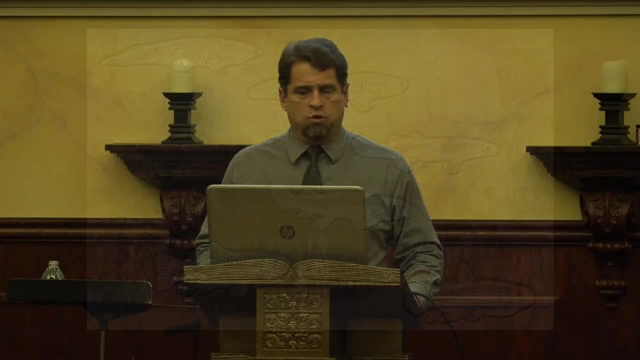 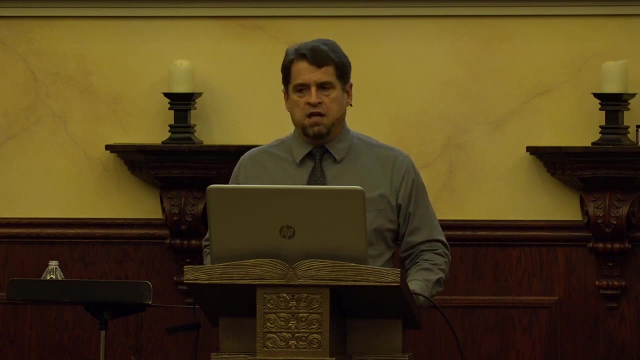 wasn't, didn't invent evolution. there are many people during darwin's time who believed in evolution. um he, though, proposed something a little different, he himself. he was himself a- uh, an accomplished breeder of pigeons, and was well familiar with how different breeds of animals 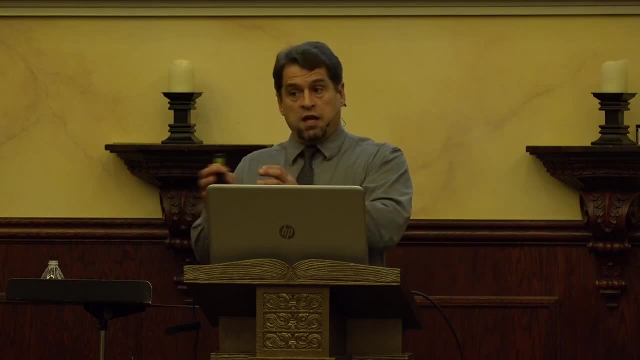 had been created slowly and gradually through selective breeding processes, and he argued that the same process was happening in nature and if that same process was responsible for the changing of animals and the changing of the environment, it was a process that was happening in nature and it was a process that was happening in nature. and it was a process that was happening in nature. 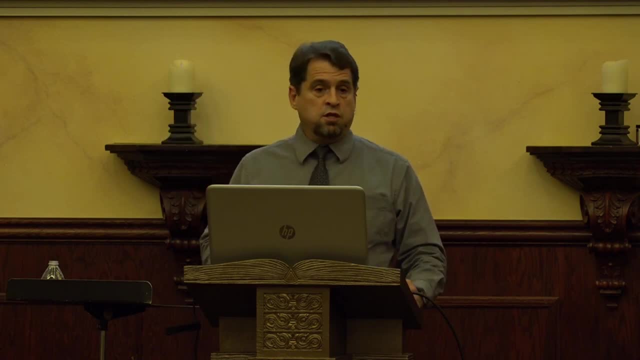 animals in nature. then it was a slow and gradual process. most of the evolutions of darwin's day held to a process called saltation. they believe that evolution occurred in rapid jumps because when they looked around at living populations they saw distinct groups. you got a whole bunch of 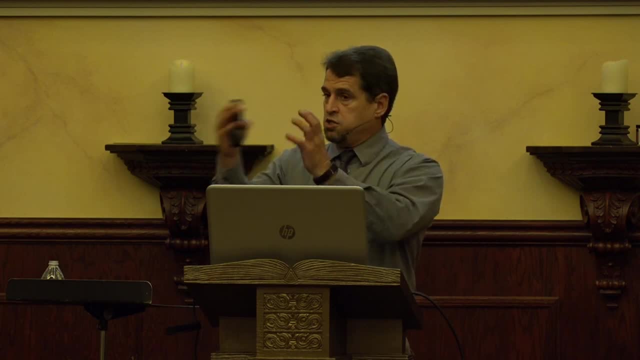 turtles and a whole bunch of lizards and a whole bunch of snakes, but you don't see turtles and that gradually change into rept, into lizards, and then lizards that gradually change in reptiles. for all the animals you can think of, there are distinct groups of animals, and at least of the. 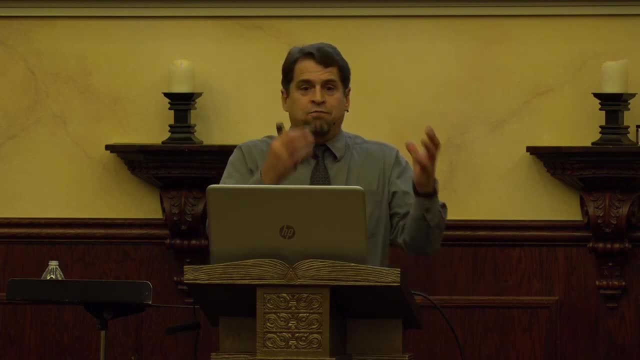 fossils they knew of in darwin's time. they also just knew of those distinct groups. but darwin assumed that other animals had lived, that these distinct groups were just due to extinctions. and he predicted- and it actually gives a carefully worded apology in his 1859 book- 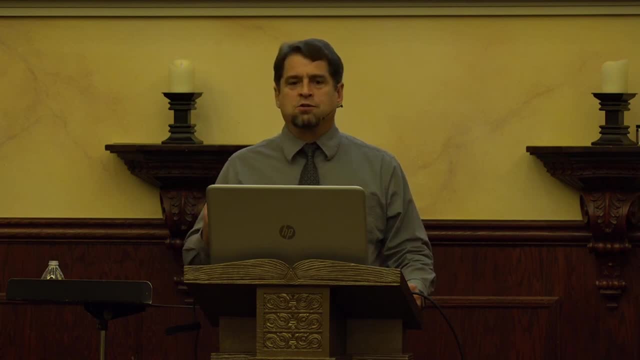 on the origin of species, that he can't point to fossils to prove that they were distinct groups, this theory that life slowly and gradually evolves through this natural selection process. but he argued that he predicted that the fossils would eventually be found. he acknowledged that groups of animals exist in living populations but he- uh, he argued that this slow and gradual 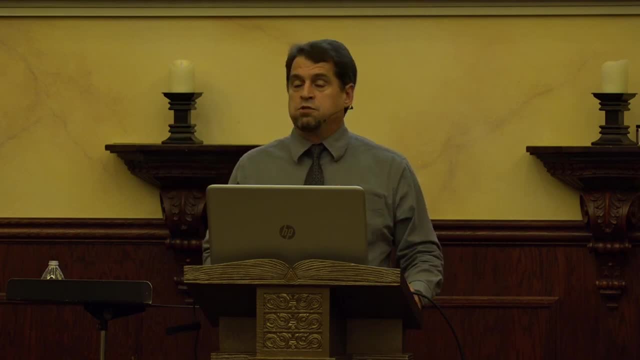 process would have produced animals. that did produce animals in the past. they're just extinct today. but he predicted they would be found in the fossil record, and uh so. but here we are, 150 years later, and they're no better able to illustrate this process. the fact that darwin 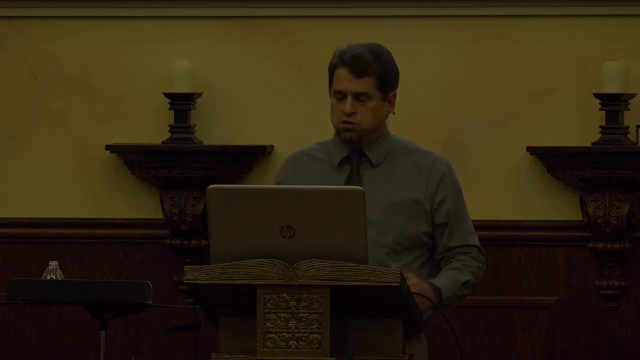 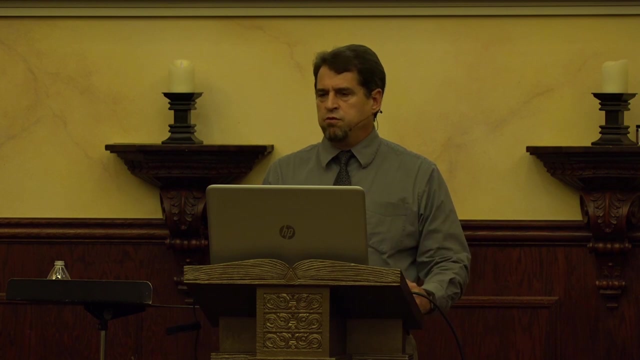 couldn't point to fossils gave him great concerns. so what we see are these distinct groups and and since darwin published origin species and predicted that fossils would eventually be found, literally here we are, 150 years later, and they're no better able to fill in these gaps. 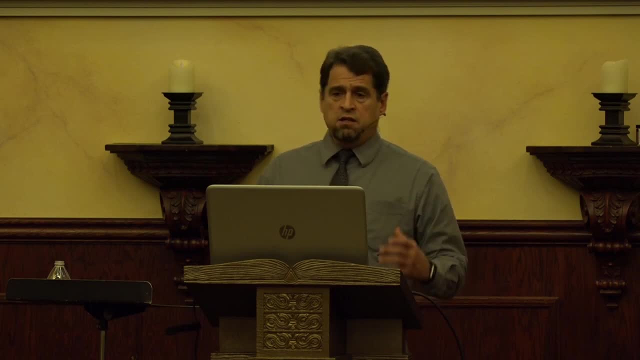 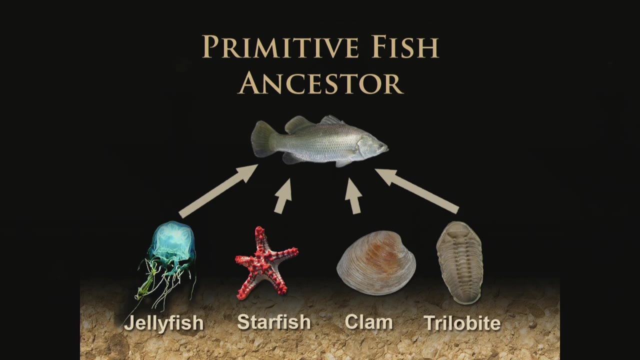 these missing links are real and they're monumental. to illustrate how significant this, this is, i mean, i've just given you four examples of. there are multiple invertebrate phyla like the, the nidarians, represented here by the jellyfish, the echinoderms, like is your starfish, or your mollusks, represented by the clams, or your arthropods. 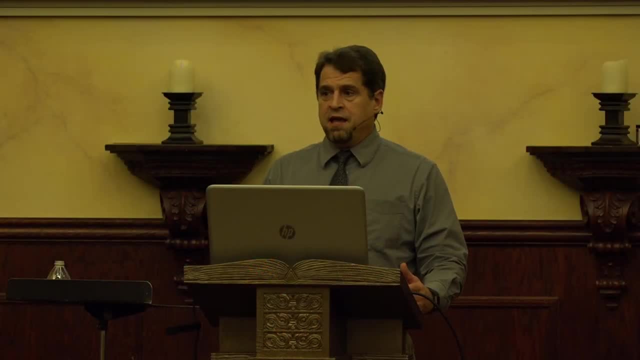 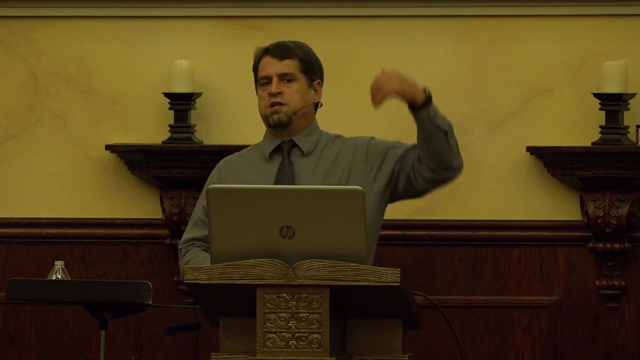 there are multiple invertebrate phyla that are about as distinct from each other as you can possibly be, and there's just no indication what evolved into the first nidarian. there's no animal that that is in the fossil record that was in the process of evolving into a nidarian or into an. 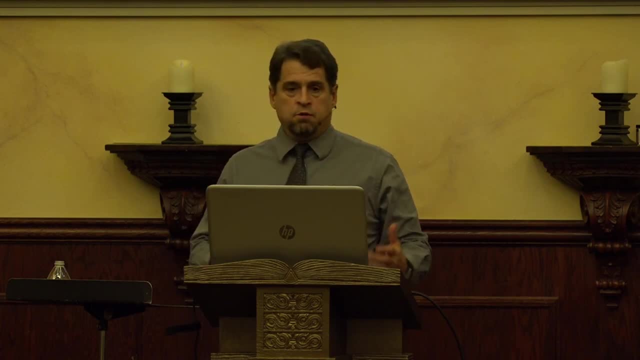 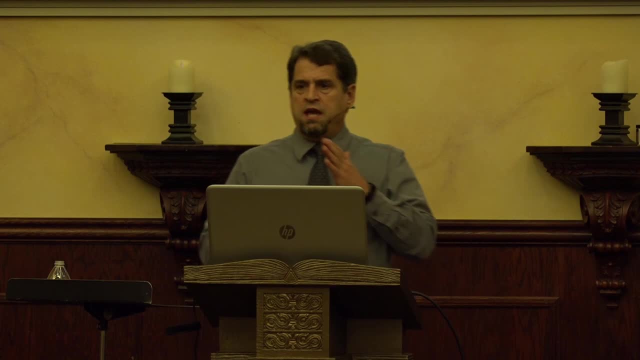 the ones we still find alive today, And there's just no indication. what did a Cnidarian evolved into a Cynoderm and a Cynoderm mollusk? If Darwin's theory is true, there should be an imperceptible blend of one type as it gradually evolved into another type and another type, and 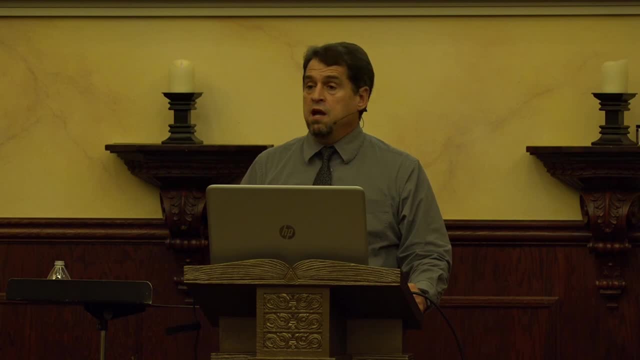 another type, But there is just distinct from one another as they can possibly be. The gaps between organisms are real and they are massive. We're talking about massive gaps in the fossil records And that evolutionists don't acknowledge this is very troubling because it's a very stark 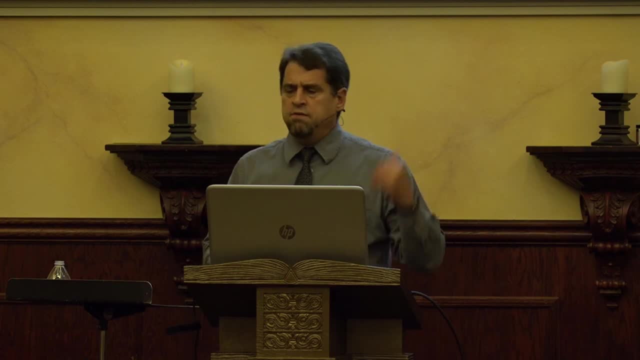 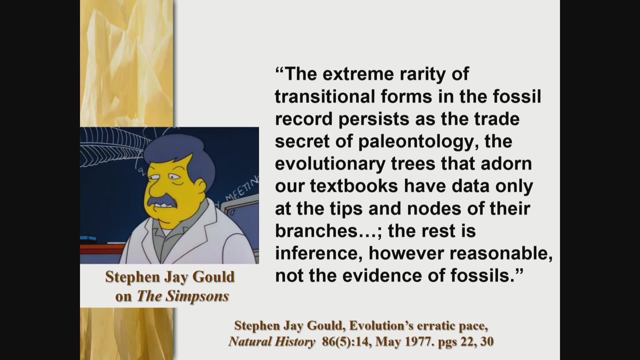 fact of paleontology. Stephen Jay Gould, arguably, is one of the most famous paleontologists of our day. I say this because he was featured on an episode of The Simpsons. you know, and I think that's acclaimed fame for any scientist, if you're on the episode of The Simpsons had a cameo on the episode of. 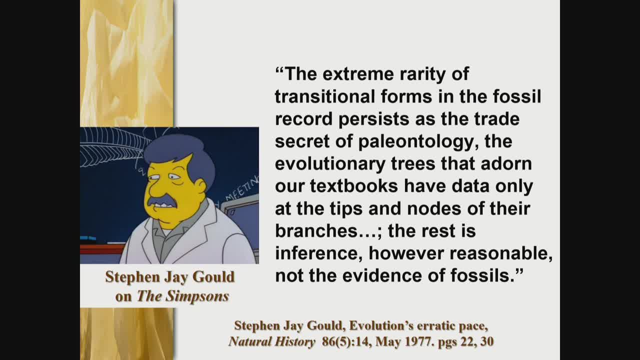 The Simpsons. Anyway, Stephen Jay Gould said that the extreme rarity of transitional forms in the fossil record persists as a trade secret of paleontology. The evolutionary trees that adorn our textbooks, he says, have data only at the tips and nodes of their branches. The rest is inference. 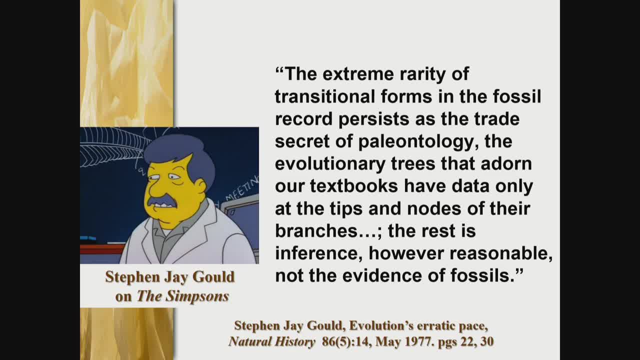 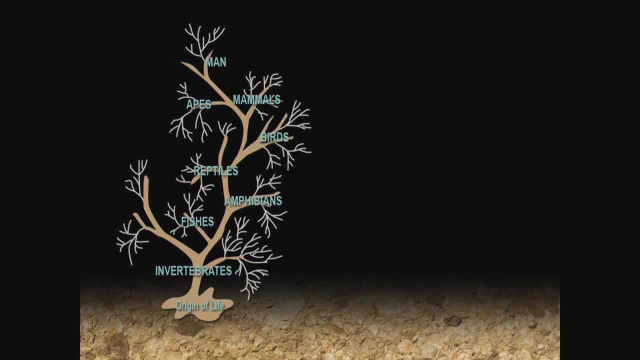 however reasonable, not the evidence of fossils. We simply cannot point to fossils to fill out Darwin's tree of life. He assumed that we would, that the groups of animals that are alive today would be connected together by fossil forms, But the fossils that we find in the fossil record are, by and large, 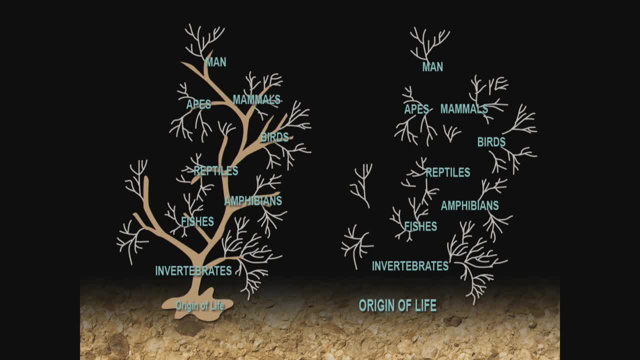 the same animals we find alive today, And some of them are just identical. You don't see the change. They're living fossils. They're the same animals we find alive today And again. when they first appear in the fossil record, they just pop out of nowhere, They just boom, suddenly appear in the 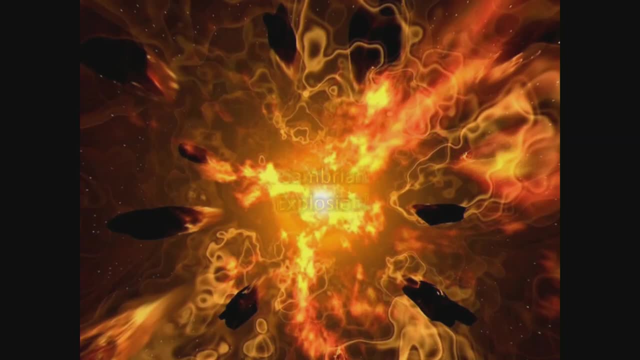 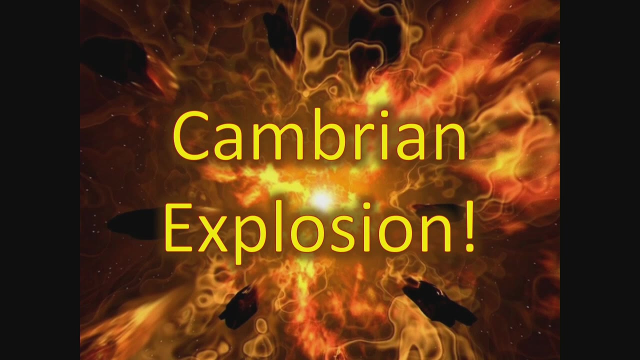 fossil record, And the best evidence of that is that they're not just living fossils. They're living fossils, And the best evidence of this, or illustration of this, is an evolutionary event that is called the Cambrian Explosion. This geologic or evolutionary event is called an. 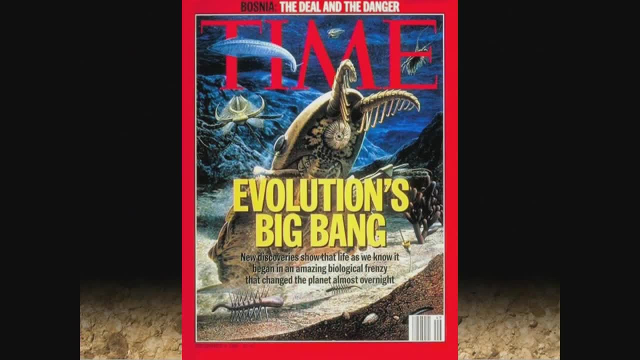 explosion because at one point in time life just suddenly boom appears on the scene. It's called evolution's big bang in this Time magazine article. The Cambrian Explosion is what they call the sudden appearance of life in that one geologic period. 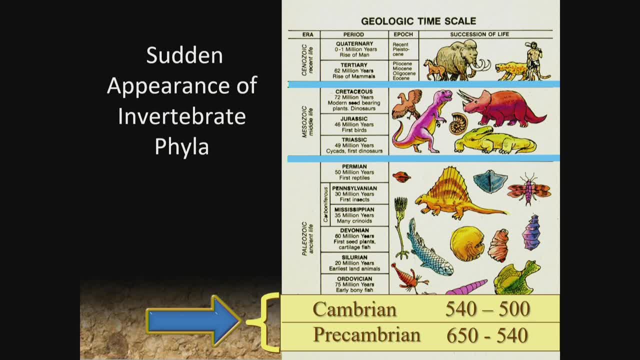 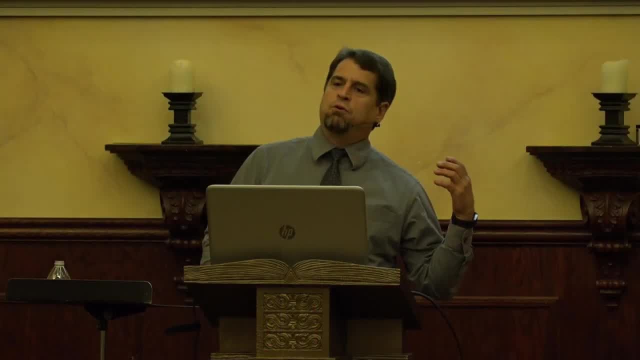 We call the Cambrian. Before the Cambrian there's just bacteria, bacteria and bacteria and bacteria. And actually the origin of life is getting pushed further and further and further back, because as they dig deeper into geologic strata and as they analyze the geologic rocks, they keep finding bacteria. At this point in time, the origin of life has been pushed all the way back to like 3.9 billion years. They believe the Earth is 4.6 billion years old and the origin of life is now pushed back all the way back to 3.9 billion years. And that's the origin of life. 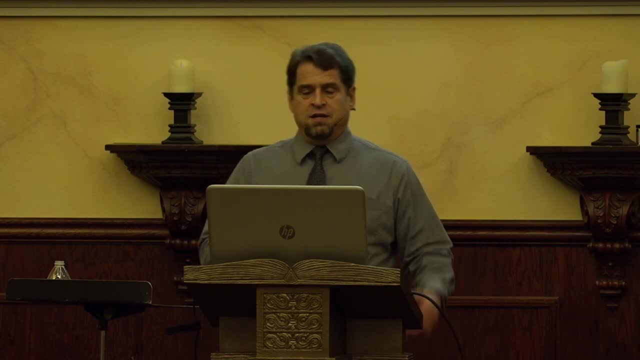 But at one point in time there's nothing but bacteria, bacteria and bacteria for billions of years. And then, suddenly, out of nowhere, boom during this Cambrian period. all of the major invertebrate phyla just suddenly appear, most of them, And they appear fully formed Out of. 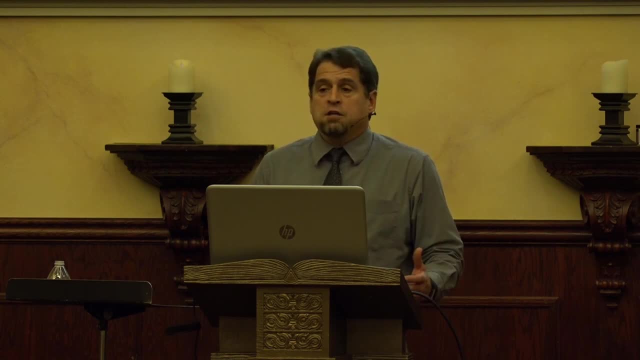 nowhere. these things just suddenly pop into existence. But that's the case for the vast majority of animals we find alive today- highly specialized animals, the flying animals, animals like bats and so on, And that's the origin of life. And that's the origin of life, And that's the 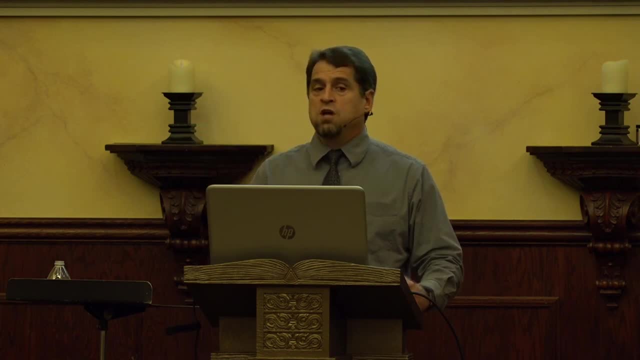 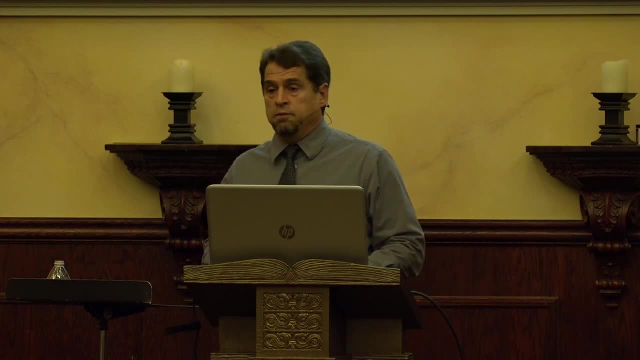 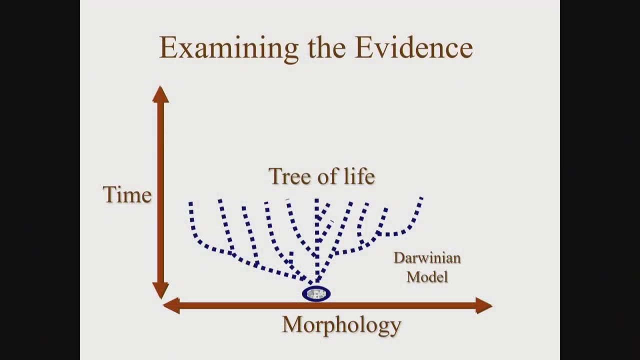 formed bat. These animals just appear in the fossil record out of nowhere. Darwin's tree of life as he drew, he drew a tree of life like this. That's what it's affectionately called by evolutionists. They call it the tree of life, the phylogenetic tree. But where did 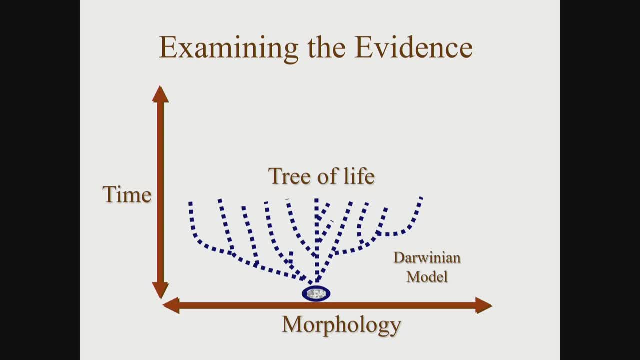 they get the term tree of life. That's from the Bible, right, That's how they use our biblical terms: the tree of life. But Darwin's tree of life, as he envisioned it, starting off with just that one ancestral cell, eventually evolving into multiple life forms on earth, is just not. 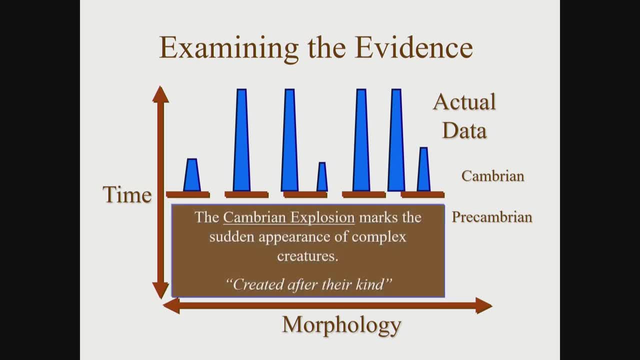 illustrated by way of the fossil record. What we see is a sudden and rapid, abrupt appearance of life on earth. Life appears out of nowhere. Most of the invertebrate phyla just suddenly pop into existence, and many of them are identical to ones we still find alive today. So let me summarize. 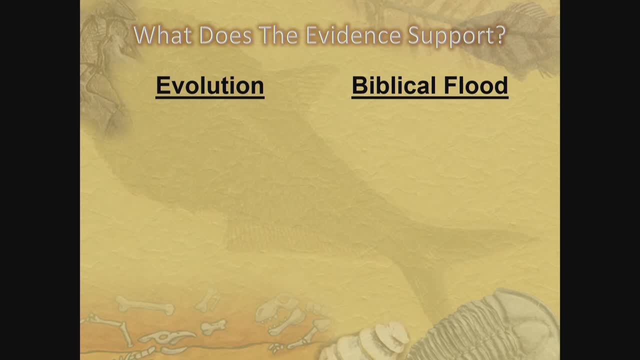 what the evidence really shows, whether geology and the fossils actually prove evolution or whether it's more strongly supportive of a biblical flood. Let's look at the evolution side. We see life appearing suddenly in the Cambrian explosion. That argues strongly against what Darwin's 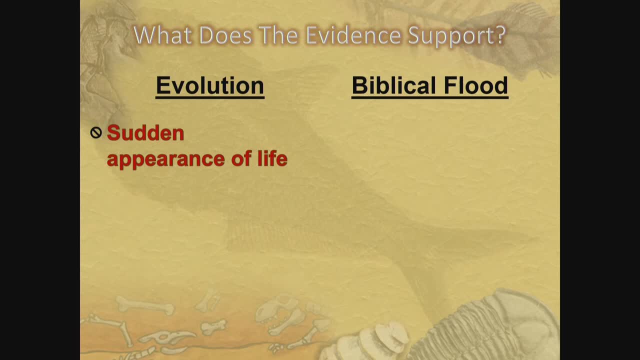 asserted. a slow and gradual process like natural selection doesn't give rise to multiple phylas. suddenly, the way they appear in the fossil record, We see an overwhelming absence of transitional forms. Distinct groups of animals are found both living and in fossil forms. This is not at all. 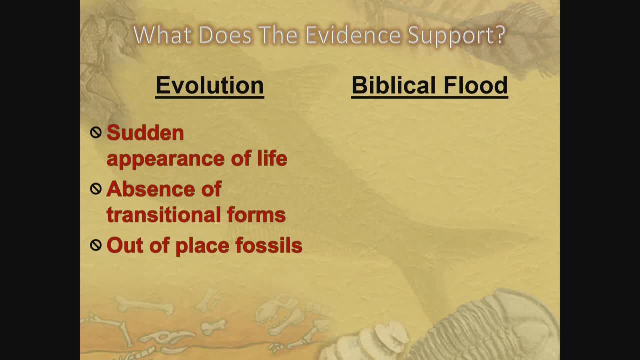 what is expected if Darwin's theory is true. We see a great number of out-of-place fossils. many animals that are not found in upper layers of the fossil record and were assumed to be extinct for millions of years have been found living, forcing them to completely revise their views on 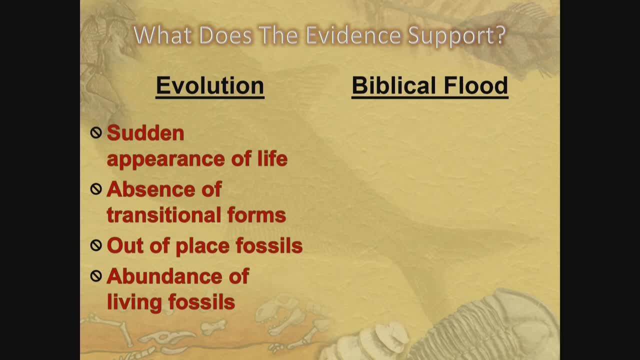 these organisms And we see a tremendous abundance of living fossils. But what about the biblical flood? We see one of the laws of stratigraphy strongly supporting the biblical flood: the law of lateral continuity. These layers of fossiliferous rock extend forever, Blanket entire regions of 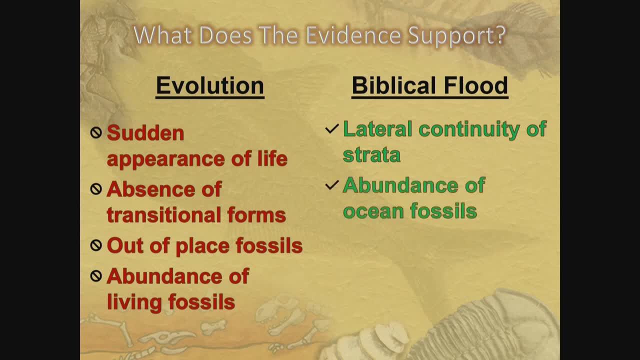 continents can be traced for hundreds and in some cases thousands of miles. We see an overwhelming abundance of ocean fossils in the fossil record We see fossils that are highly preserved, showing almost no sign of decomposition. Soft tissues can be found in many, many. We also see these mass mortality beds, these fossil 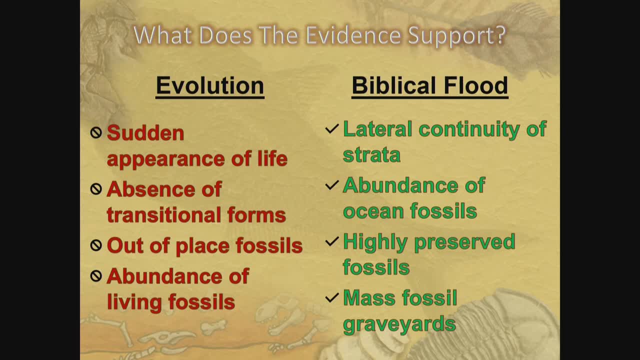 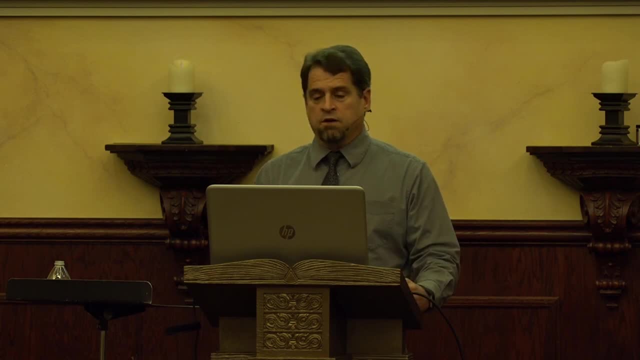 graveyards that are a common part of the fossil record. If you look at the overall characteristic of the fossil record of geology and the fossils, it is much more supportive of the biblical catastrophic flood, because that's what the fossil record is. I mean, it is a record but it's not a 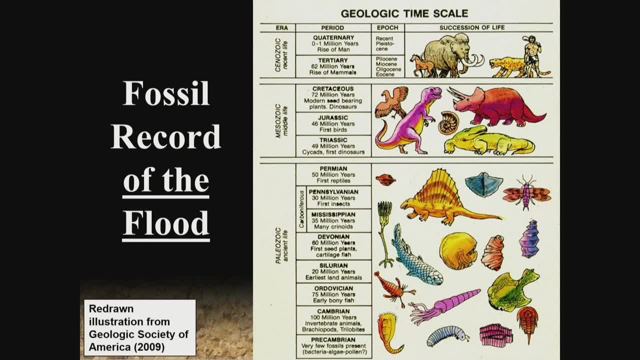 record of life on earth. It's a record of life on earth. It's a record of life on earth. It's a record of life on earth over hundreds of millions of years. It's a record of a devastating judgment brought about by God. And the reason why it's so important, the reason why upholding these historical events, 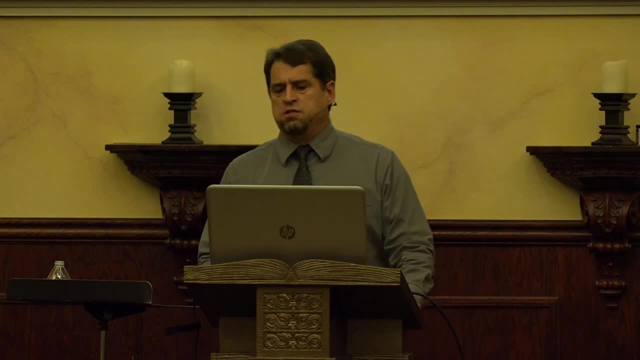 in the Bible is so important. I think it was summarized well by Jesus. He actually said two different things. He said: if you believe Moses, you will believe me before he wrote about me. But since you do not believe what Moses wrote, how are you going to believe what I say? 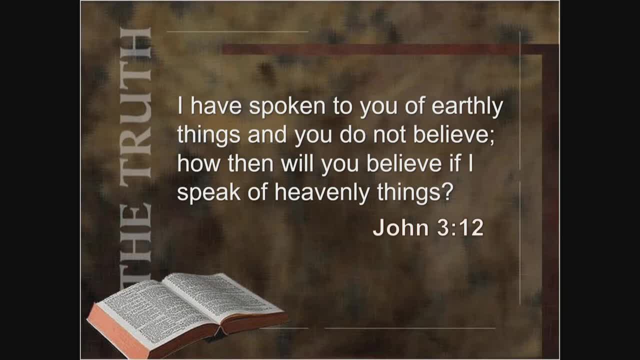 He also said: I've spoken of earthly things that you do not believe. How, then, will you believe I speak of heavenly things? Point made in both was that if we can't trust what the Bible says on historical matters, events like the biblical flood, events like the Garden of Eden, how can we trust? 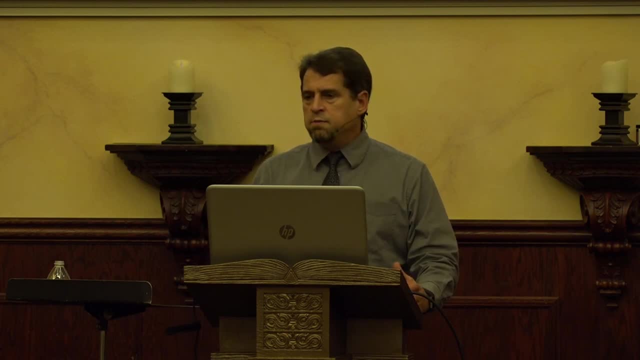 what it says on spiritual matters like salvation. The Old Testament and the New Testament are part of the same book. If we let events in the Old Testament fall to the fault of fables or myths, if we let these be challenged by scientific claims and those challenges go unanswered, it will 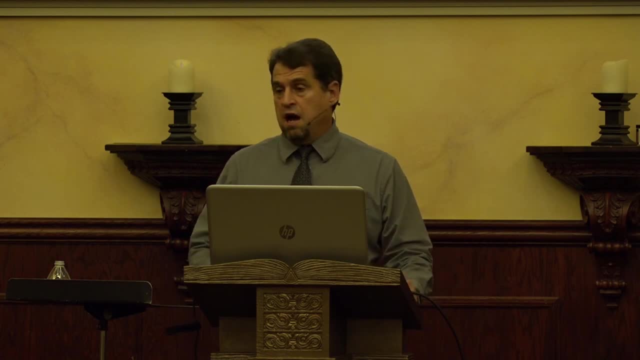 cause a person to lose their faith. I believe that the theory of evolution is one of the main impediments today that keeps a person from coming to the faith, And it is one of the main causes for the loss of faith that we see in, particularly amongst young people, Young people that grow up. 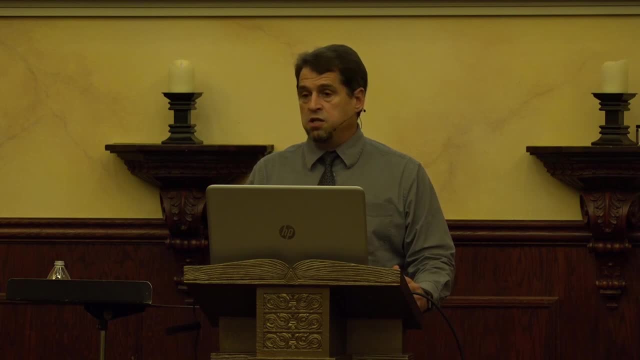 in the church get up higher into their education. By the time they're out of high school, they're already starting to doubt the Bible because of historical events like Noah's flood, And by the time they get out of college, many of them have lost their faith, And it's because we're 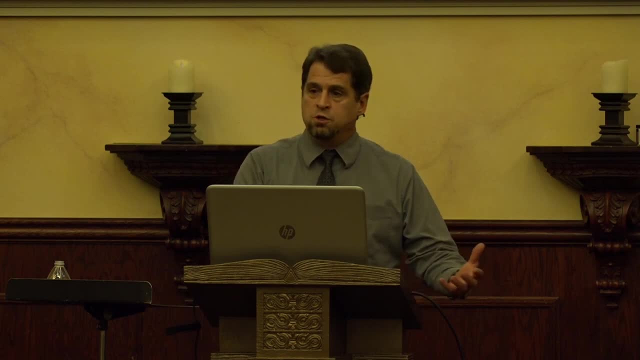 not giving them the answers. We need to give them the answers before the questions come up in their mind. We don't let the doubts start, because those festering doubts will grow, And I believe it's a terrible thing that leads both to loss of faith and loss of faith, And I believe it's a terrible thing that leads both to. 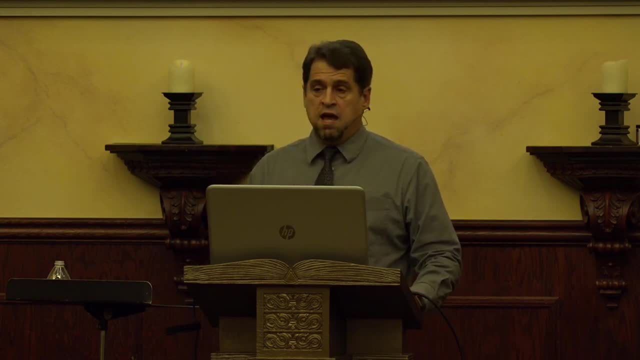 loss of faith and loss of faith, And I believe it's a terrible thing that leads both to loss of faith and loss of faith in kids that have grown up in the church, And it's an impediment that can keep someone from coming to the faith. That's why apologetics are so important. I don't study these. 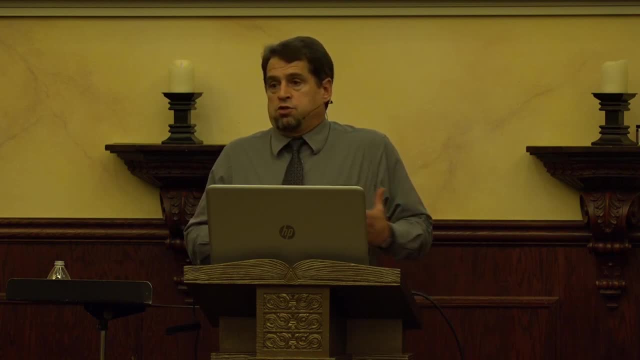 things to bolster my own faith or to strengthen my own faith. I study them so that I can give answers to others, others who are struggling To be a witness. today, again, you need to be prepared to answer some questions, you know, because there are a lot of people think evolution 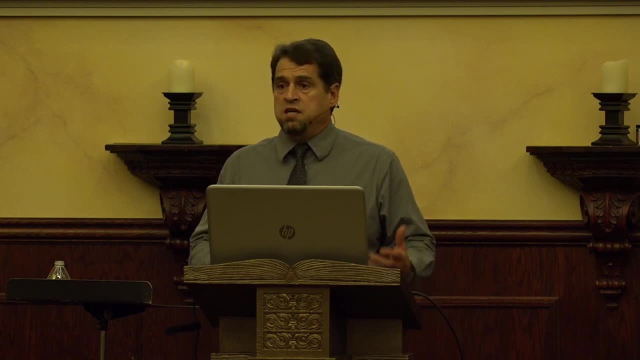 has been proven, but often they just have not seen the evidence, And so I think it's important to have not seen what the evidence really is and where the big holes are in that evidence, like transitional forms or the origin of life, Or you know, some people think they've proven that we've 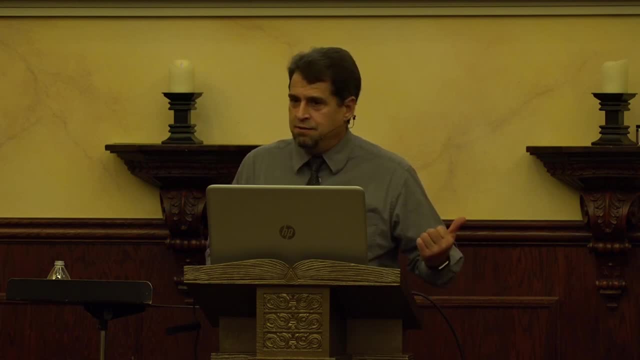 evolved from apes. Have they looked into those ape men? Have they looked into those, the missing links between apes and men. Those are pretty big too. But I think one of the most harmful things about them reinterpreting the fossil record, about them reinterpreting these layers of sedimentary. 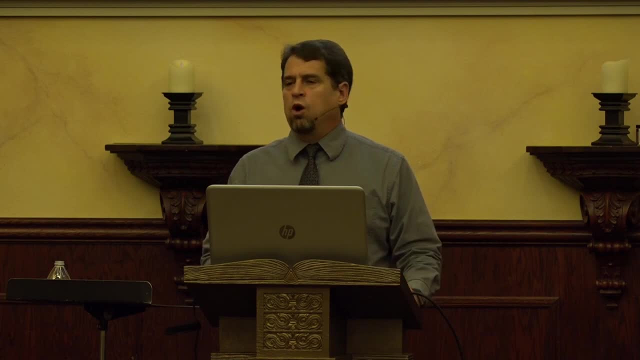 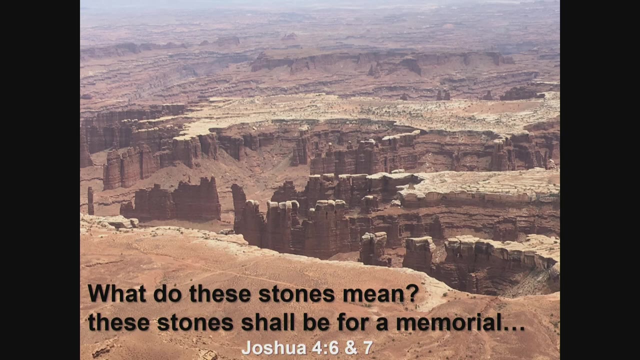 rocks is because of what these layers of rocks were always meant to be. I mean, we know why God sent the global flood. He sent it because of the wickedness of the human race on earth in those days, And he decided to wipe people from the face of the earth and the birds and the 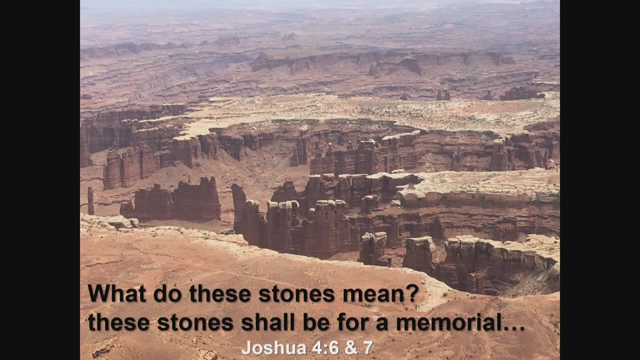 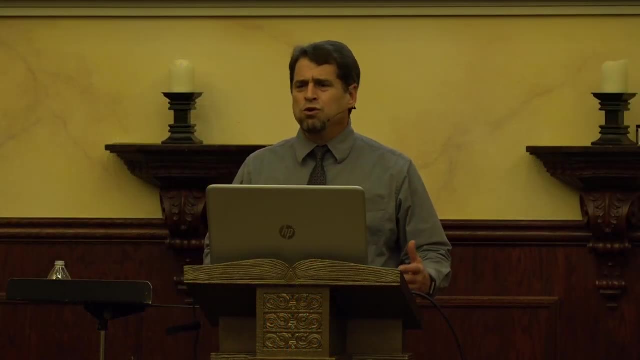 creatures. But if his purpose was just to wipe out mankind, he could have done it much more cleanly, you know, could have released a virus And just killed the people And not kill all the plants and animals, not destroy the hydrological system, not destroy the earth as it was originally created. The whole earth was. destroyed The system, the water cycle that existed before the flood is gone. We don't really even know how the earth operated before, but it was devastatingly altered. I guarantee you that He could have done it much more cleanly, But I believe he did it through a global flood. 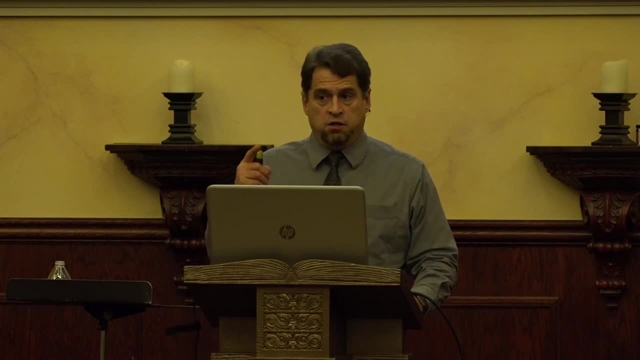 because he wanted to leave a monument a reminder to us of just how much he hates sin. And he wanted to leave a monument a reminder to us of just how much he hates sin, That he did it by way of a flood, to leave a monumental reminder. So when we looked at those, 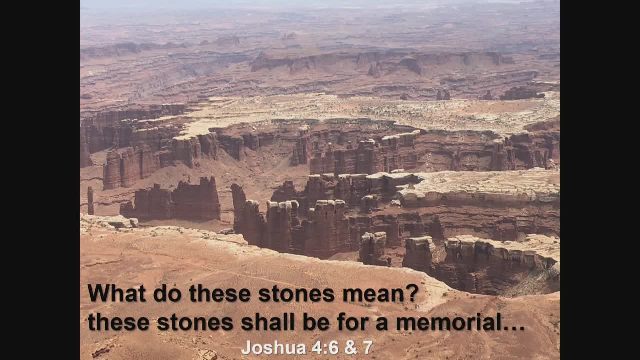 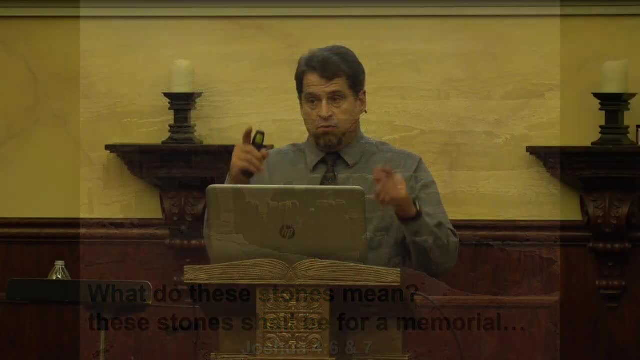 layers of rocks. when we look at those fossils, when you go to places like Grand Canyon or out to the Columbia River Gorge and you see those vast layers of rocks, you're reminded how much God hates sin By them. reinterpreting those layers of rocks, they've taken away this important 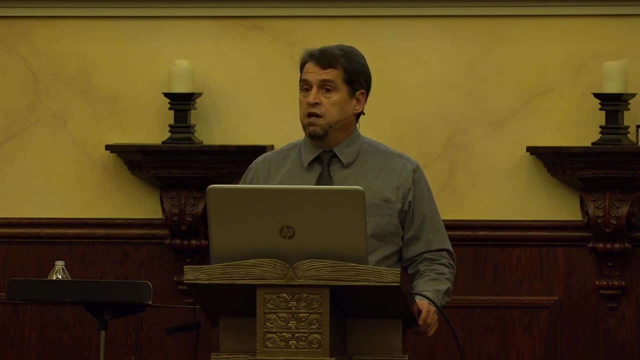 reminder And we shouldn't forget, because God's hatred of sin has never changed. The modern church tends to avoid the verses that talk about his hatred of sin and his hatred of sinners And they emphasize the passages that talk about his love. but his hatred of sin has never changed The God. 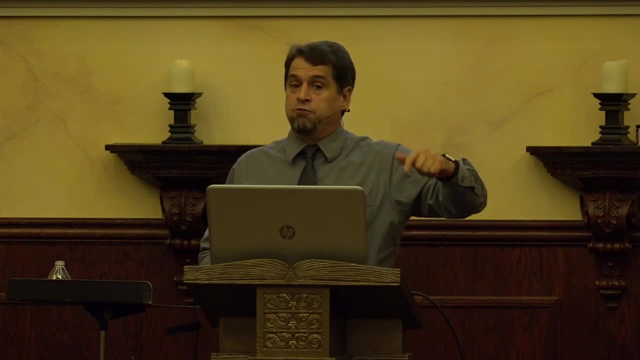 that destroyed the world by flood. we will stand in front of one day and have to give a reckoning to about why we lived the way we live. And I got to say, if you want to debate the point, whether God's hatred of sin has changed or not, I don't think so. I don't think so. I don't think so, I don't. 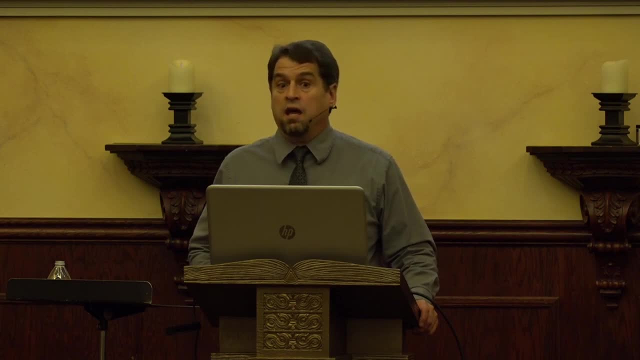 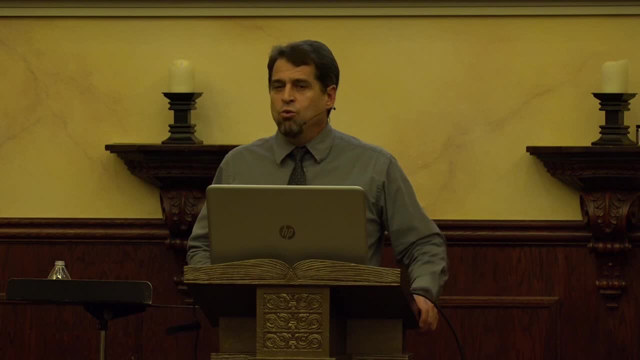 for us And we know that. We know he sent his son to die for us. And then you continue to live in sin. I got to tell you his hatred of sin is probably much greater today than it was before the flood. We shouldn't forget the God that destroyed the world by flood. We will stand in. 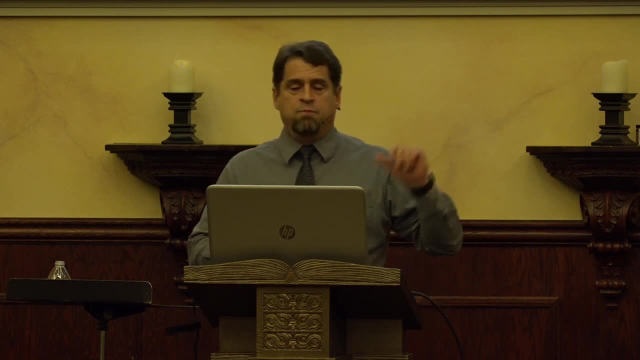 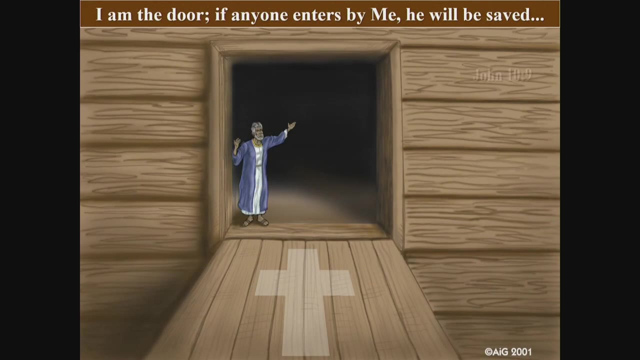 front of one day and have to give an account for him. But just like he provided us with the, a plan for Noah to survive the judgment of his day, remember that he's provided a plan for us too. All we have to do is ask for forgiveness. The penalties for our sins have been paid. 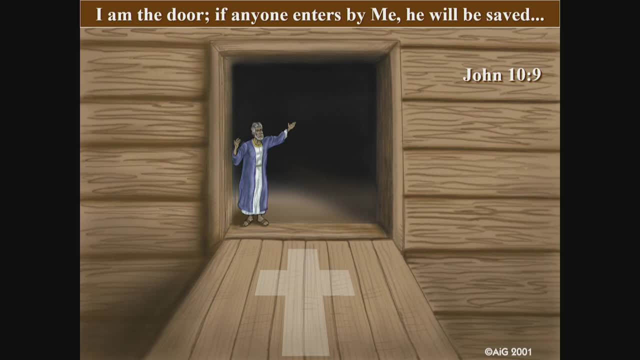 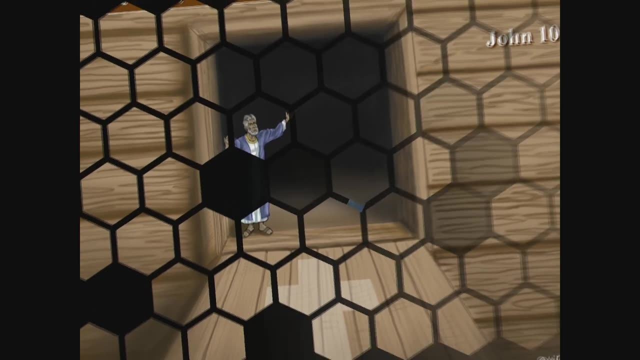 All you have to do is ask for forgiveness and repent, turn from those sins, and forgiveness is there and waiting for us. That's all we have to do. Let me close in a word of prayer, Father God. thank you so much, Lord, for your word and for the tremendous insight that we have. 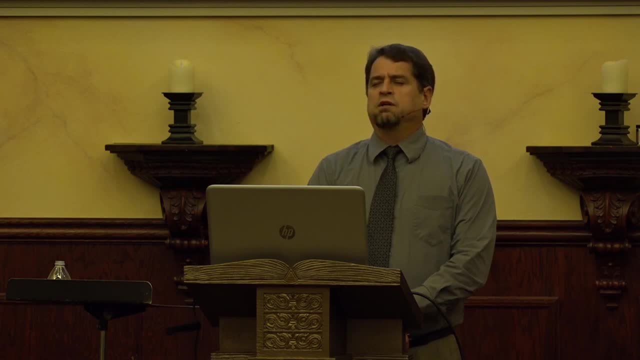 gained from it, Father God, that we know that these events were real and we understand the world that we live on better than most. Father God, Father God, give us wisdom. Father God, we want to be a servant for you, Father, but it's difficult understanding the science. It's.